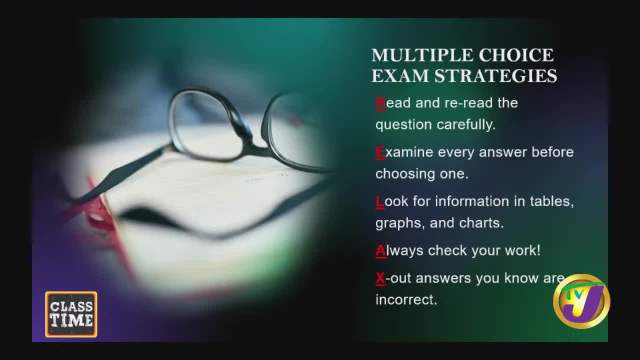 choosing one. So you're going to go over your questions. Examine the questions carefully. The distractors are there for a reason: in tables, graphs and charts. always check your work. I know sometimes you're speeding through multiple choice. I know this. I got this. I don't check over check. 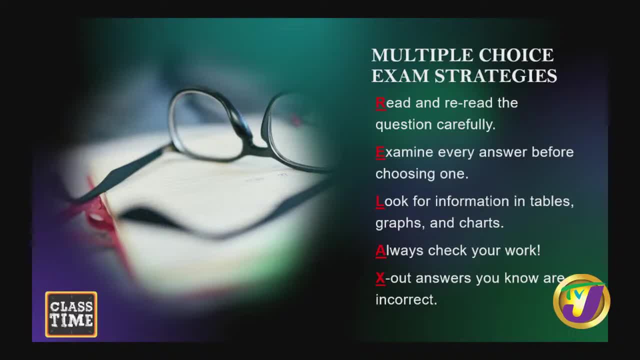 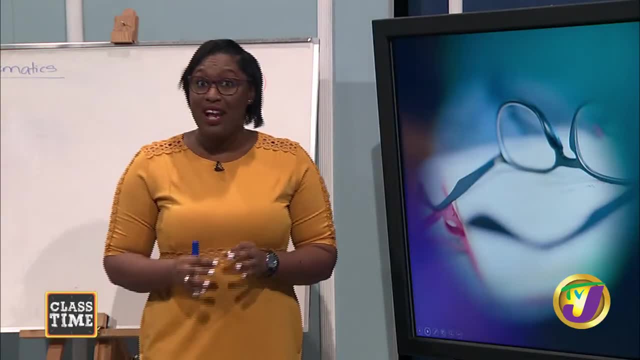 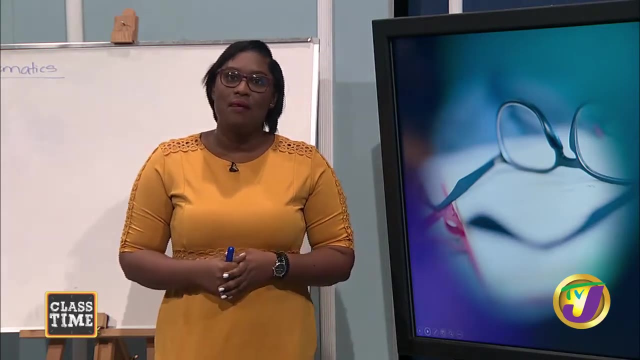 over your work. please do that. exalt all answers you know are incorrect. and again, there are lots of answers on your multiple choice paper that are very, very similar, so go through and eliminate them right. so again, when you're doing your exam, relax what you got me, Brittany, what you mean, eliminate, eliminate. 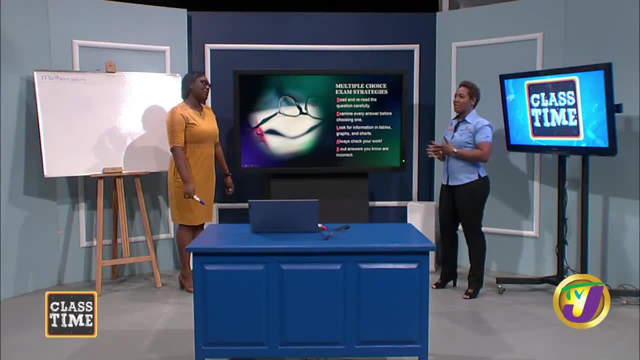 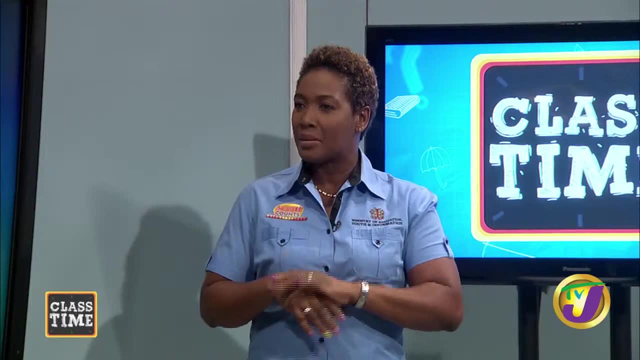 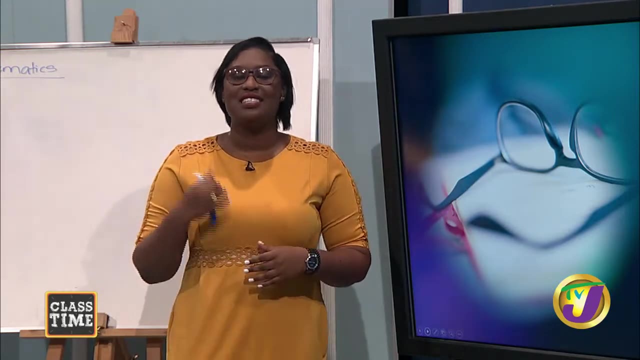 mark it all to get rid of it. that's what you mean: eliminate. you had said something, though you said that some of the some of the destruction, the distractors, are very similar. yes, what you mean. so with the multiple choice paper, it's so designed that several answers are going to look very they're. 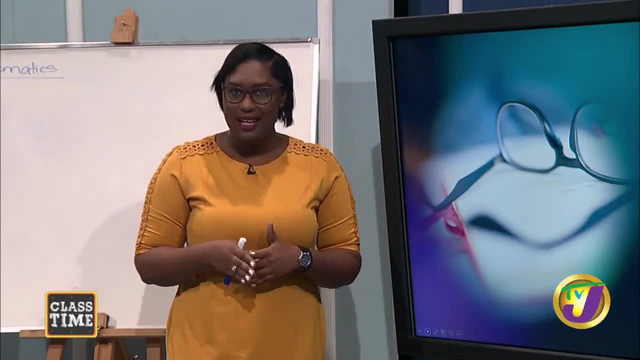 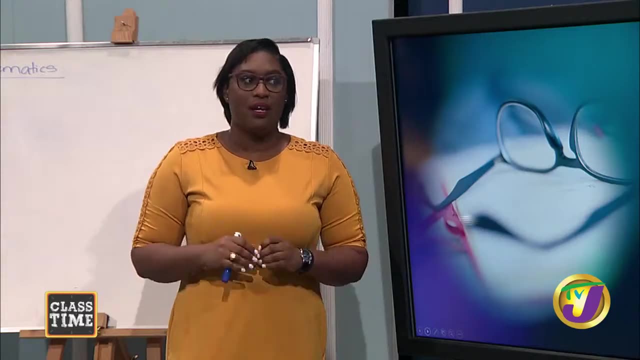 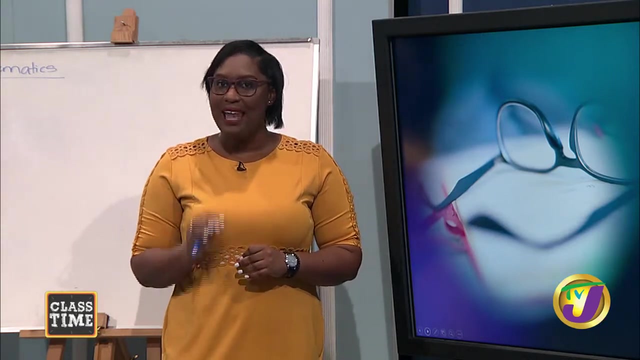 very good. they're going to be very close. so there's only really one correct answer most times on these papers anyway, because you do have multiple select exam, multiple choice. people's chemistry does that, yeah, but for this one in math we're looking for one correct answer, but they're going to be several answers that. 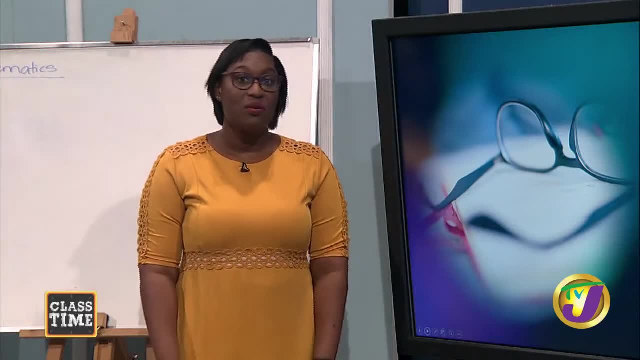 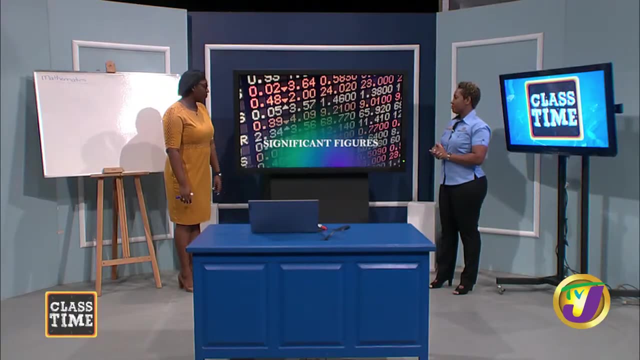 are very similar, all right. so when I say eliminate, get rid of it, throw it out, right, so look for the correct one. so now we're going to go into some interesting stuff we're going to know, getting to know the answer. and then we're going to go into some interesting stuff. we're going to know. 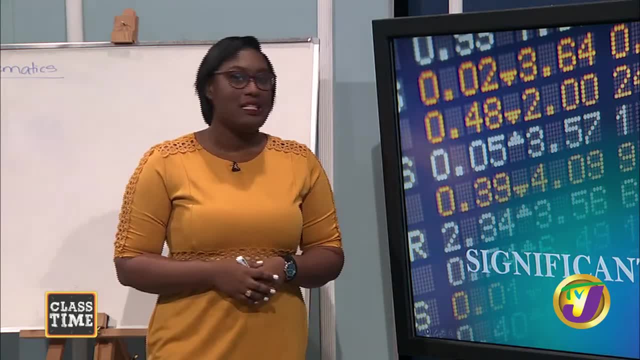 getting to know the answer. and then we're going to know the answer. and then we're going to know the meat of the matter. we're getting into the math of it so significant. the meat of the matter. we're getting into the math of it so significant. 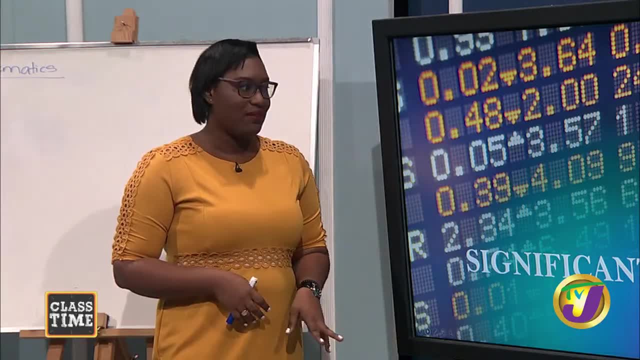 the meat of the matter. we're getting into the math of it. so, significant figures, right. why them significant figures, right? why them significant figures, right? why them significant? what are they? hey, they're figures and they, what are they? hey, they're figures and they, what are they? hey, they're figures and they clearly have some value. we need to. 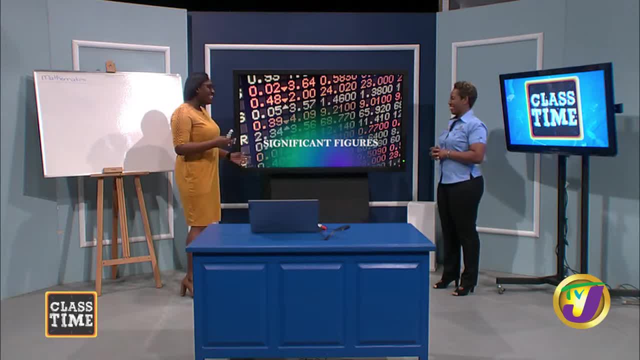 clearly have some value. we need to clearly have some value. we need to do something to turn to Tamika today. yeah, do something to turn to Tamika today. yeah, do something to turn to Tamika today. yeah, my name significance all right, so let's my name significance all right, so let's. 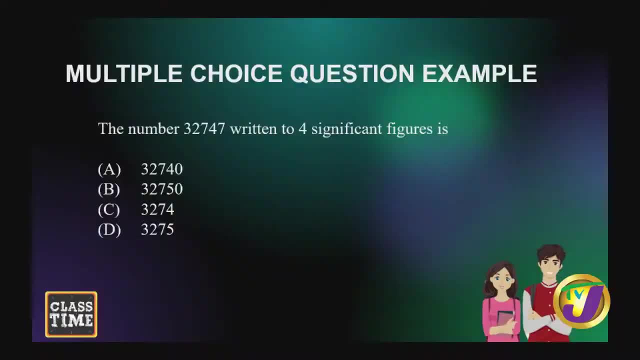 my name significance. all right, so let's get into it, guys. all right. so here we get into it, guys. all right. so here we get into it, guys, all right. so here we have a question. the number three thirty have a question. the number three thirty have a question. the number three: thirty thousand thirty two thousand seven. 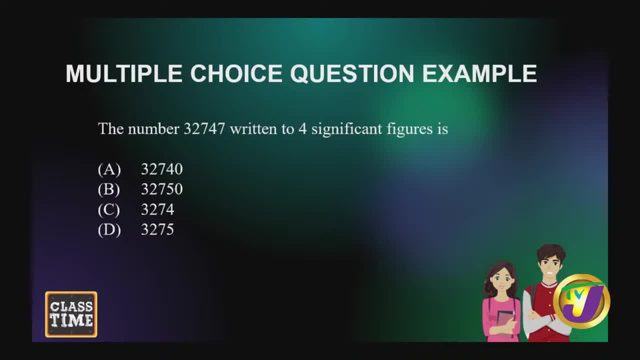 thousand thirty two thousand seven thousand thirty two thousand seven hundred forty seven, written to four hundred forty seven, written to four hundred forty seven, written to four significant figures. so let me, let me let significant figures. so let me let me let significant figures. so let me, let me let me do it. all. right, it's so, I'm gonna. 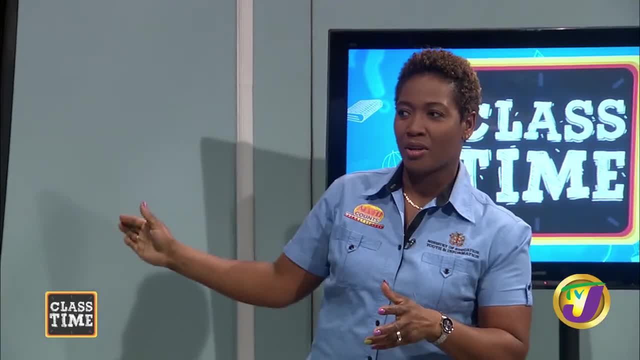 me do it all right, it's so. I'm gonna me do it all right, it's so. I'm gonna write three thousand two hundred seventy. write three thousand two hundred seventy. write three thousand two hundred seventy four because I just been drop off at four. because I just been drop off at. 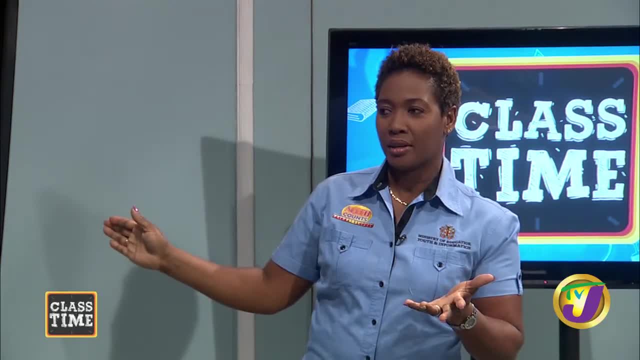 four, because I just been drop off at seven. what why that can't work well seven? what why that can't work well seven? what why that can't work well? let's have our friends, so on the screen. let's have our friends, so on the screen. let's have our friends, so on the screen. right, we're still friends. we have Jenny. 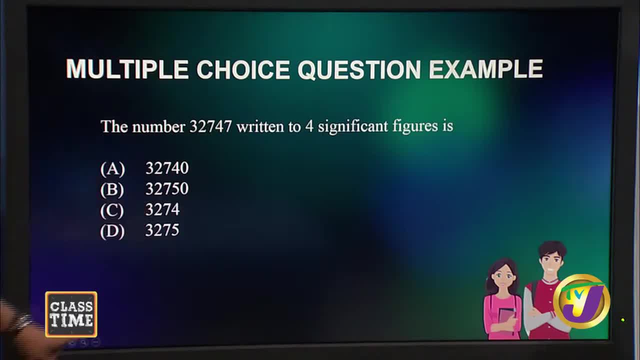 right, we're still friends. we have Jenny. right, we're still friends. we have Jenny and Jack. Jenny and Jack is here to help and Jack, Jenny and Jack is here to help and Jack, Jenny and Jack is here to help us today. okay, so you know when we're. 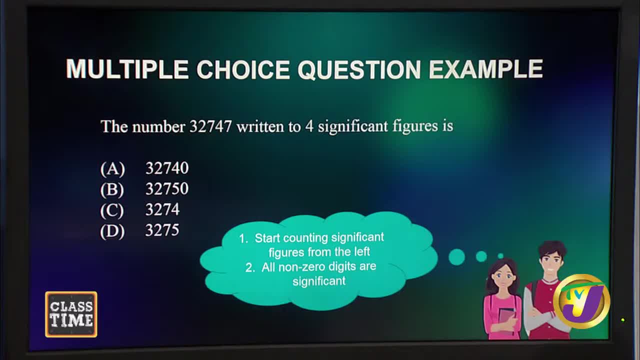 us today. okay, so you know when we're us today. okay, so you know when we're he's there helping us out. so when we he's there helping us out, so when we he's there helping us out, so when we talk about significant figures, right, we? 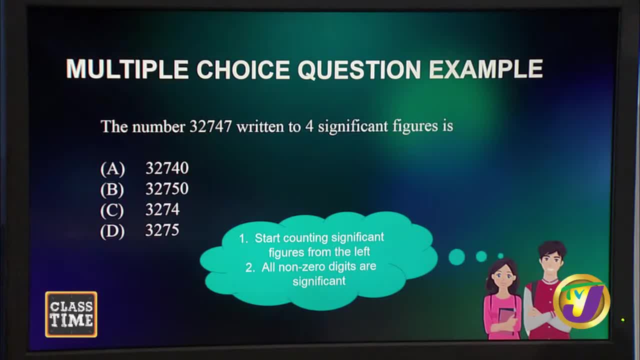 talk about significant figures, right, we talk about significant figures, right, we have to start identifying our have to start identifying our have to start identifying our significant figures from the left of the significant figures, from the left of the significant figures from the left of the number. so here we have 32 thousand. 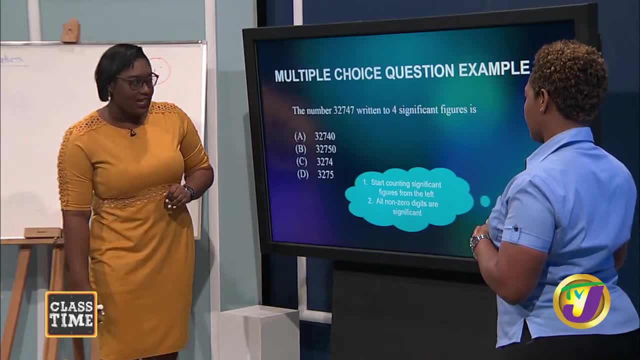 number. so here we have 32 thousand number. so here we have 32 thousand seven hundred forty seven and Jenny and seven hundred forty seven and Jenny and seven hundred forty seven and Jenny and Jack said that was need to start. Jack said that was need to start. 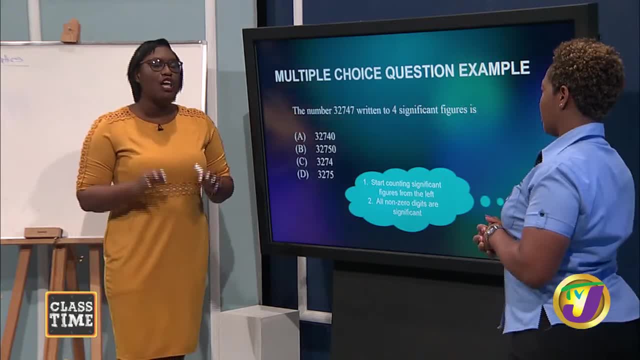 Jack said that was need to start counting significant figures and in this, counting significant figures, and in this counting significant figures, and in this case, all non zero digits are case. all non zero digits are case, all non zero digits are significant. so let's go. so here my three. 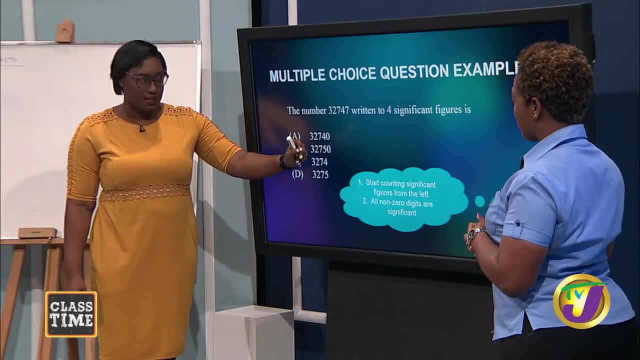 significant, so let's go. so here. my three significant, so let's go, so here. my three is significant, my two is significant, my is significant. my two is significant, my is significant, my two is significant, my seven significant, my four significant. I seven significant, my four significant I. 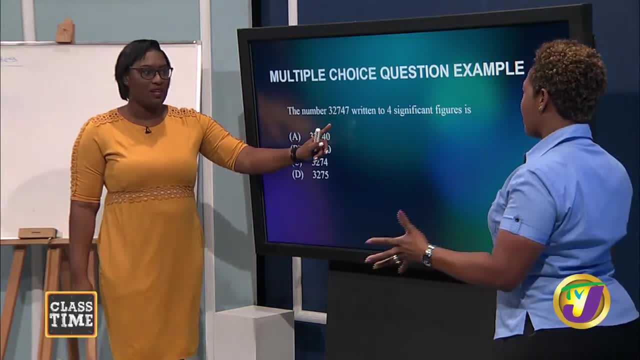 seven significant, my four significant. I know what you're going to fire for four. know what you're going to fire for four. know what you're going to fire for four. all right lady. what is wrong with this? all right lady? what is wrong with this? all right lady? what is wrong with this lady? so no, let's look at the seven right. 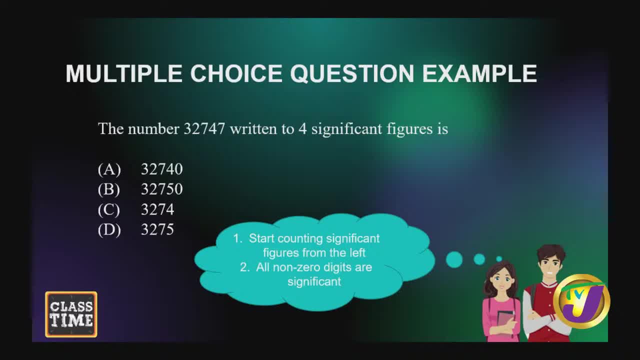 lady. so no, let's look at the seven, right lady. so no, let's look at the seven, right. what's the value? seven is seven. what's what's the value? seven is seven. what's what's the value? seven is seven. what's the value of seven? well, it's seven ones. 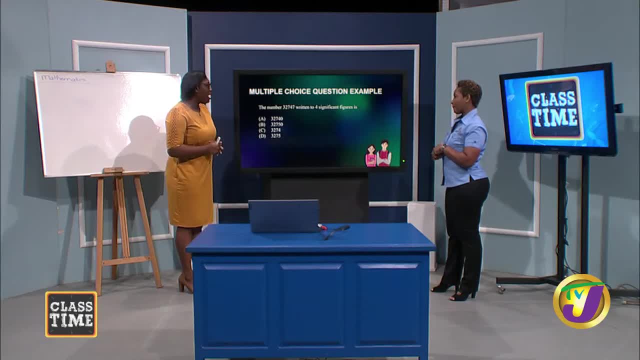 the value of seven. well, it's seven ones. the value of seven. well, it's seven ones in this number. all right, so it's seven in this number. all right, so it's seven in this number. all right, so it's seven ones in this number. and another way we. 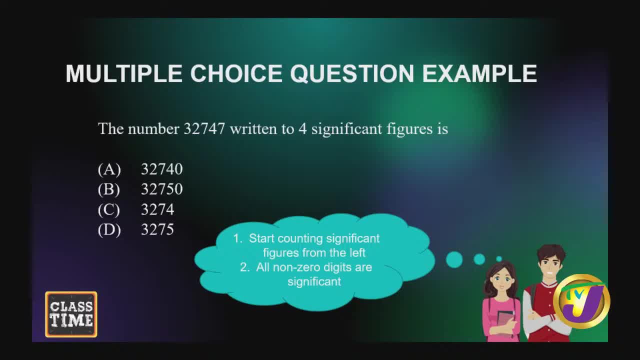 ones in this number and another way we ones in this number and another way we can look at it is how close is thirty can look at. it is how close is thirty can look at it is how close is thirty. two thousand seven hundred forty seven to two thousand seven hundred forty seven to. 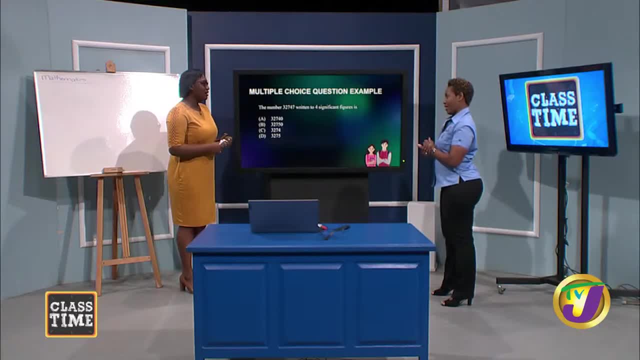 two thousand seven hundred forty seven to the nearest, the nearest, the nearest: 10. oh well, is it closer to 40 or is it 10? oh well, is it closer to 40 or is it 10? oh well, is it closer to 40 or is it closer to 50? well, if you give me 47. 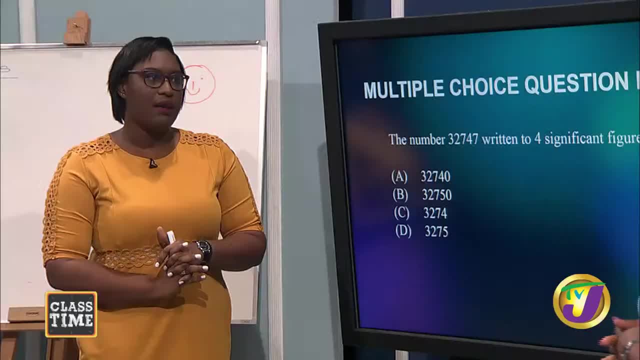 closer to 50. well, if you give me 47 closer to 50. well, if you give me 47 dollars, it i almost have fifty dollars dollars. it i almost have fifty dollars dollars, it i almost have fifty dollars. so it's close to 50.. okay, so it's close to 50.. okay, so it's close to 50.. okay, so, if it is that we're now going to, so, if it is that we're now going to, so, if it is that we're now going to write this to: 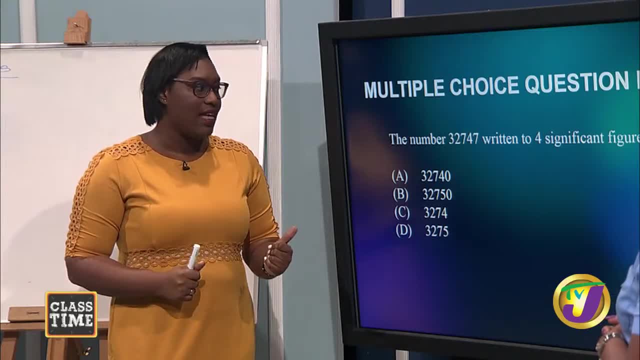 write this, to write this to four significant figures right and my four significant figures right and my four significant figures right, and my zero is not going to be significant. zero is not going to be significant. zero is not going to be significant, then it simply means that my solution in 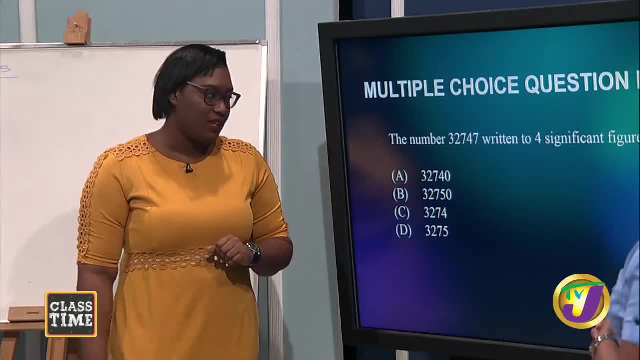 then it simply means that my solution in then it simply means that my solution in this case is going to be: this case is going to be: this case is going to be: thirty two thousand seven hundred fifty thirty two thousand seven hundred fifty thirty two thousand seven hundred fifty no. 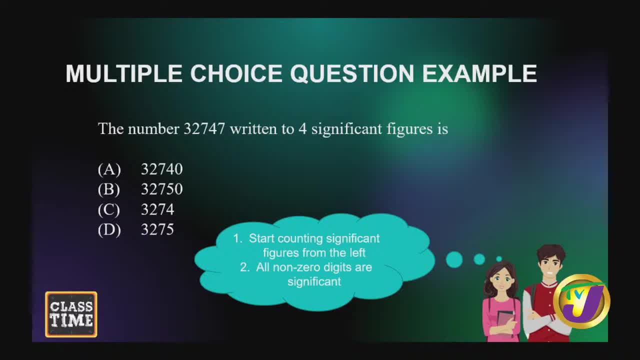 no, no, we're seeing it because my zero here is. we're seeing it because my zero here is. we're seeing it because my zero here is not going to be significant and when i not going to be significant and when i not going to be significant, and when i count, it's one, two, three, four. 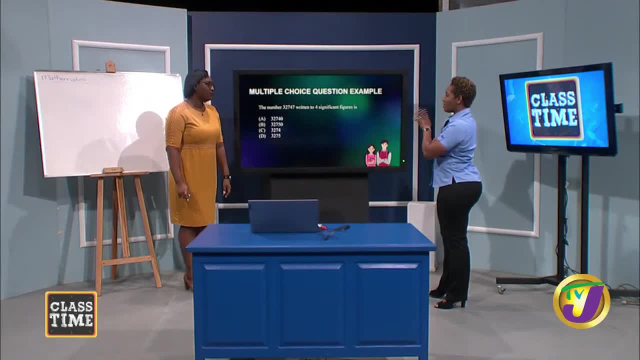 count it's one, two, three, four. count: it's one, two, three, four. significant figures, significant figures, significant figures. oh, if i drop off the seven, i would no. oh, if i drop off the seven, i would no. oh, if i drop off the seven, i would no longer have thirty two thousand. 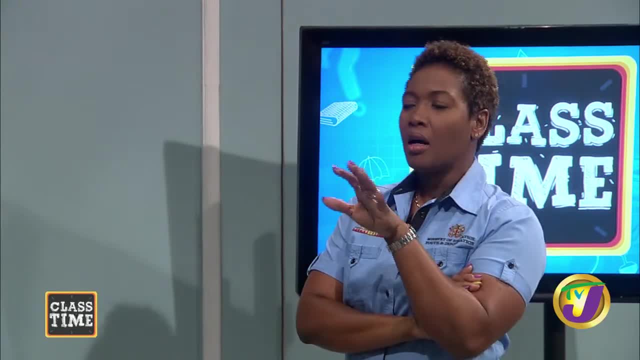 longer have thirty two thousand, longer have thirty two thousand, i would only have three thousand, so i, i would only have three thousand, so i, i would only have three thousand, so i would change the number all together, would change the number all together, would change the number all together. oh so, when you're looking at significant 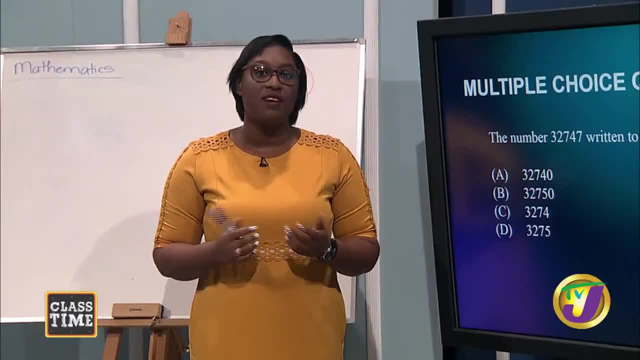 oh so when you're looking at significant? oh so, when you're looking at significant figures, you have to keep the integrity figures. you have to keep the integrity figures. you have to keep the integrity of the original number, of the original number, of the original number. yes, so the value has to remain the same. 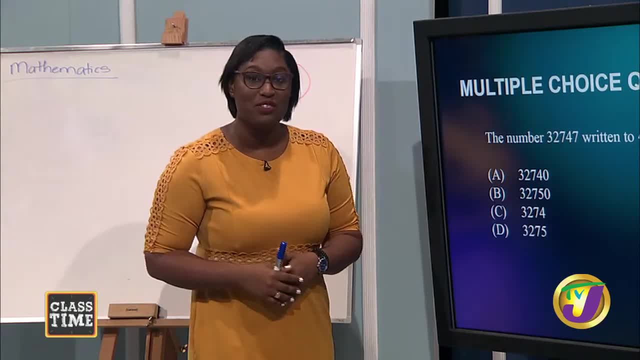 yes, so the value has to remain the same. yes, so the value has to remain the same. gotcha hence. why gotcha hence, why gotcha? hence why we now have 32 750, we now have 32 750, we now have 32 750. but wait, maybe, maybe i'm not right. 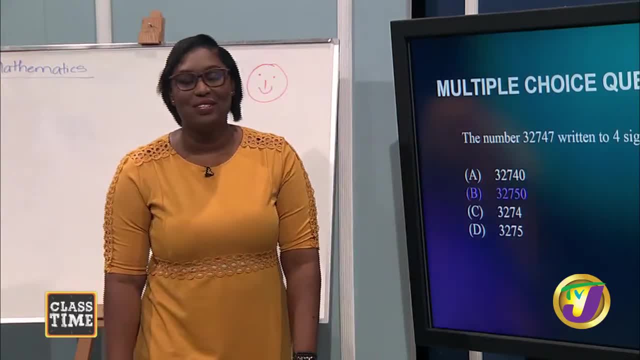 but wait, maybe maybe i'm not right. but wait, maybe maybe i'm not right, i'm correct. so, as you can see, guys, it is i'm correct. so, as you can see, guys, it is, i'm correct. so, as you can see, guys, it is 32 750.. look a joke, you know? look a. 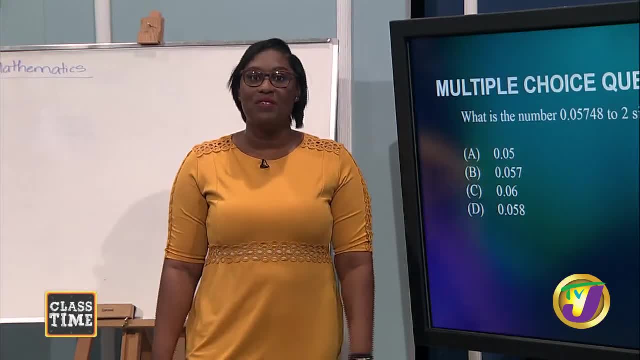 32 750.. look a joke, you know. look a 32 750.. look a joke, you know. look a joke in the early morning. joke in the early morning, joke in the early morning. all right, so here we have another one. all right, so here we have another one. 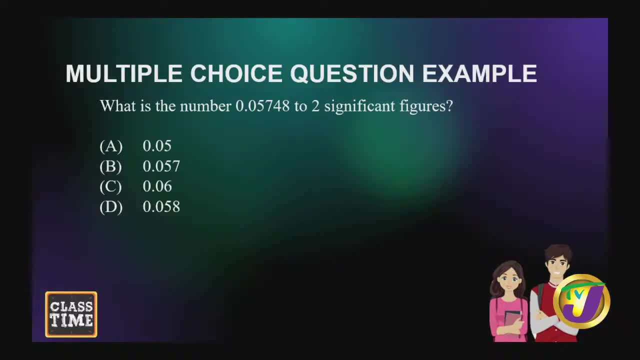 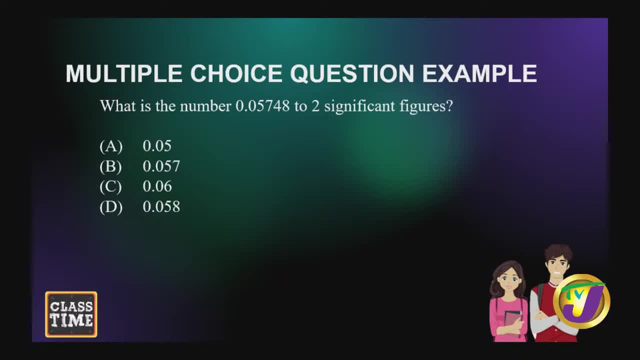 number: five thousand seven hundred. number five thousand seven hundred forty eight, that's what. ten thousandth forty eight, that's what. ten thousandth forty eight, that's what ten thousandth. is it ten, one, two, three, four? yes it. is it ten one, two, three, four? yes it. 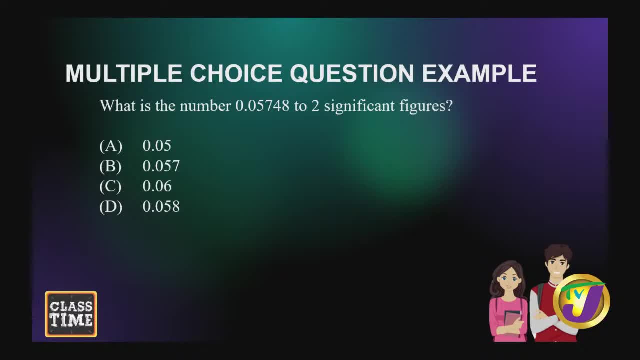 is it ten, one, two, three, four? yes, it looks like ten thousandth. that's the looks like ten thousandth. that's the looks like ten thousandth. that's the place. or you can say zero point, zero place, or you can say zero point, zero place, or you can say zero point, zero. five, seven, four, eight, just to let you. 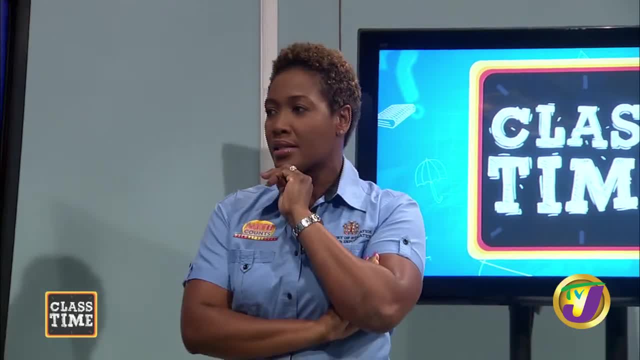 five, seven, four, eight, just to let you: five, seven, four, eight, just to let you know the digits that we're looking at, know the digits that we're looking at, know the digits that we're looking at, to two significant figures, to two significant figures, to two significant figures. well, you know what i would do already. well, you know what i would do already. well, you know what i would do already. but let's, let's look at it the way it. but let's, let's look at it the way it, but let's, let's look at it the way it should be done. 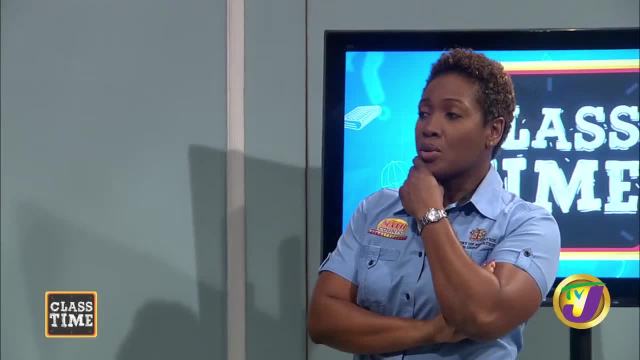 should be done should be done. okay, all right, so we have this number. you okay, all right, so we have this number. you okay, all right, so we have this number. you want to talk about. you said we count. want to talk about you said we count. want to talk about you said we count from the left. 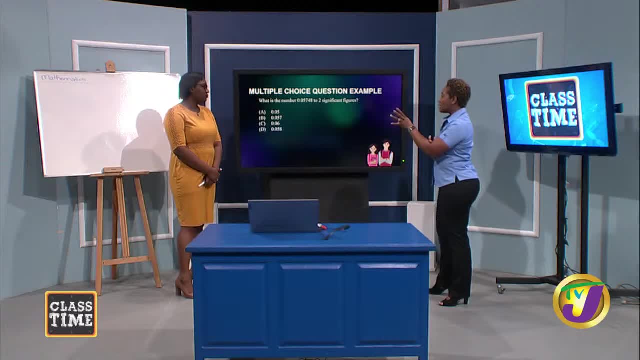 from the left, from the left, and it's any non-zero from the left, so, and it's any non-zero from the left, so, and it's any non-zero from the left. so, those two zeros, those two zeros, those two zeros, they're not significant because they're. 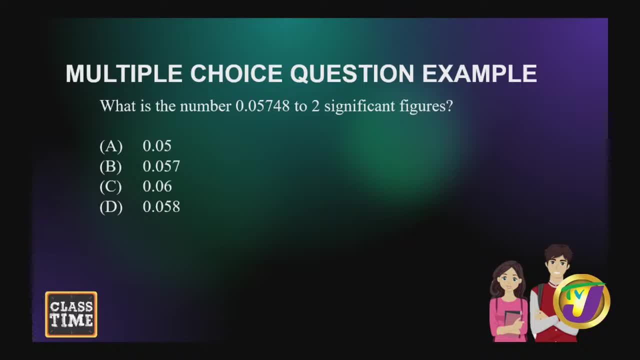 they're not significant because they're. they're not significant because they're ten, oh, lord, ten hundredth ten, oh, lord, ten hundredth ten, oh, lord, ten hundredth is closer to, is closer to, is closer to. hmm, hmm, hmm, all right, so that wouldn't make it so it. 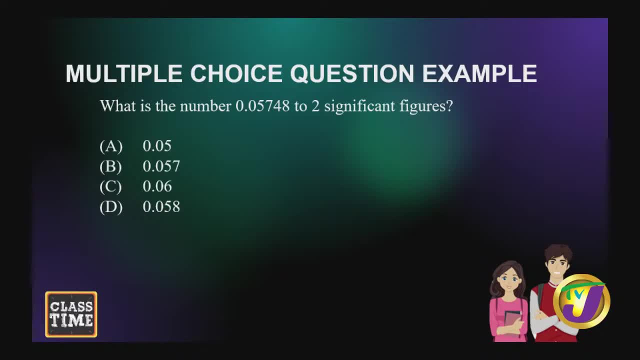 all right, so that wouldn't make it. so it all right, so that wouldn't make it. so it wouldn't be eight, wouldn't be eight, wouldn't be eight, it wouldn't make it to eight. because it wouldn't make it to eight, because it wouldn't make it to eight, because that's really not close to eight hundred. 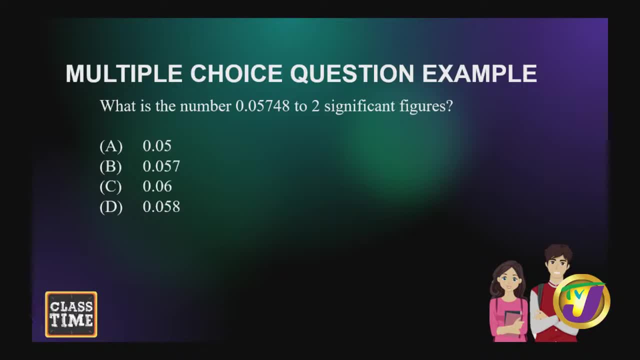 that's really not close to eight hundred. that's really not close to eight hundred. eight hundred ten thousandth, eight hundred ten thousandth, eight hundred ten thousandth. or is it yes, or is it yes, or is it yes? all right, so that would be zero point. 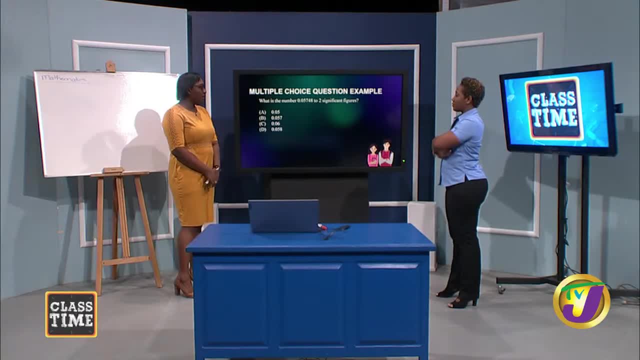 all right, so that would be zero point. all right, so that would be zero point. zero five seven. i'd go with that. zero five seven. i'd go with that. zero five seven. i'd go with that. okay, all right, hold on. so let's ask our. okay, all right, hold on. so let's ask our. okay, all right, hold on. so let's ask our friends jenny and jack. you know i told friends jenny and jack. you know i told friends jenny and jack. you know i told you guys. so jenny and jack is here to you guys, so jenny and jack is here to. 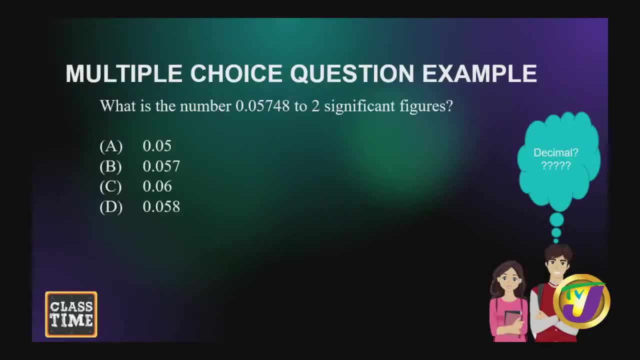 you guys. so jenny and jack is here to help us today, help us today, help us today. let's see what they have to say. so let's see what they have to say. so let's see what they have to say. so they're screaming about the decimals. 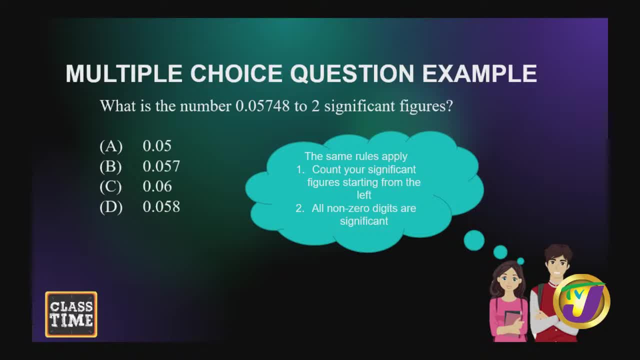 they're screaming about the decimals. they're screaming about the decimals right and right and right, and they're right on par. so our answer is: they're right on par. so our answer is: they're right on par. so our answer is b, which is 0.057. 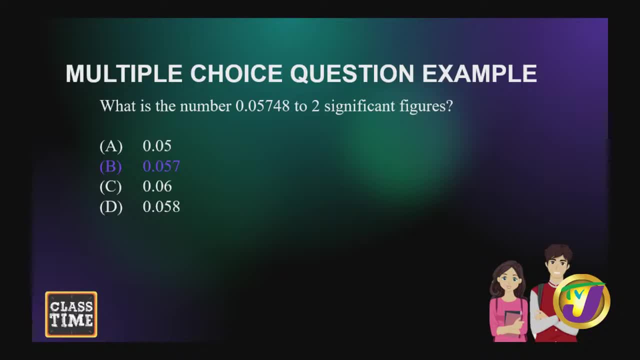 b, which is 0.057. b, which is 0.057. all right, we've seen that there. all right, we've seen that there. all right, we've seen that there. i hope you guys are following so far, and i hope you guys are following so far, and 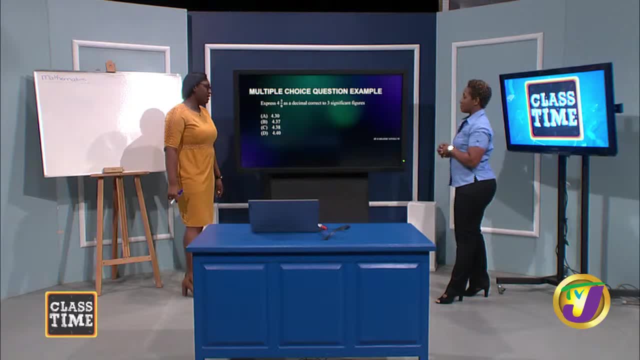 i hope you guys are following so far and you can identify what digits are. you can identify what digits are. you can identify what digits are significant and what are not significant, and what are not significant and what are not. oh boy, so now they're throwing us for. 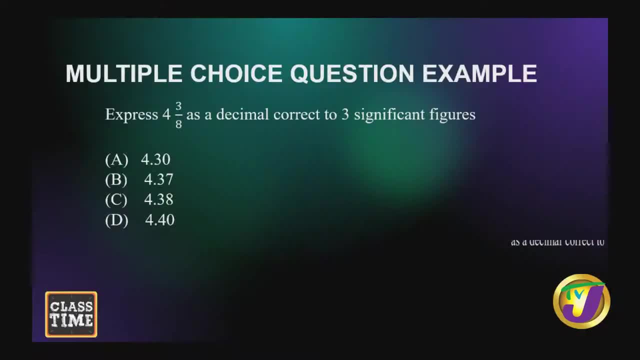 oh boy, so now they're throwing us for. oh boy, so now they're throwing us for a loop here it is that we have express a loop. here it is that we have express a loop. here it is that we have express three, sorry, express four and three. 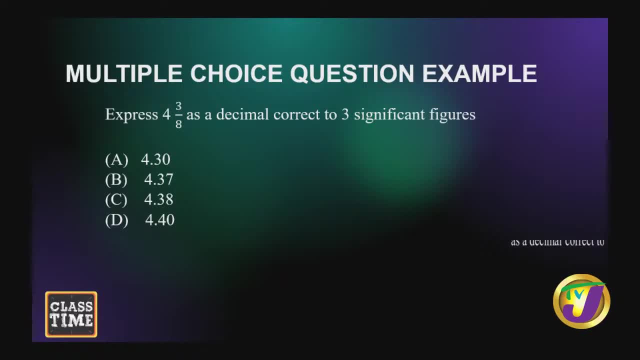 three, sorry express four and three. three, sorry express four and three. eights as a decimal correct to three. eights as a decimal correct to three. eights as a decimal correct to three. significant figures, significant figures, significant figures. now, here it is that we have a mixed 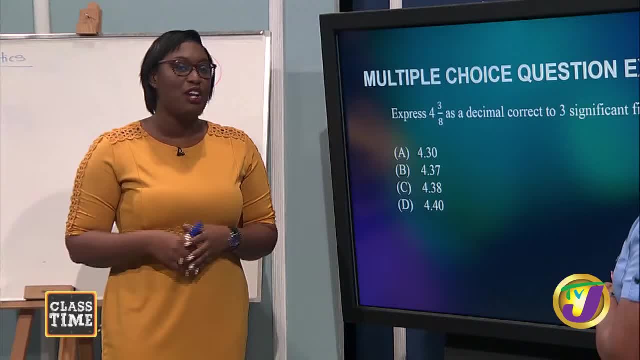 now, here it is that we have a mixed. now, here it is that we have a mixed number and we're asked to now express number, and we're asked to now express number, and we're asked to now express this mixed number as a decimal, and then this mixed number as a decimal, and then 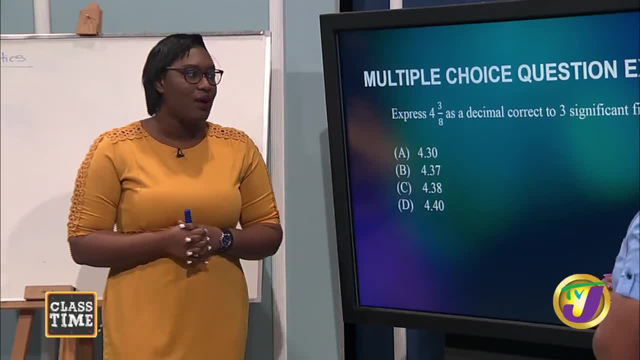 this mixed number as a decimal and then write it correct to three significant, write it correct to three significant, write it correct to three significant figures: figures, figures. all right, so how are we going to go? all right, so how are we going to go? all right, so how are we going to go about this one? all right, so we have to. 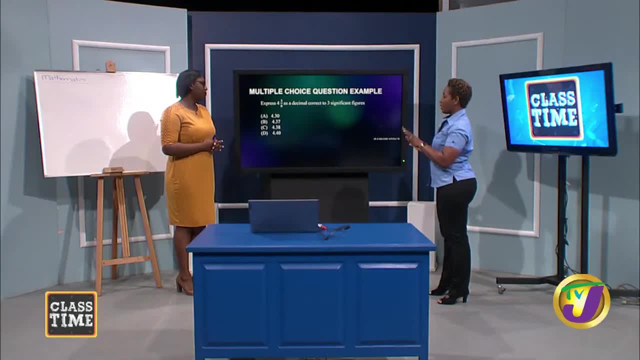 about this one. all right, so we have to. about this one. all right, so we have to convert that mixed number to a decimal. convert that mixed number to a decimal. convert that mixed number to a decimal first. okay, so we know we have four first. okay, so we know we have four. 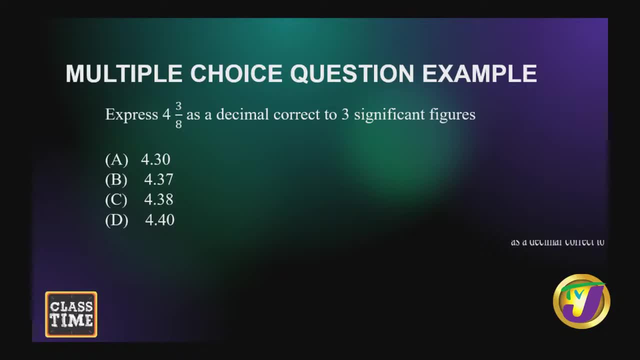 first: okay, so we know we have four holes and all the options give you the holes and all the options give you the holes and all the options give you the four holes in it. okay, three eights, four holes in it. okay, three eights, four holes in it. okay, three eights. are we going to work that out? 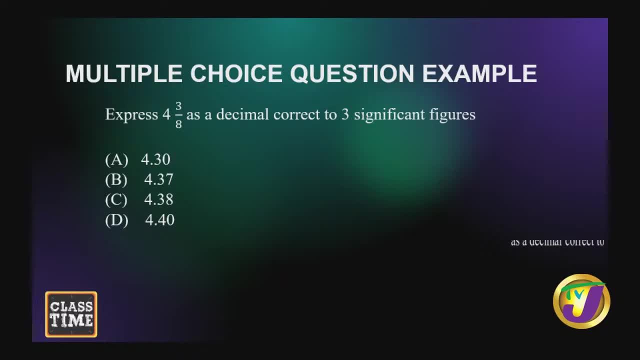 are we going to work that out? are we going to work that out? we're going to divide three by eight to. we're going to divide three by eight to. we're going to divide three by eight to get the decimal. get the decimal, get the decimal. all right, so we're going to do this on. 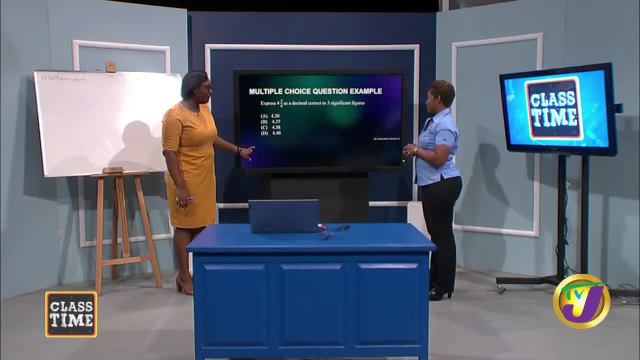 all right. so we're going to do this on all right. so we're going to do this on the board. we're going to do it on the the board. we're going to do it on the the board. we're going to do it on the screen. 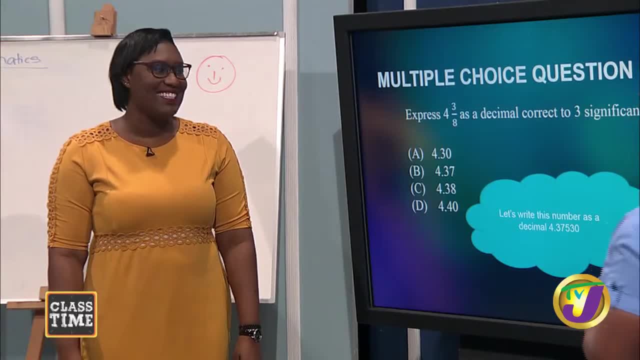 yeah man, so here we go. so we've written: yeah man, so here we go. so we've written: yeah man, so here we go. so we've written a number, a number. a number. so three eights is thirty seven thousand, so three eights is thirty seven thousand. 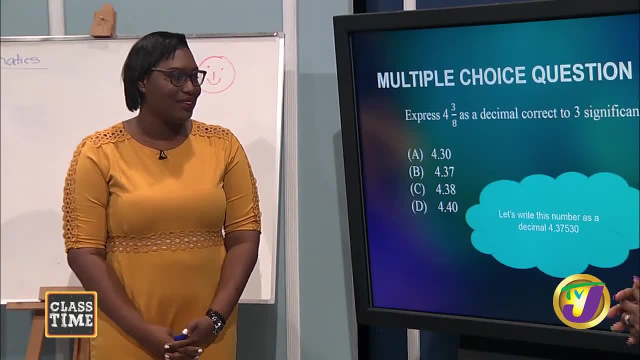 so three eights is thirty seven thousand, five hundred thirty ten thousand, five hundred thirty ten thousand, five hundred thirty ten thousand, and so that is our, that is when we, and so that is our. that is when we, and so that is our. that is when we convert four and three eights to a. 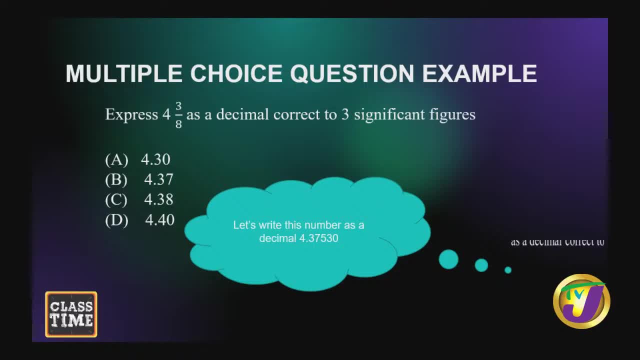 convert four and three eights to a. convert four and three eights to a decimal. all right, so two, three decimal. all right, so two, three decimal. all right, so two, three. significant figures. significant figures. significant figures: all right, you do it because you come from. all right, you do it because you come from. 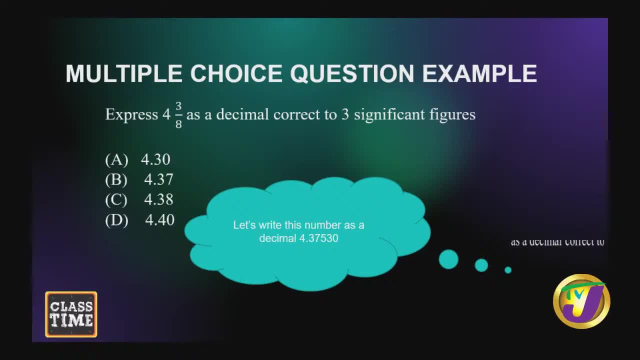 all right, you do it because you come from the left, the left, the left. all right, three significant figures, okay, all right, three significant figures, okay, all right, three significant figures, okay. so here my whole is significant. so my, so here my whole is significant. so my, so here my whole is significant. so my four is significant. 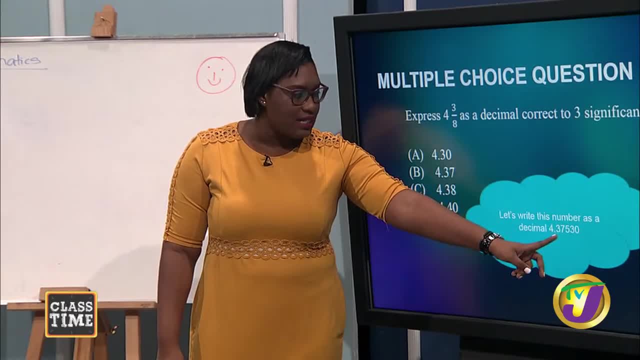 four is significant. four is significant, my three is also significant and my, my three is also significant and my, my three is also significant and my seven is significant. so there, i have, seven is significant. so there, i have, seven is significant. so there i have three significant figures. however, we need 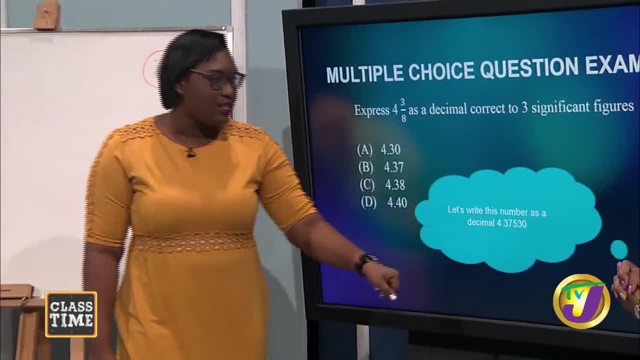 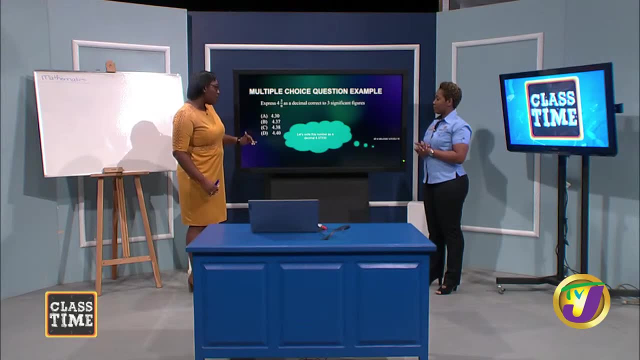 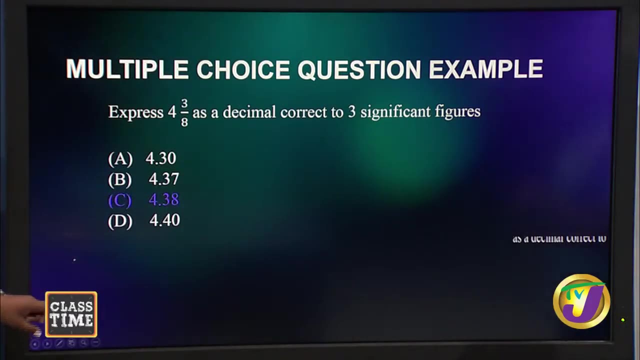 three significant figures, however. we need three significant figures. however, we need to to to 4.38 right, 4.38 right, 4.38 right, so so. so our answer would be 4.38, our answer would be 4.38, our answer would be 4.38. so we look at the number. 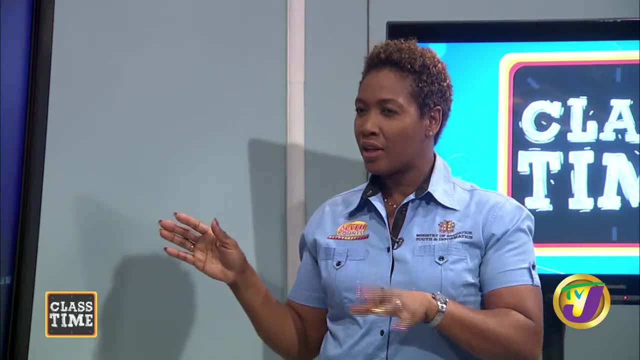 so we look at the number. so we look at the number to the right of the last significant num, to the right of the last significant num, to the right of the last significant num, last significant digit and last significant digit and last significant digit, and we see if it's closest to the next. 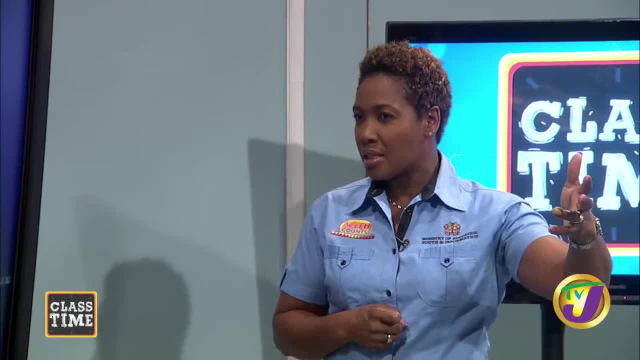 we see if it's closest to the next. we see if it's closest to the next to the next place: yes, and we add one if to the next place. yes, and we add one if to the next place. yes, and we add one. if it is, it is. 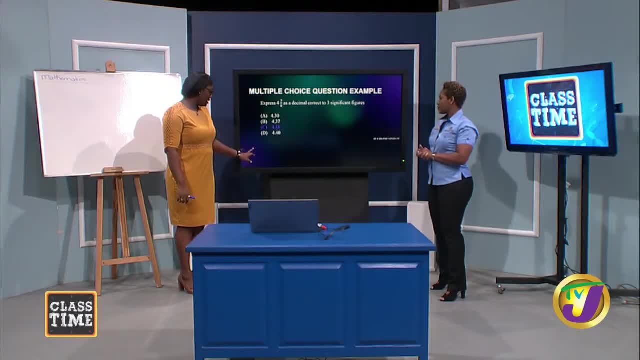 it is, and if it's not, we drop it off- yes, okay. and if it's not, we drop it off. yes, okay, and if it's not, we drop it off- yes, okay, all right, all right. so now my favorite: all right, all right. so now my favorite. 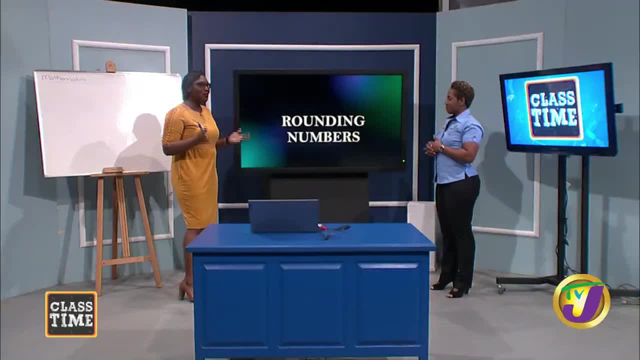 all right, all right. so now my favorite part, part part: rounding numbers. everybody must love this rounding numbers. everybody must love this. rounding numbers. everybody must love this. you know from grade seven we're rounding. you know from grade seven, we're rounding. you know from grade seven, we're rounding. we're rounding from primary school we're. 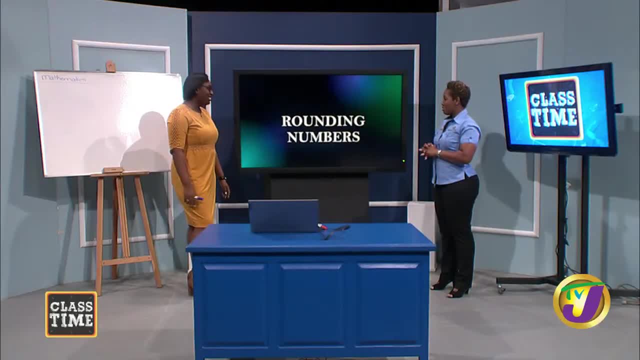 we're rounding. we're rounding from primary school. we're, we're rounding, we're rounding. from primary school. we're rounding, rounding, rounding. every time we go shop, we're rounding. every time we go shop, we're rounding. every time we go shop, we're rounding, we're estimating, we're rounding, yeah, yeah. 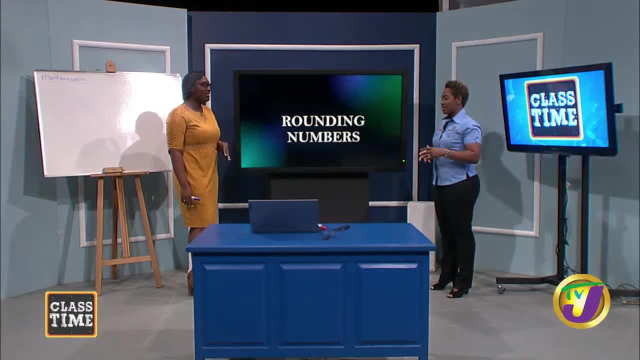 we're estimating, we're rounding. yeah, yeah, we're estimating, we're rounding, yeah, yeah, go to the supermarket. four dollars and go to the supermarket. four dollars and go to the supermarket. four dollars and fifty cents. all right, fifty cents, all right, fifty cents, all right, so so. 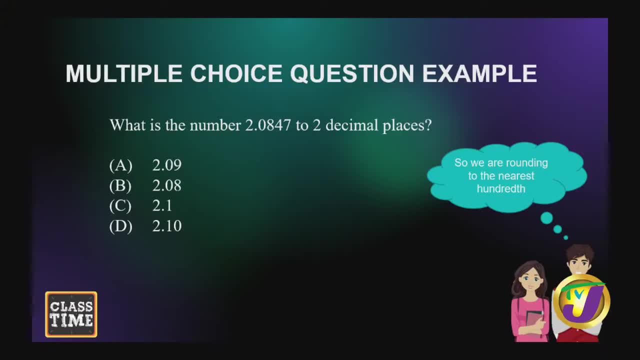 so what is the number two points zero eight? what is the number two points zero eight? what is the number two points zero eight. four, seven to two decimal places? you four, seven to two decimal places, you four, seven to two decimal places. you just love the decimal then. 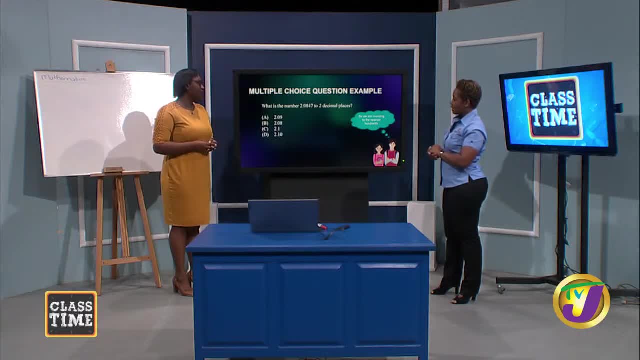 just love the decimal, then just love the decimal, then ah, ah, ah. two decimal places, so i know my decimal. two decimal places, so i know my decimal. two decimal places, so i know my decimal. and then zero my first decimal place it. and then zero my first decimal place it. 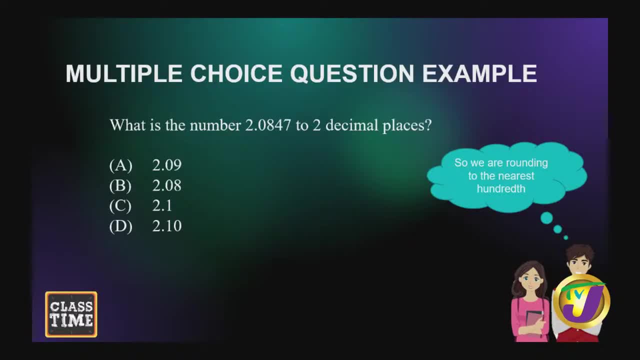 and then zero: my first decimal place. it is my second decimal place. is my second decimal place? is my second decimal place? all right, i know i can't just drop it. all right, i know i can't just drop it. all right, i know i can't just drop it off. i have to pay attention to. so i have. 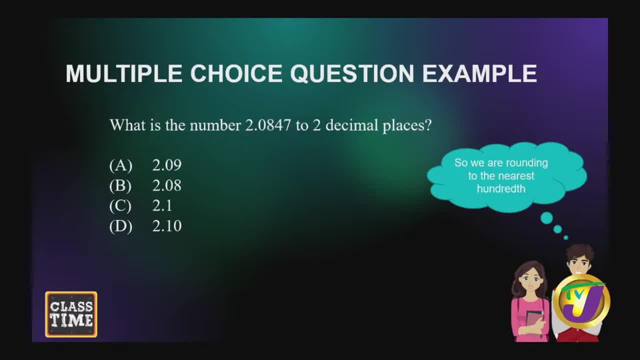 off i have to pay attention to. so i have off i have to pay attention to. so i have my tenth, my hundredth, my thousandth, my tenth, my hundredth, my thousandth, my tenth, my hundredth, my thousandth place. i have to pay attention to the. 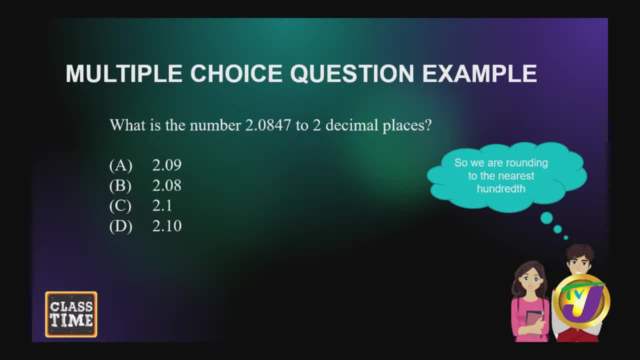 place. i have to pay attention to the place. i have to pay attention to the digit in my thousandth place. all right. digit in my thousandth place, all right. digit in my thousandth place, all right, and that is and that is and that is not. it's not even halfway, so i'm going. 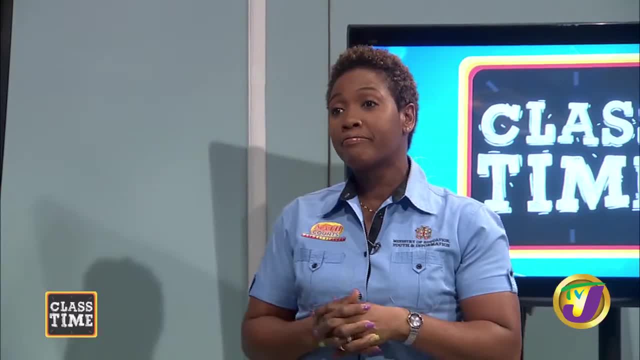 not, it's not even halfway, so i'm going. not, it's not even halfway, so i'm going to make it's going to be 2.08. to make it's going to be 2.08. to make it's going to be 2.08, all right. so again we're rolling into. 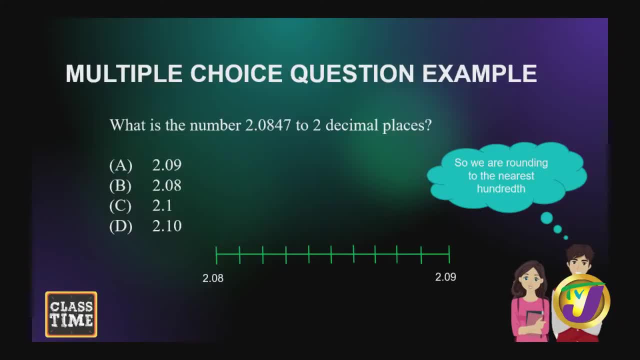 all right. so again we're rolling into. all right. so again we're rolling into. the nearest hundredth this time around. the nearest hundredth this time around, the nearest hundredth this time around. let's see, let's see, let's see. so here we have our number line, so we 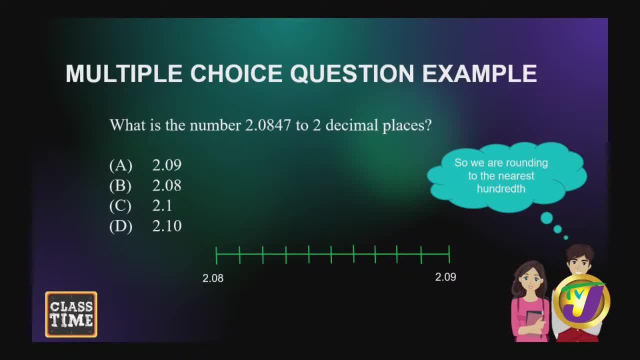 so here we have our number line, so we. so here we have our number line, so we have a number line. now guys have a number line. now guys have a number line. now, guys, and again we're going to place our number, and again we're going to place our number. 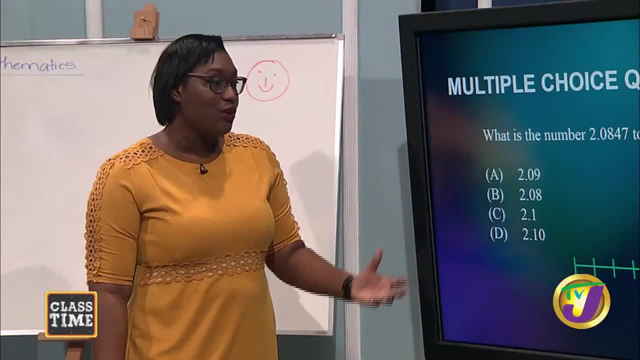 and again, we're going to place our number on the number line and as tamika on the number line and as tamika on the number line, and as tamika rightfully said, rightfully said, rightfully said, it is closer to 2.08. it is closer to 2.08. 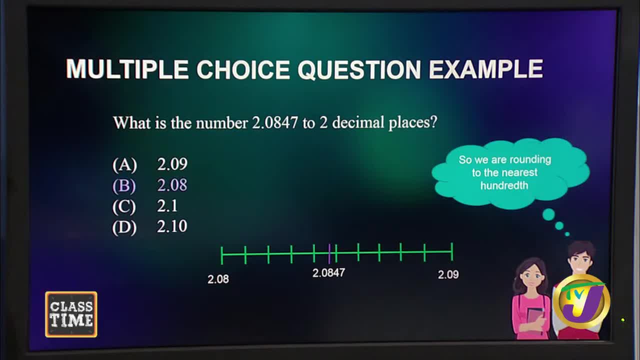 it is closer to 2.08, or or or two and eight hundreds right, and so my two and eight hundreds right, and so my two and eight hundreds right, and so my answer is: answer is: answer is b right, all right, so this is also a b right, all right, so this is also a. b right, all right. so this is also a visual that you guys can look at. you can visual that you guys can look at. you can visual that you guys can look at. you can see it on the lumber line and the. see it on the lumber line and the. 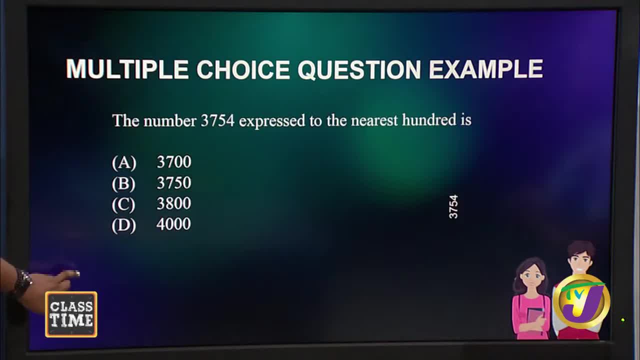 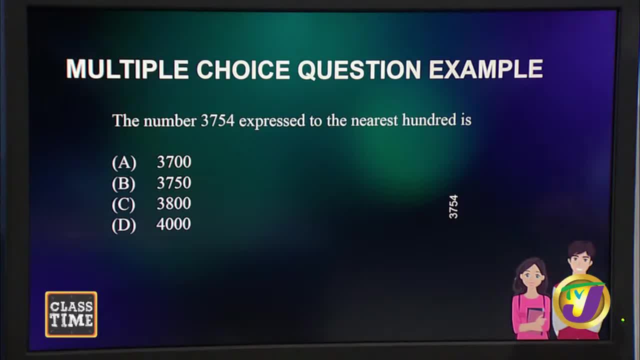 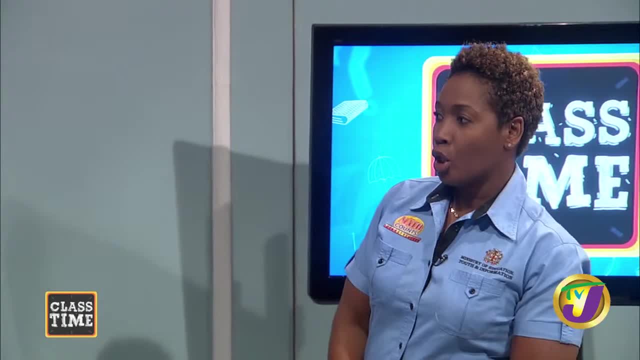 express to the nearest hundred. express to the nearest hundred. so i would like to look at the digit in. so i would like to look at the digit in. so i would like to look at the digit in the hundredth place, the hundredth place, the hundredth place in the hundred place, and that would be. 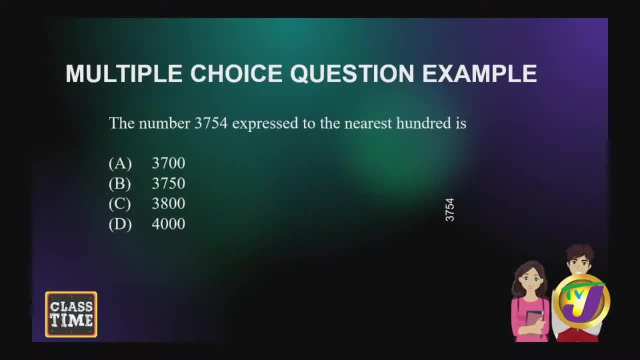 in the hundred place, and that would be in the hundred place and that would be seven, seven, seven. all right, so we are working in base 10. all right, so we are working in base 10. all right, so we are working in base 10 and every digit is: 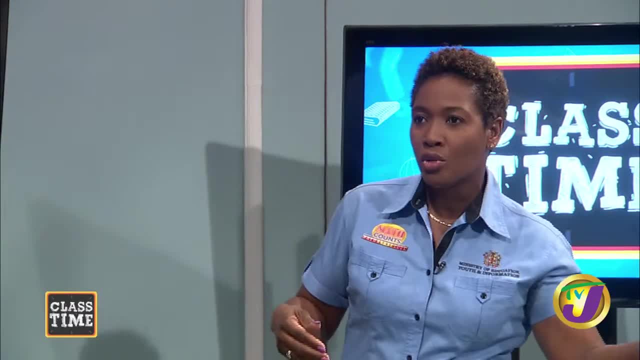 and every digit is, and every digit is um would have been: if you reach 10 in, um would have been: if you reach 10 in, um would have been: if you reach 10 in that place, that place, that place, you would regroup it to the next place. 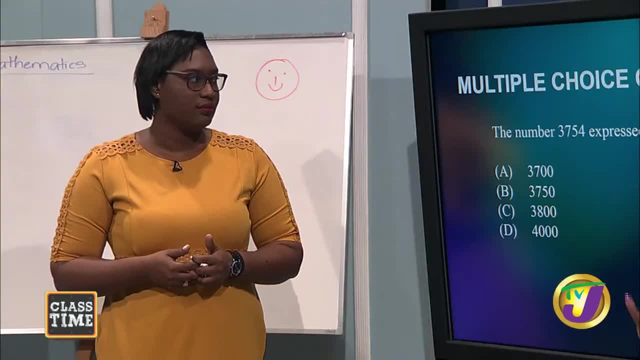 you would regroup it to the next place. you would regroup it to the next place, to the place to the, to the place to the, to the place to the. that's left all right, so i'm in my. that's left all right, so i'm in my. 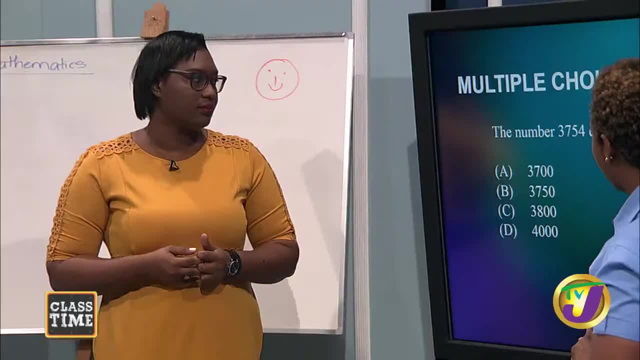 that's left, all right. so i'm in my hundred place, which is seven hundred place, which is seven hundred place, which is seven. let me look at my 10th place, my 10th. let me look at my 10th place, my 10th. 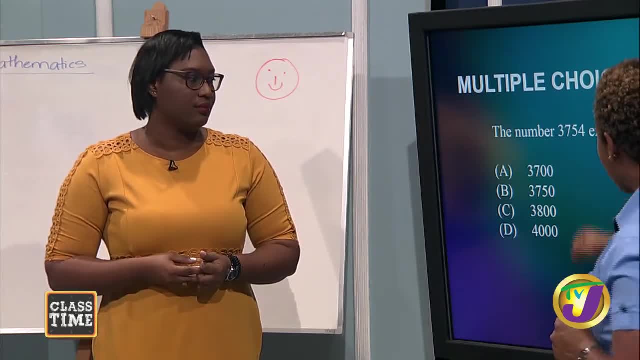 let me look at my 10th place, my 10th place. why do i place? why do i place? why do i? i'm still in the decimal in my 10th place. i'm still in the decimal in my 10th place. i'm still in the decimal in my 10th place. i have 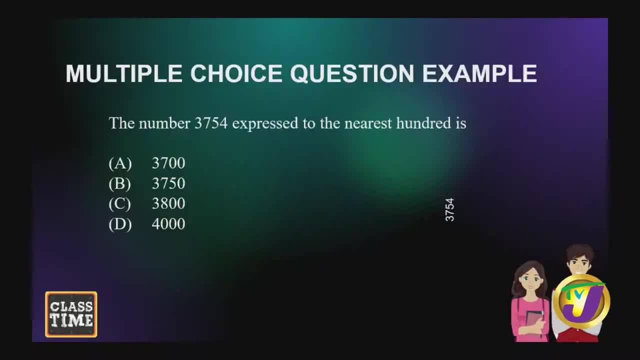 i have. i have five. five is five, five is five. five is pretty much. you know 54. 50- all right, pretty much. you know 54. 50- all right, pretty much. you know 54. 50, all right, okay, 54, it got good world. that's up to a. 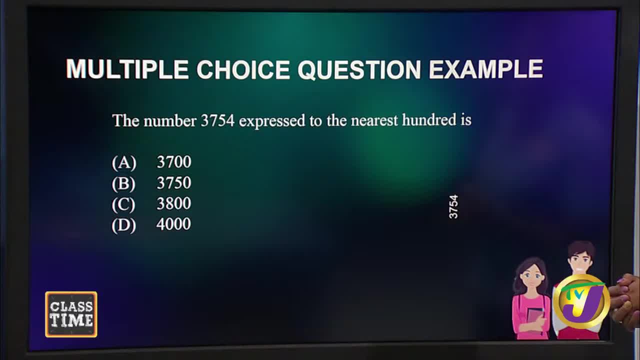 okay, 54, it got good. world that's up to a. okay, 54, it got good world that's up to a hundred. you know hundred, you know hundred. you know it's closer to the next hundred. okay, it's closer to the next hundred. okay, it's closer to the next hundred. okay, all right. so let's, let's take a look. 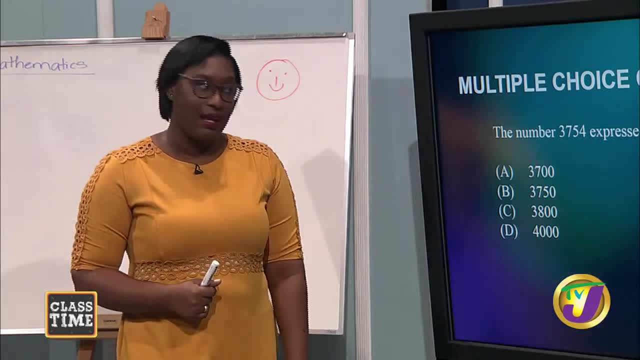 all right. so let's, let's take a look. all right, so let's, let's take a look again. so again, guys, again, so again, guys, again, so again, guys. we're going back to our number line and we're going back to our number line and we're going back to our number line and we're going to place our number on our 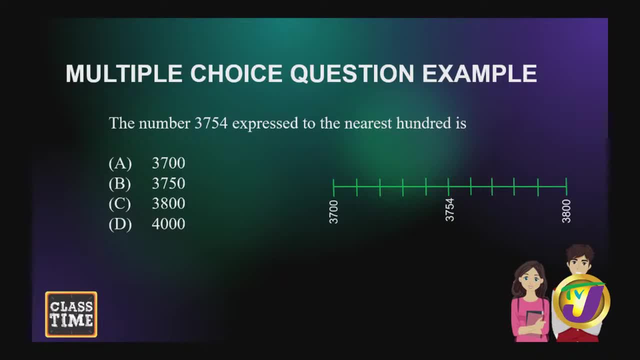 we're going to place our number on our, we're going to place our number on our number line. so the nearest hundreds number line, so the nearest hundreds number line, so the nearest hundreds. we're looking at right so we're close to. we're looking at right, so we're close to. 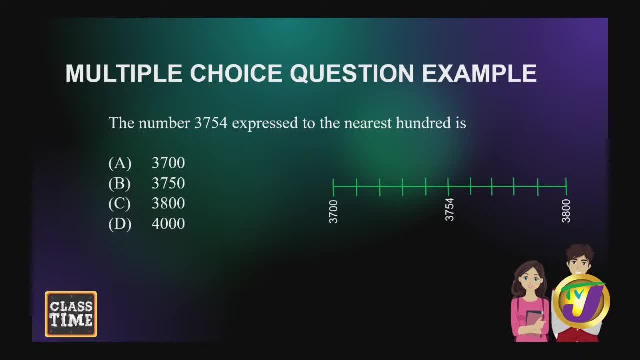 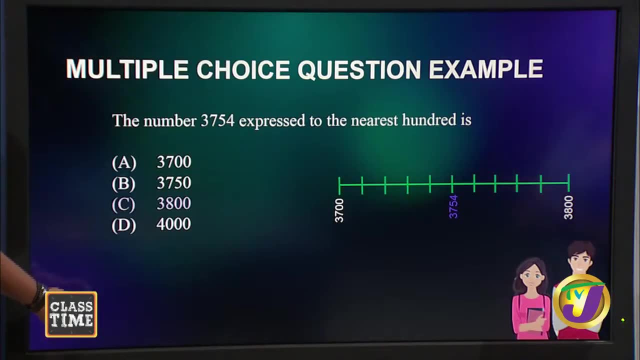 we're looking at right, so we're close to 3700 or 3800, 3700 or 3800, 3700 or 3800 and, as you rightfully, as you said, and as you rightfully, as you said, and as you rightfully, as you said, so, as you said, we are. 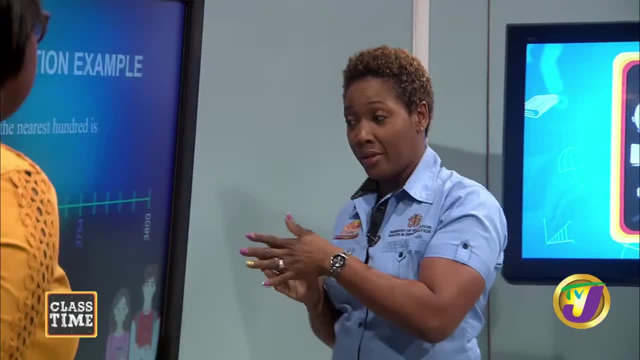 so as you said, we are. so as you said we are, but going brittany before you move on, but going brittany before you move on, but going brittany before you move on. it's halfway in there now. it's halfway in there now. 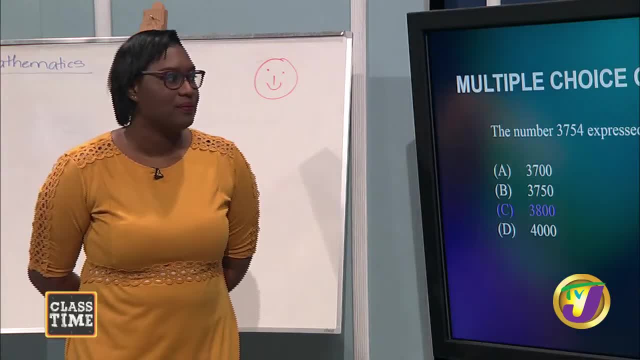 it's halfway in there now, yes and so because it's halfway there, yes and so because it's halfway there, yes and so because it's halfway there. so why i couldn't just call it 3700? so why i couldn't just call it 3700? 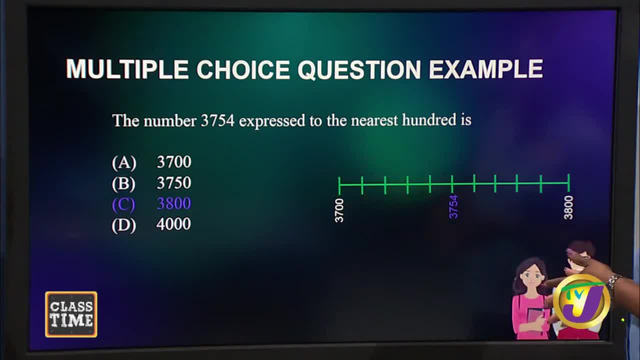 so why i couldn't just call it 3700, conventionally? i guess you, you don't conventionally. i guess you, you don't conventionally, i guess you, you don't want to lose your 54, want to lose your 54, want to lose your 54 dollars? it's 50 is money. no, you're 54. 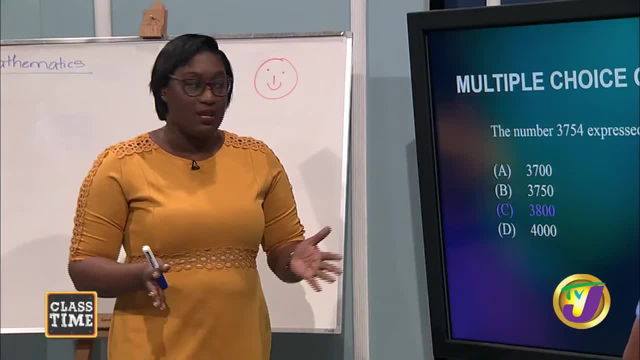 dollars. it's 50 is money? no, you're 54 dollars. it's 50 is money? no, you're 54. okay, um well, so it's equidistance. okay, um well, so it's equidistance. okay, um well, so it's equidistance between. 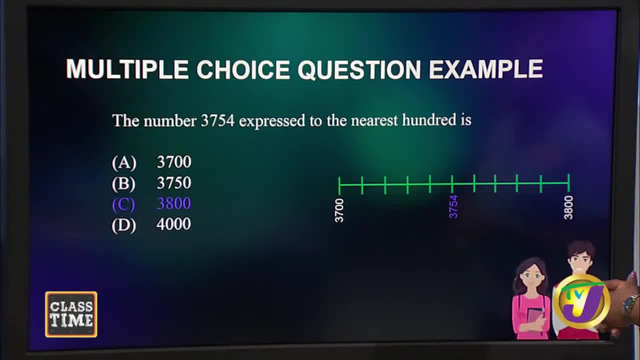 between between 3700 and 3800, but convention has it 3700 and 3800, but convention has it 3700 and 3800. but convention has it that when it's equidistant, that when it's equidistant, that when it's equidistant, we tend to go higher and not lower. so 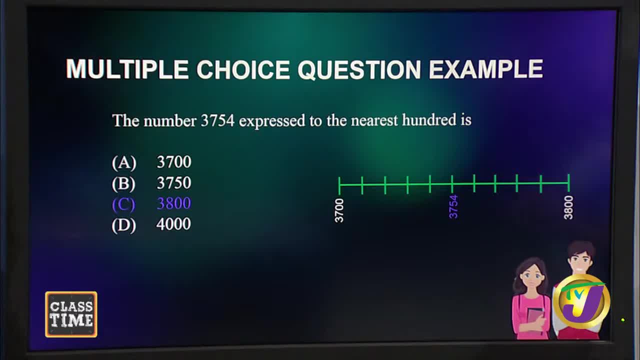 we tend to go higher and not lower. so we tend to go higher and not lower. so hence why we will now round it. hence why we will now round it. hence why we will now round it to 30: 3800. oh right, okay. to 30: 3800: oh right, okay. 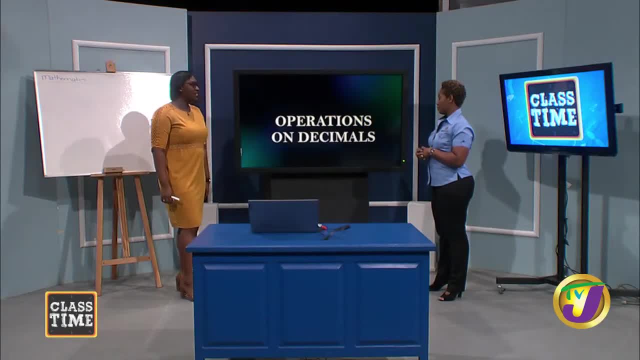 to 30: 3800. oh right, okay, all right. operations on boy the decimals guys. ah, operations on boy the decimals guys. ah, operations on boy the decimals guys. ah, geez, geez, geez. it's like we're all decimals out this. it's like we're all decimals out this. 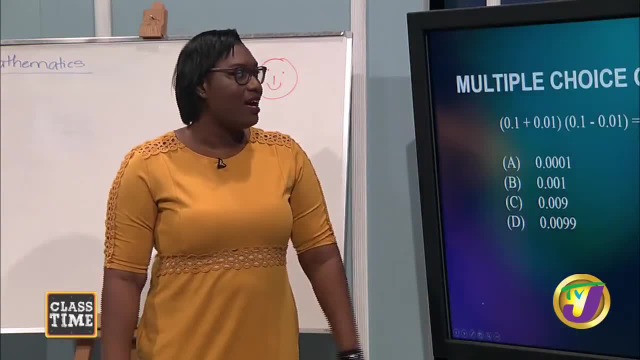 it's like we're all decimals out this morning, so we're going on to operations morning, so we're going on to operations morning, so we're going on to operations on decimals, on decimals, on decimals. all righty, oh wow, all righty, oh wow, all righty, oh wow, yay, this is unique, yay. 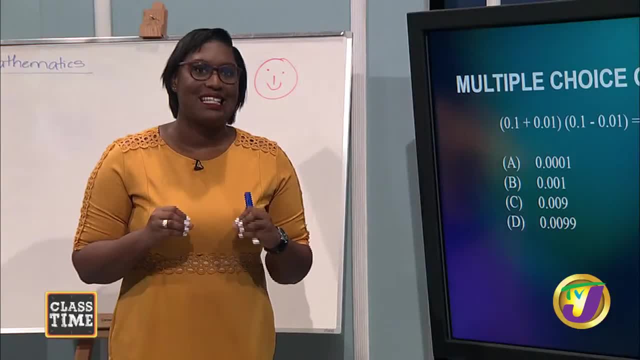 yay, this is unique. yay, yay, this is unique. yay, we're still relaxing, right, don't forget. we're still relaxing, right, don't forget, we're still relaxing, right, don't forget. guys, guys, guys, relax. so we're looking at the multiple relax. so we're looking at the multiple. 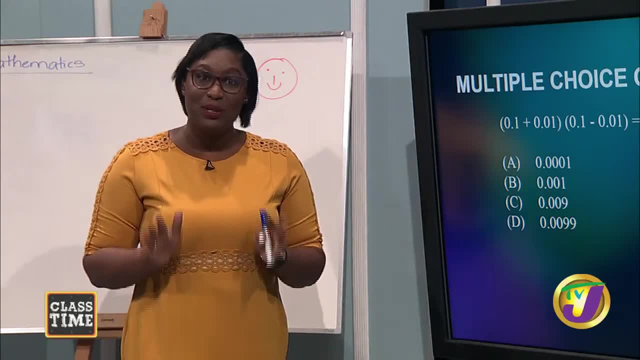 relax. so we're looking at the multiple choice questions, choice questions, choice questions, and we're remembering one of the and we're remembering one of the and we're remembering one of the strategies we're using is strategies we're using is strategies we're using is relaxation, because we got this right. 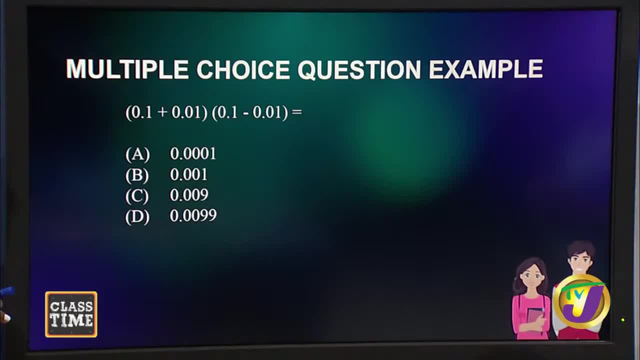 relaxation because we got this right. relaxation because we got this right. so i'm relaxing all right, so i'm so i'm relaxing all right, so i'm, so i'm relaxing all right. so i'm reading the question, reading the question, reading the question. i'm rereading the question, all right, i. i'm rereading the question, all right. i i'm rereading the question, all right. i think we should set this up on the board. think we should set this up on the board. think we should set this up on the board just to let them see. 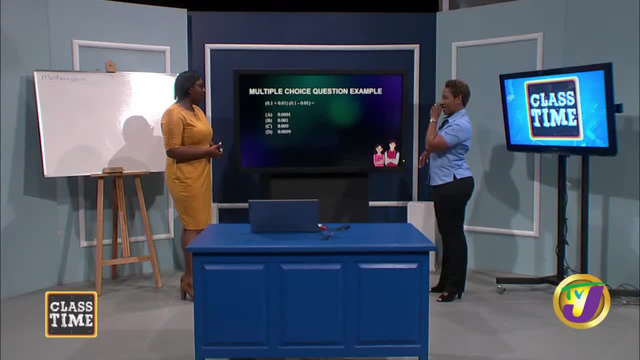 just to let them see. just to let them see how to to, to make sure they write this, how to to, to make sure they write this, how to to, to make sure they write this down properly, down properly, down properly. what do you think all right so? what do you think all right so? 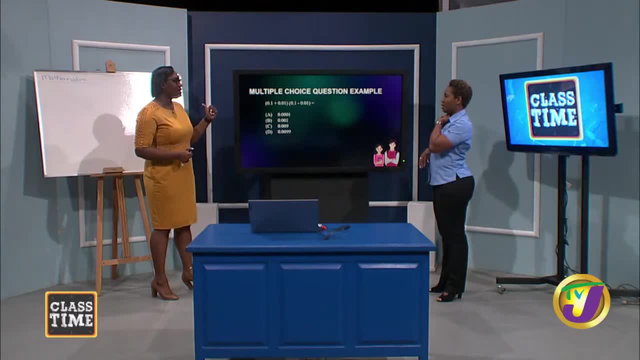 what do you think? all right? so, firstly, we have several things happening. firstly, we have several things happening. firstly, we have several things happening in this question, right in this question, right in this question, right, all right, so we're adding, we're all right, so we're adding, we're. 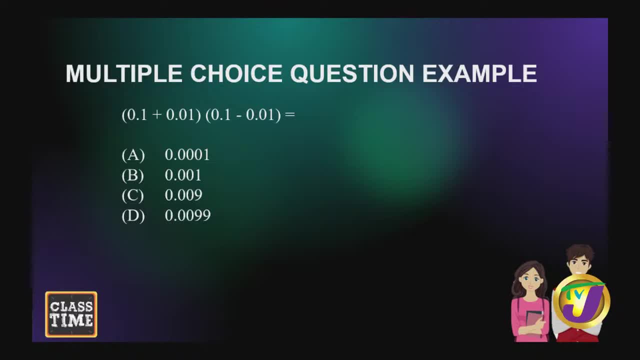 all right. so we're adding, we're subtracting decimals, and we're also subtracting decimals, and we're also subtracting decimals, and we're also multiplying operations. indeed, all right, multiplying operations. indeed, all right, multiplying operations, indeed all right. so, jenny and jack, so, jenny and jack. 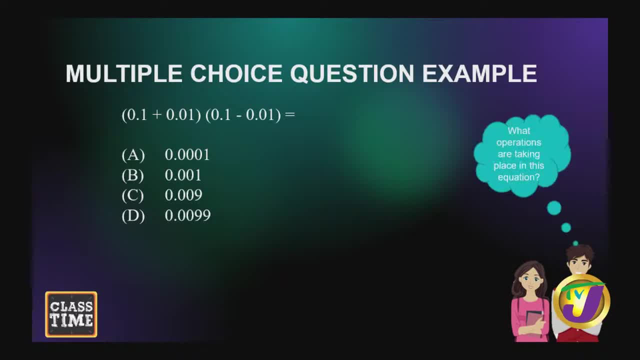 so jenny and jack, we love jenny, i'm a love jack. we love jenny, i'm a love jack. we love jenny, i'm a love jack. what operations we tell them already. what operations we tell them already. what operations we tell them already right. addition, subtraction, multiplication. 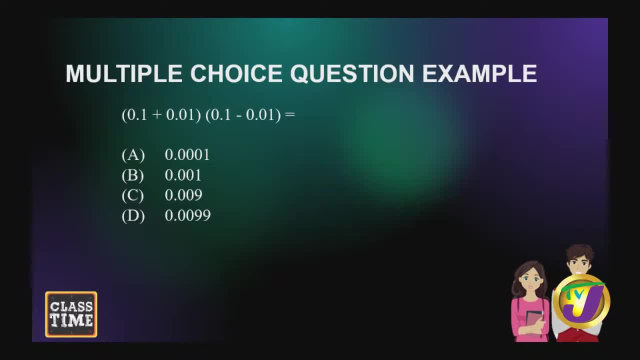 right addition subtraction multiplication. right addition subtraction multiplication. we're good, jenny and jack won't come to. we're good, jenny and jack won't come to. we're good, jenny and jack won't come to the rescue. so, guys, the rescue, so guys, the rescue. so, guys, we have it set up for you, right? so? 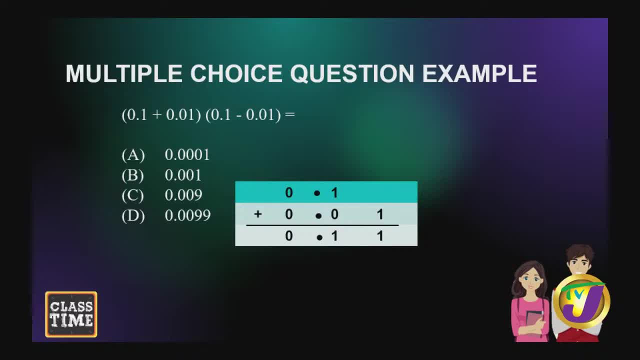 we have it set up for you right. so we have it set up for you right. so holes are in our ones place, or holes are in our ones place, or holes are in our ones place, or all the digits are in the tenths place. all the digits are in the tenths place. 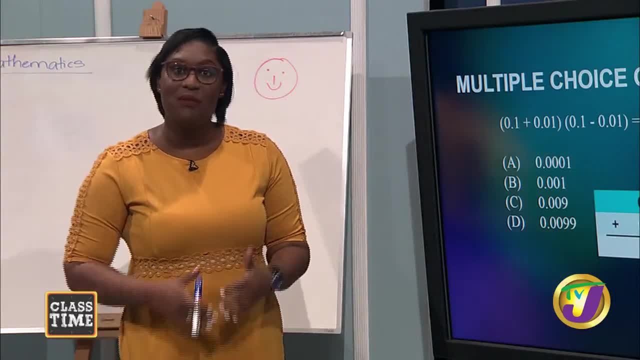 all the digits are in the tenths place and we have one digit in the hundredths and we have one digit in the hundredths and we have one digit in the hundredths: place, place, place. so it's important that we maintain that. so it's important that we maintain that. 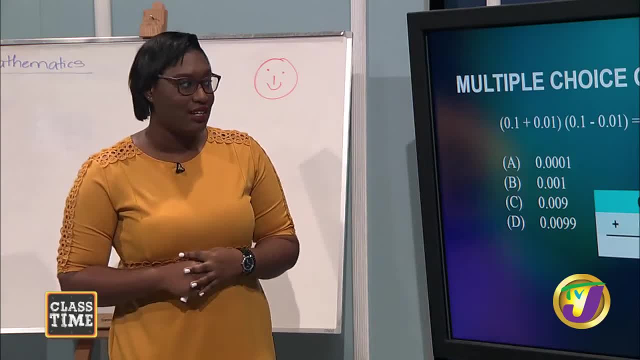 so it's important that we maintain that integrity, integrity, integrity, all right. and then we went ahead and all right, and then we went ahead, and all right, and then we went ahead and did the addition, did the addition, did the addition. so one is added to nothing, we get one. 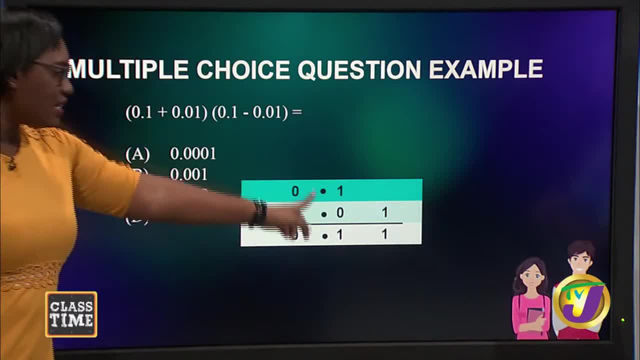 so one is added to nothing. we get one. so one is added to nothing. we get one. one is added to zero, we get one. one is added to zero. we get one. one is added to zero. we get one. and we notice our decimal, and we notice our decimal. 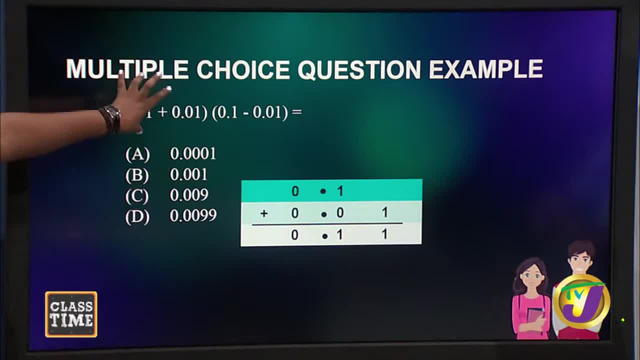 and we notice our decimal still maintained. so it's actually 0.11 still maintained. so it's actually 0.11 still maintained. so it's actually 0.11 for our first, for our first, for our first brackets. so one tenth plus one hundredth. 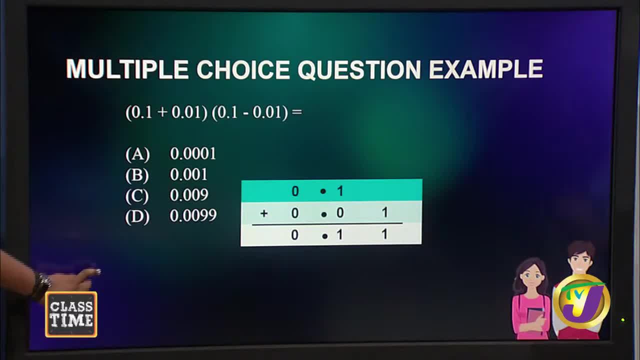 brackets, so one tenth plus one hundredth. brackets, so one tenth plus one hundredth. gives us, gives us, gives us 1100, yes, okay, 1100, yes, okay, 1100, yes, okay, all right, all right, all right, jenny and jack got us today guys. 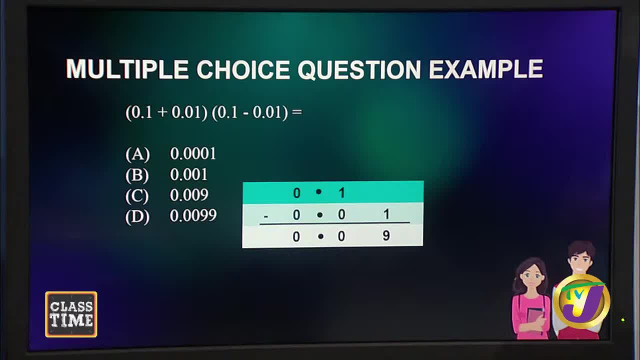 jenny and jack got us today, guys. jenny and jack got us today, guys. all right, so now we're subtracting. all right, so now we're subtracting. all right, so now we're subtracting. so we have one. we have one tenth. so we have one, we have one tenth. 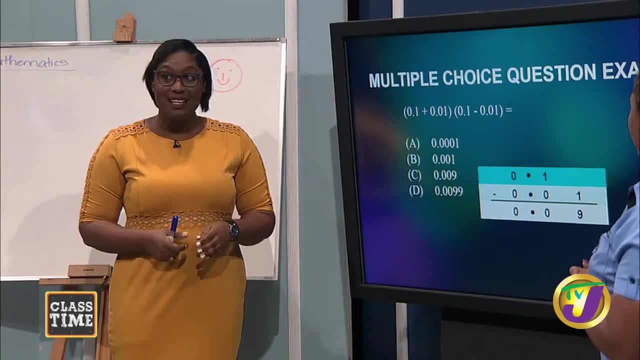 so we have one, we have one tenth. subtract one hundredth, ah, all right. so subtract one hundredth, ah, all right, so subtract one hundredth, ah, all right. so jenny and jack went ahead, and jenny and jack went ahead, and jenny and jack went ahead, and you know we'll get not 900. yes, 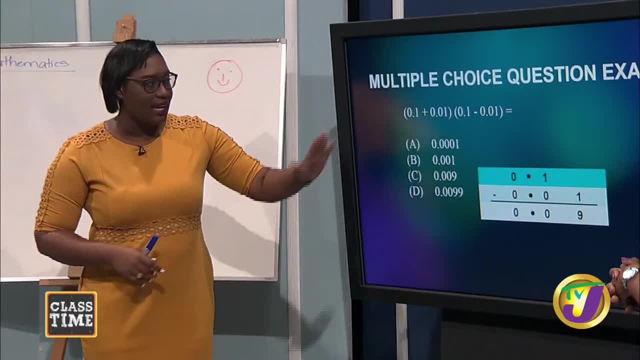 you know we'll get not 900. yes, you know we'll get not 900. yes, gotcha, so it's gotcha, so it's gotcha, so it's, so it's again, ensure that our place, so it's again, ensure that our place, so it's again, ensure that our place values are maintained, because that is. 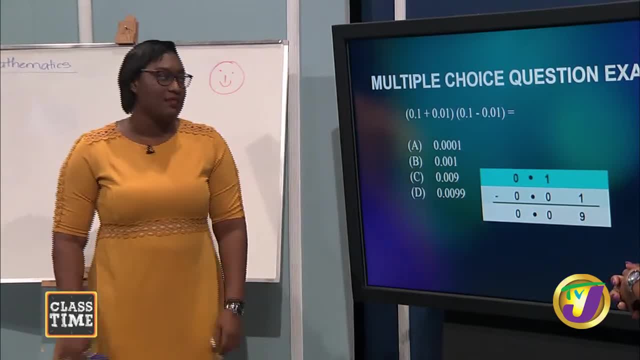 values are maintained, because that is, values are maintained, because that is extremely important, extremely important, extremely important. and when we subtract we got, and when we subtract we got, and when we subtract we got. nine hundredth now, that's not it. nine hundredth now, that's not it. 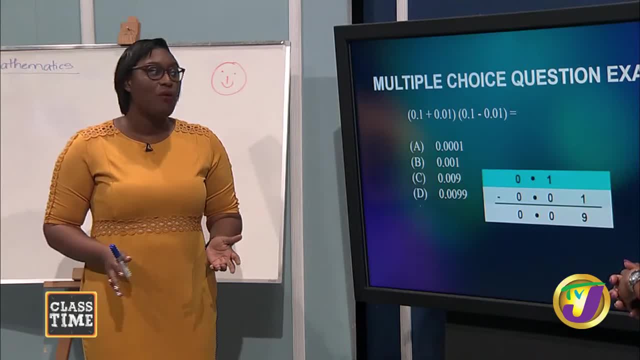 nine hundredth. now, that's not it. so our second bracket resulted in: so our second bracket resulted in. so our second bracket resulted in nine hundredth. we have nine hundredth being nine hundredth. we have nine hundredth being nine hundredth. we have nine hundredth being multiplied by what was the second it. 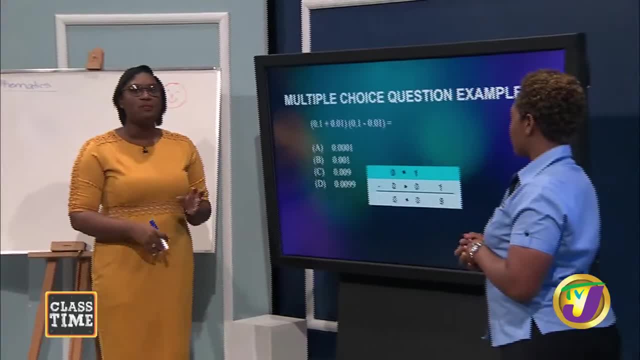 multiplied by what was the second, it multiplied by what was the second, it was eleven hundred eleven hundredths was eleven hundred eleven hundredths was eleven hundred eleven hundredths. so when we multiply nine hundredths by, so, when we multiply nine hundredths by, so, when we multiply nine hundredths by eleven hundredths, 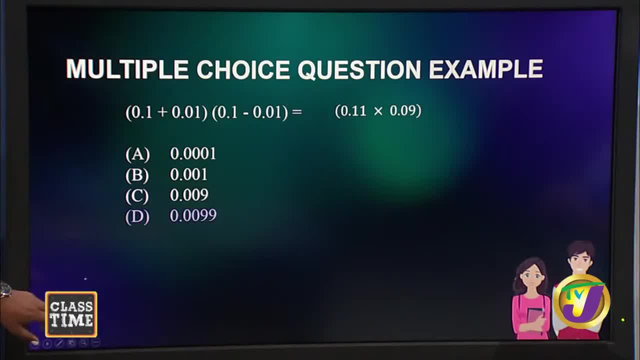 eleven hundredths, eleven hundredths, ah, ah, ah, dum dum dum. so the answer for this one is d dum dum dum. so the answer for this one is d dum dum. so the answer for this one is d. it would have been 0.0099. and again, guys. 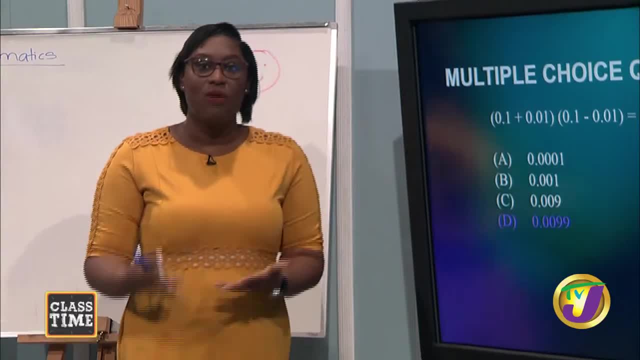 it would have been 0.0099. and again, guys, it would have been 0.0099. and again, guys, relax, relax. i didn't do it here, but i relax, relax. i didn't do it here, but i relax, relax. i didn't do it here, but i want for you guys to check over your. 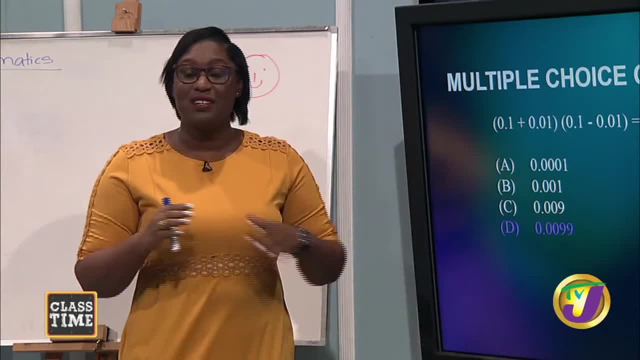 want for you guys to check over your want for you guys to check over your work. ensure that you, you know you don't work. ensure that you, you know you don't work. ensure that you, you know you don't just run through this because you're just run through this, because you're. 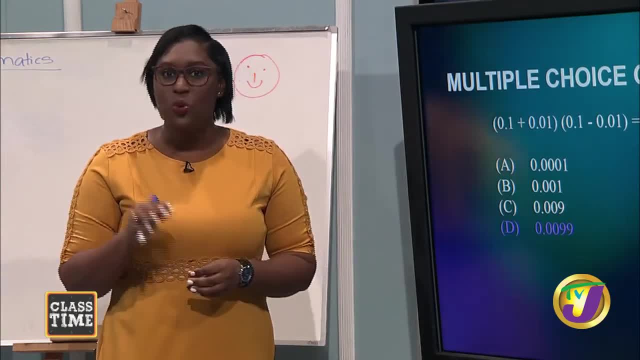 just run through this, because you're multiplying decimals, you're adding multiplying decimals. you're adding multiplying decimals. you're adding decimals. you're subtracting decimals, decimals- you're subtracting decimals, decimals, you're subtracting decimals. you may make a mistake, relax. you may make a mistake, relax. 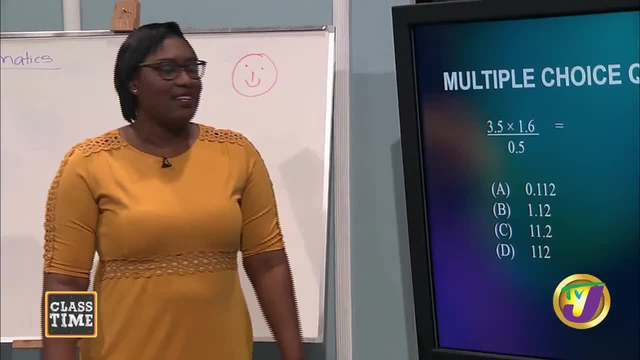 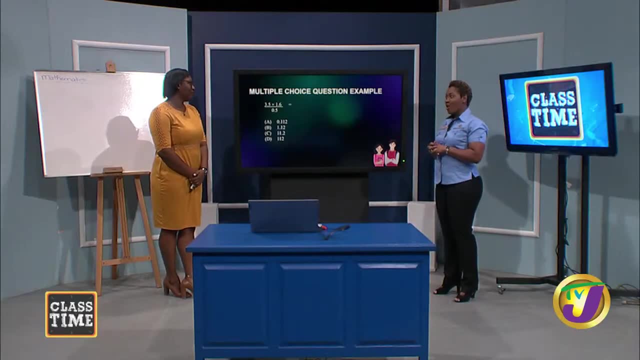 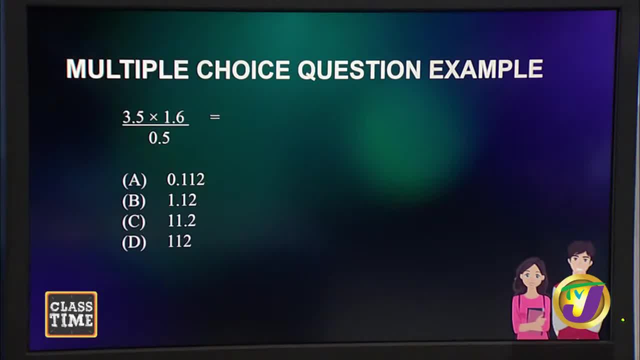 and six tenths all divided by, and six tenths all divided by: five tenths looking good, five tenths looking good, five tenths looking good. there's a lot of operations in this one. there's a lot of operations in this one. there's a lot of operations in this one. we're multiplying. 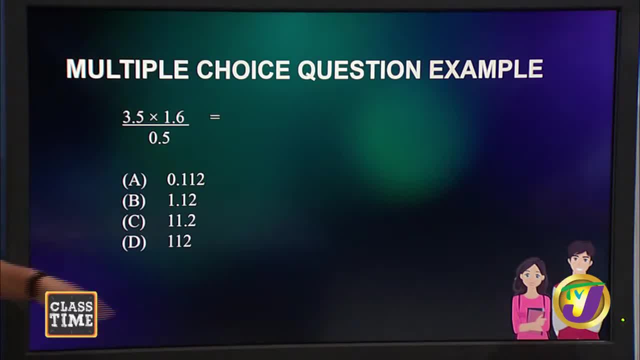 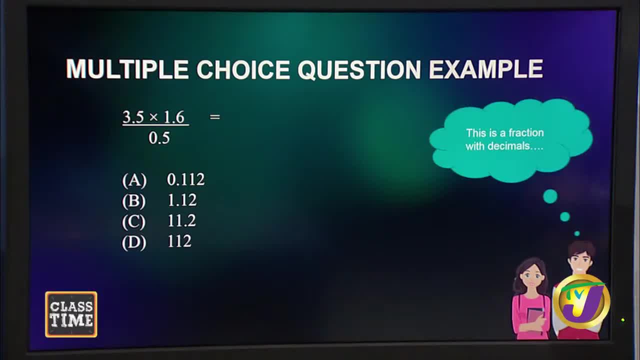 let's do like a jack drill: yeah, what you have to say, you have to say, you have to say all right. so this is a fraction with all right. so this is a fraction with all right. so this is a fraction with decimals most definitely, decimals most definitely. 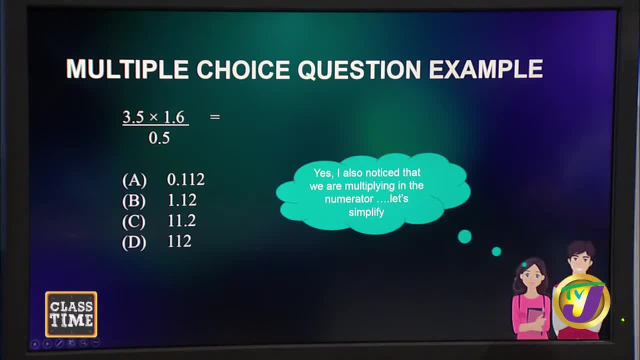 decimals. most definitely all right. i also noticed that we're multiplying in. i also noticed that we're multiplying in. i also noticed that we're multiplying in the numerator, the numerator, the numerator. let's simplify. all right, let's simplify. let's simplify. all right, let's simplify. 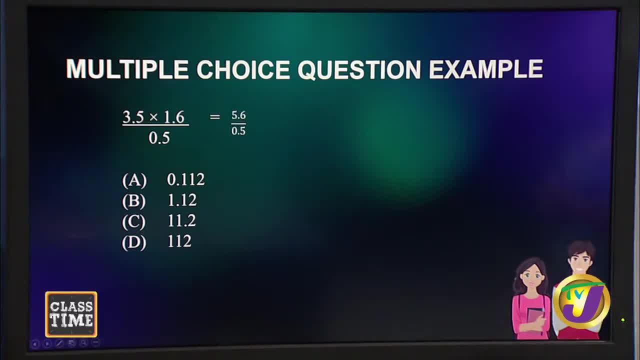 let's simplify, all right, let's simplify. so jenny's on a path here, guys. so jenny's on a path here, guys. so jenny's on a path here, guys, all right. so they have simplified by. all right. so they have simplified by all right. so they have simplified by multiplying 3.5 times 1.6, giving us 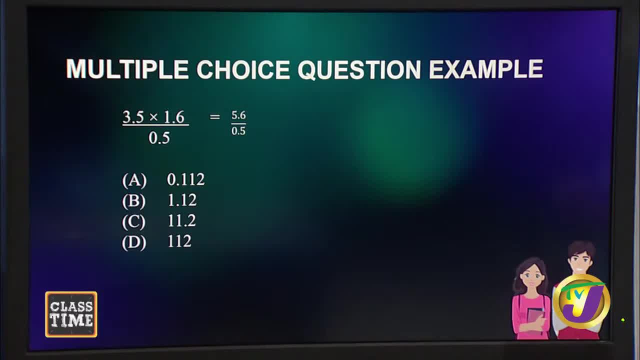 multiplying 3.5 times 1.6, giving us Alright. so now we have another question in this section: operations on decimals. So now we have: we have 3.3 multiplied by 2.2, plus 5.7 multiplied by 2.5.. 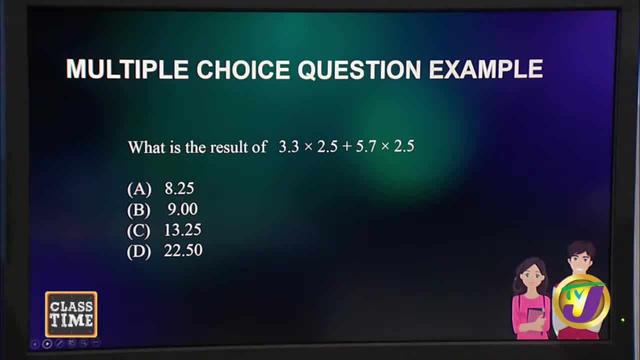 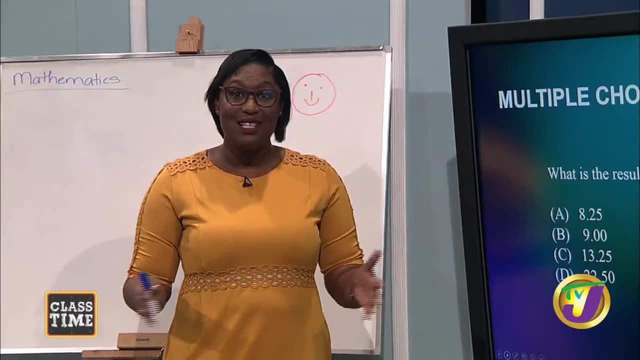 Here it is that we're multiplying and we're adding and, as you can see, and as you can see, there are no brackets. What am I going to do now? No brackets are there, so which one are the first? Do I just run in and do anything? 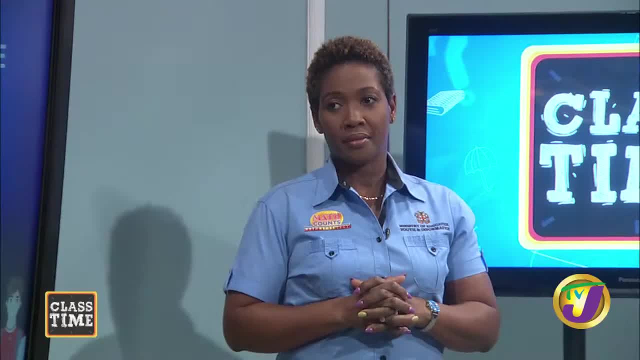 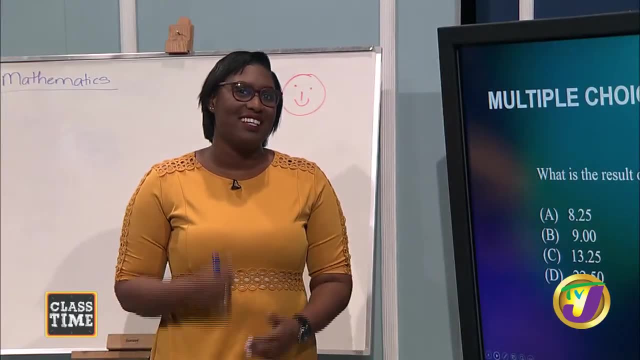 Guys tell us at home what we do. Well, you know what to do. You know to follow the order of operations. You know this: That's some order of operations: Pim das, bum das, all of those things. you know that man, so pull back on that. 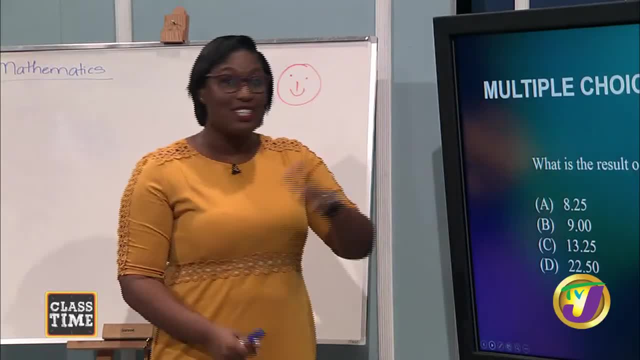 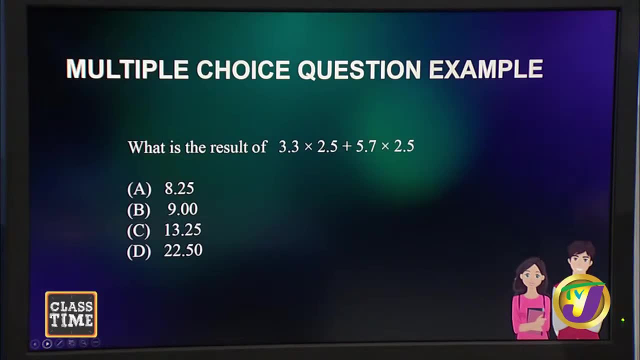 Okay, I hope you guys know it at home too. So let us start. Let us draw for the order of operations. As you rightfully said, we're going to multiply first. So we're going to multiply 3.3 by 2.5, okay- and then add the two products. 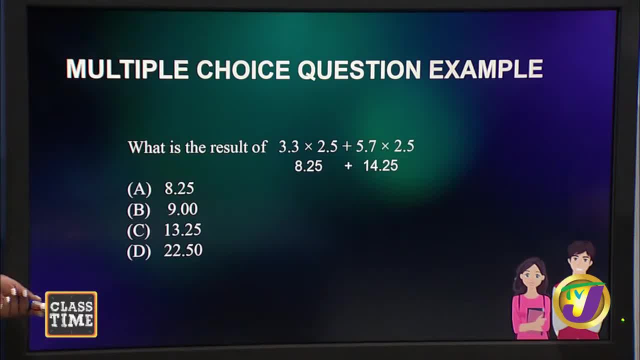 So we're going to multiply 3.3 by 2.5 and we get 8.25.. Then we're going to add the results of multiplying 5.7 by 2.5 and we're going to get 14.25.. 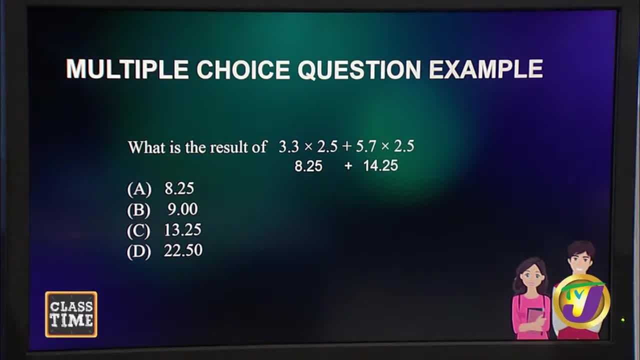 There you go. Whew, that's a lot of talking, that's a lot of math. Yep, Right. So, as you can see, the products. we're now going to go ahead and add the products to get our results. All right. so for this one now. 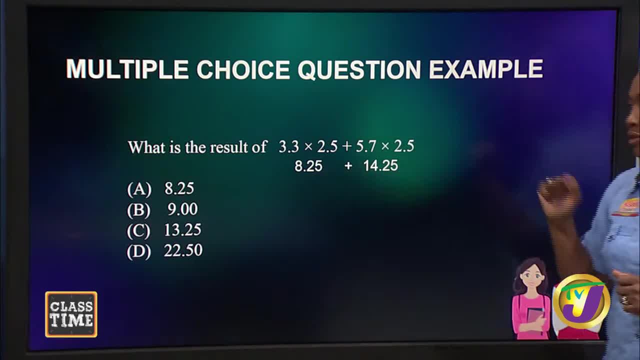 And Brittany, right away from observation, 0.25, and 0.25 is going to give us 0.5.. Yes, So if you look at the option, you kind of just want to confirm, but you kind of only have one option. 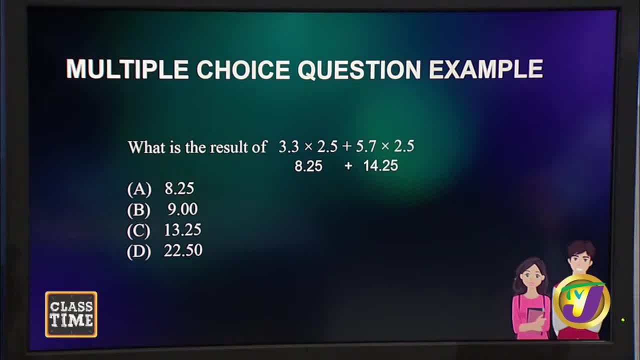 Look at that. Are we doing something from our relax? We are eliminating some of our responses. Yes, we are. Yes, we are, And then again we can check back now so we can actually do the math. We eliminated some of the answers, right. 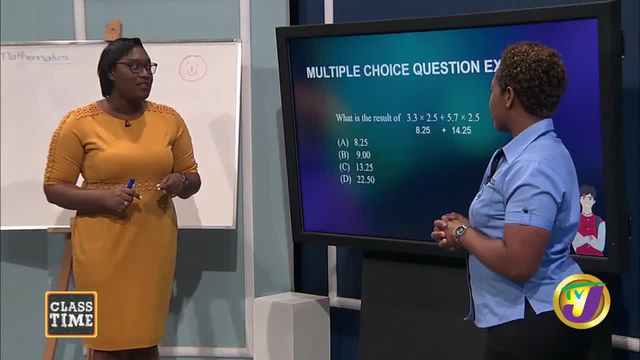 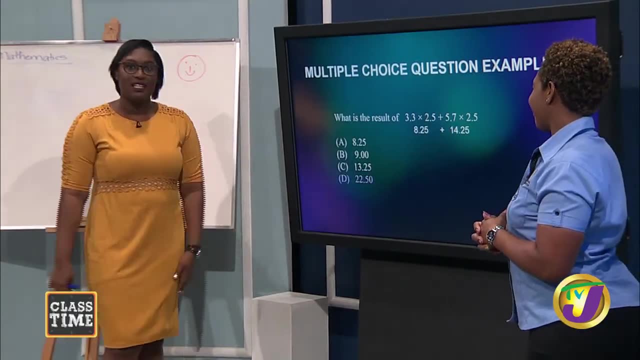 We can now check back by doing the math and doing the addition, And we know that 8 plus 14 will give us 22.. There you go, Right, We just check it back, All right. So, guys, our answer is 22.50.. 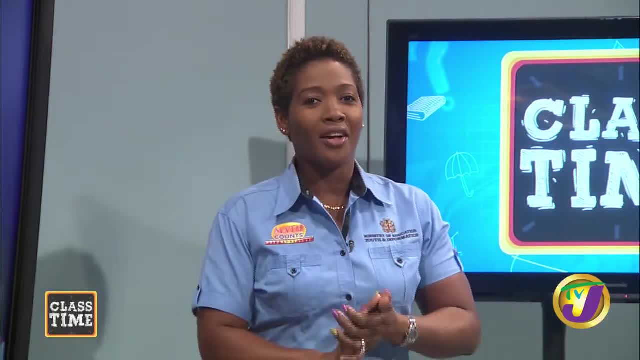 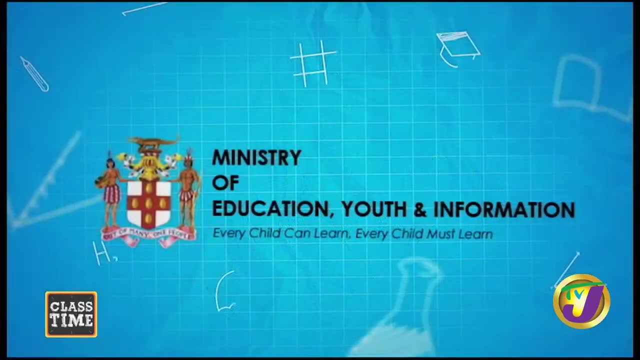 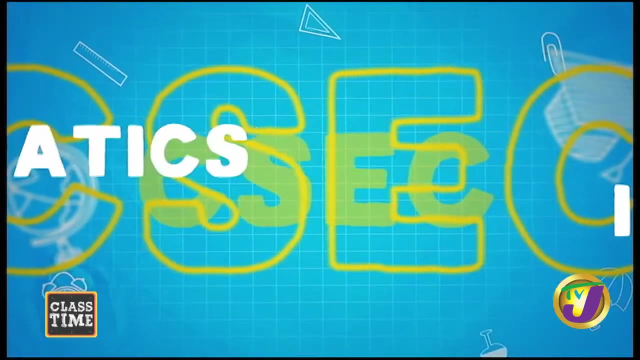 All right, Awesome stuff. Okay, We are going to take a quick break. We'll be right back with more mathematics. I'll be right back. All right, Take care, Take care, Bye-bye, Bye-bye, Have a great day. 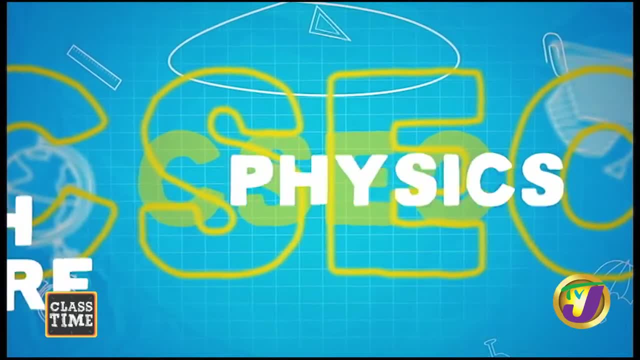 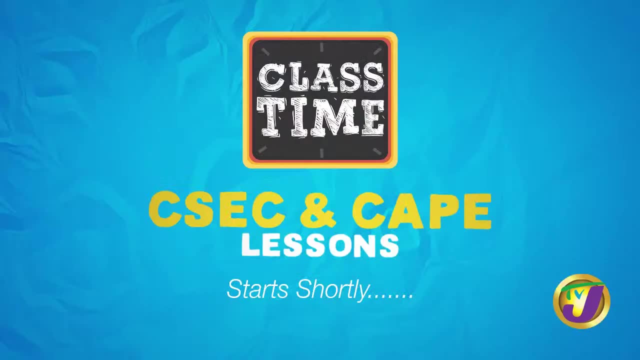 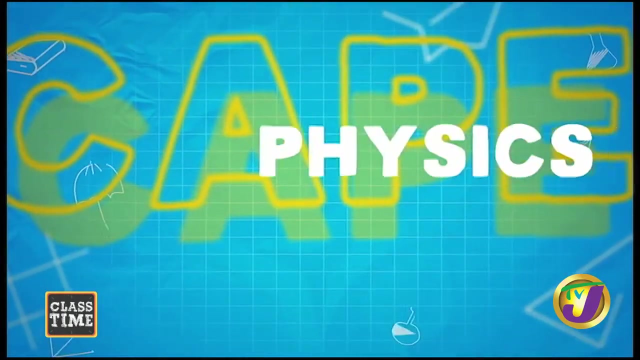 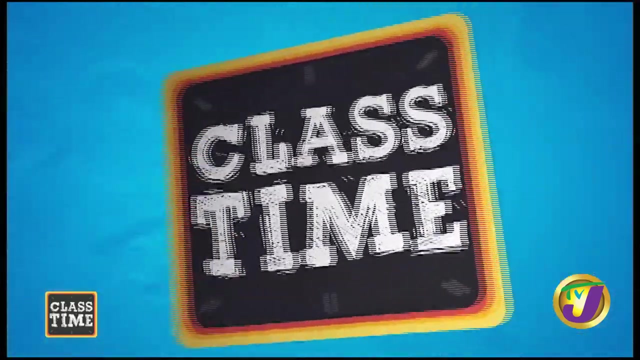 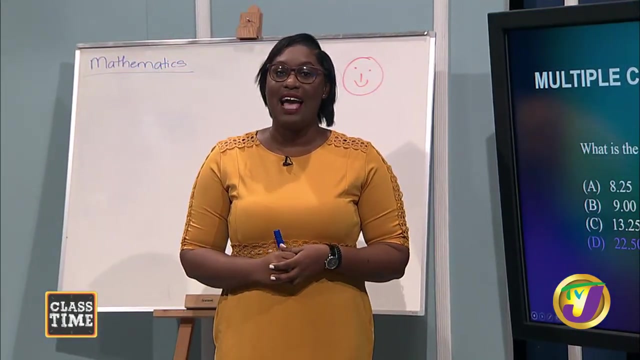 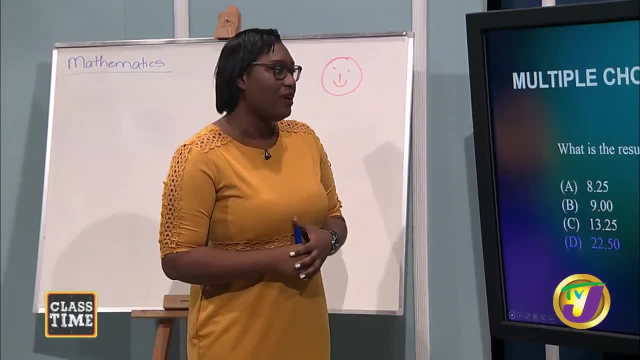 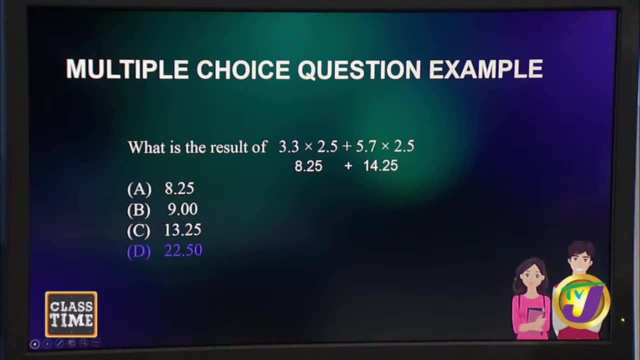 all right, so let's get back to it. so the last question we left off with was: what is the number theory of computation and what is the number theory of computation 3.3 multiply 2.5 plus 5.7 multiply 2.5, and we brought up some salient points here. we talked. 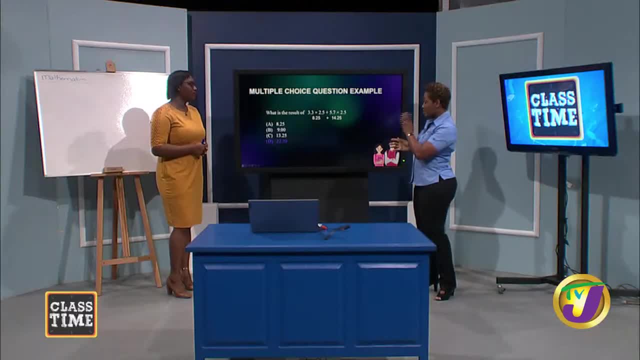 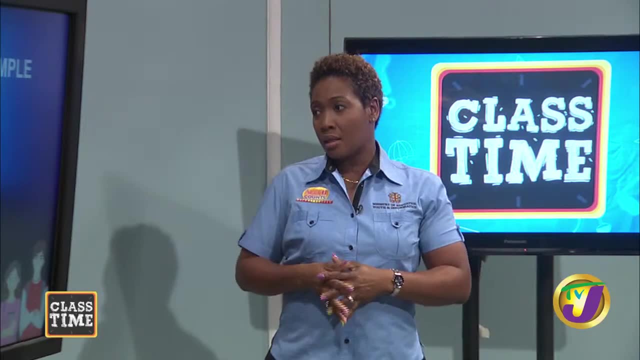 about no brackets. what else? um, there is more than one operation, so there's multiplication and addition. what do we do? first, because there's no bracket, to kind of help guide us. okay, and then we talked about order of operations. so what are you using? bum, das, pem, das, whatever the das you're? 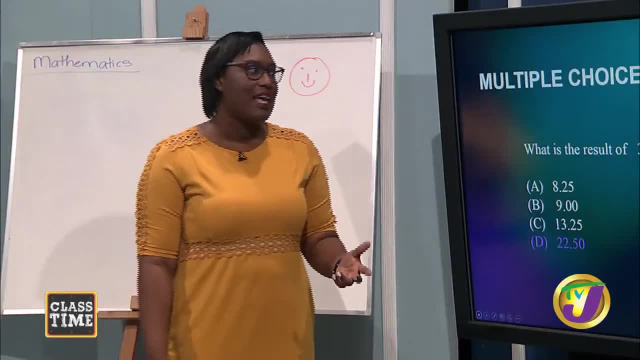 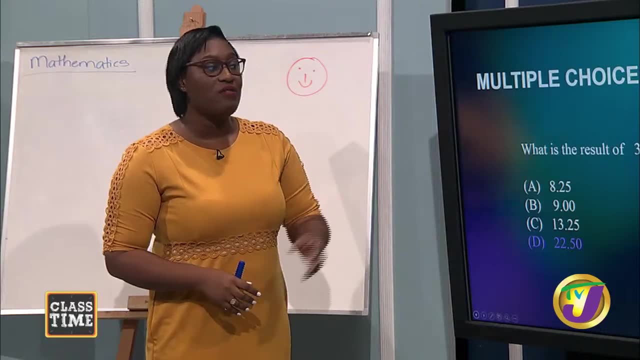 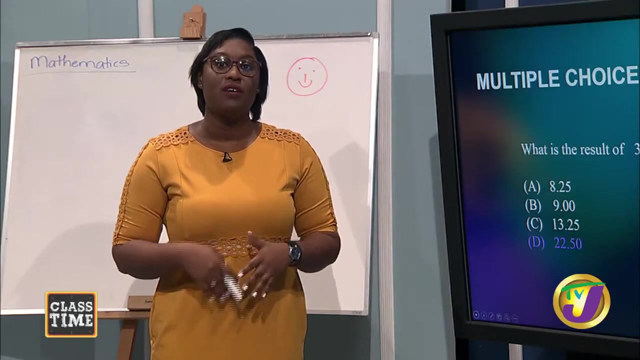 using. we're talking about order of operations and so in this case the order of operations, seems, stipulates that we first multiply. so we are going to first multiply the first two pairs, multiply the second two pairs, and we're going and we're going to find the sum of the products. 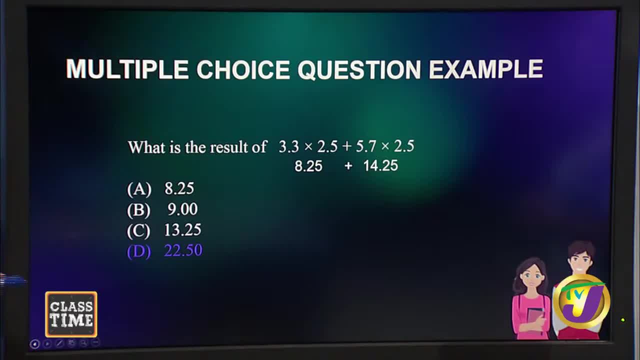 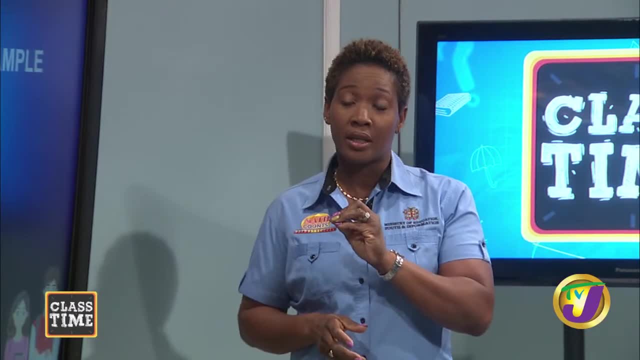 of the two, multiplication of right. so we're going to find the sum of the products. so the result of multiplying both pairs. we add them together and then you, we. you also made a very important point at the beginning of the lesson that you can eliminate some of your distractors by you know. 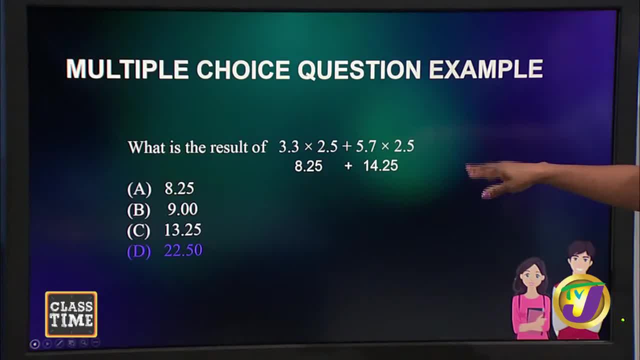 observing what you're doing. and then you- you also made a very important point at the beginning of the lesson- that you can eliminate some of your distractors by, you know, observing what is there and what is there, and we realize that eight and twenty five hundredths plus fourteen and twenty, 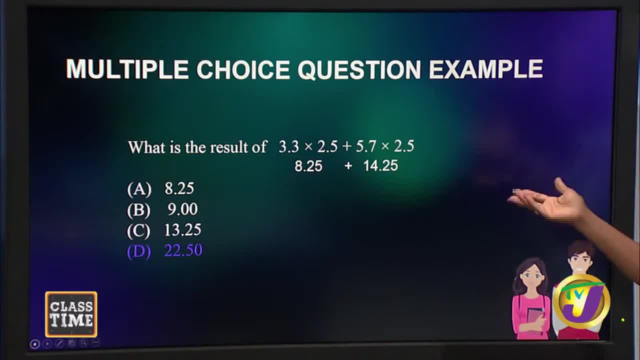 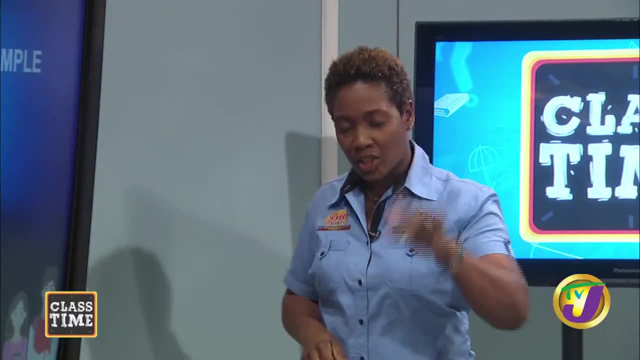 five hundred would give us five tens or fifty hundredths. so, right away, there is only one option. we just want to ensure that the fourteen and eight adds up to 22.. so, right away, you didn't have to check for the others. don't tell them not to check this. tell them to check, check, check, check, check, please. 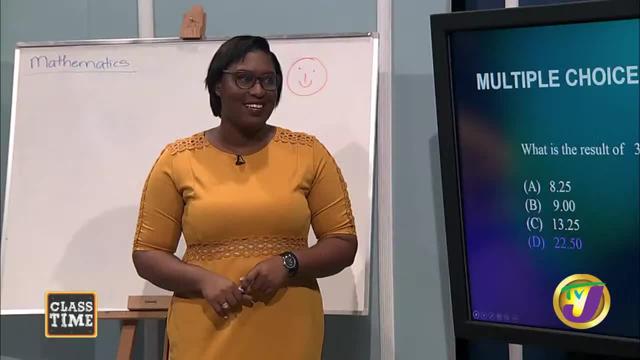 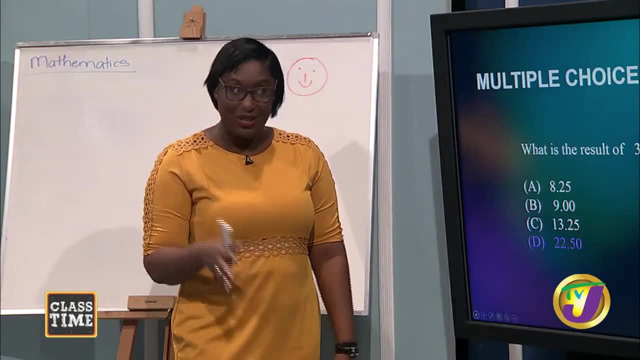 yeah, ensure that the answer is correct. yes, man, remember, that's what i mean. oh, okay, guys, remember, relax, relax. so after we read and all of these things that we eliminate, we x out, we're still like a check, check, okay, all right. so we checked and we found out that that was not relaxed to sleep. 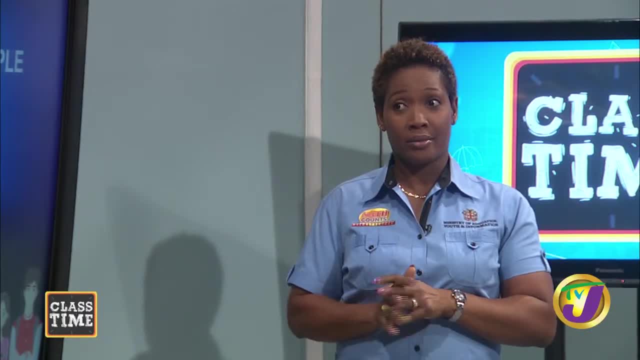 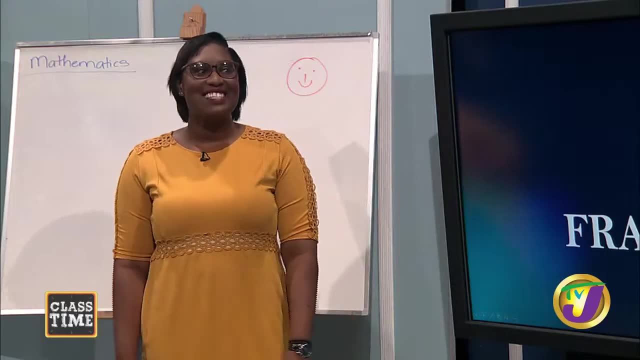 though, you know, because you don't want the dip, them can relax to sleep and then the exam not doing it, so you can't take a nap. no miss, come, come, come. let's set to the next question. we don't want enough now. come, come, come. all right, so exciting times. this is a problematic area for a lot of. 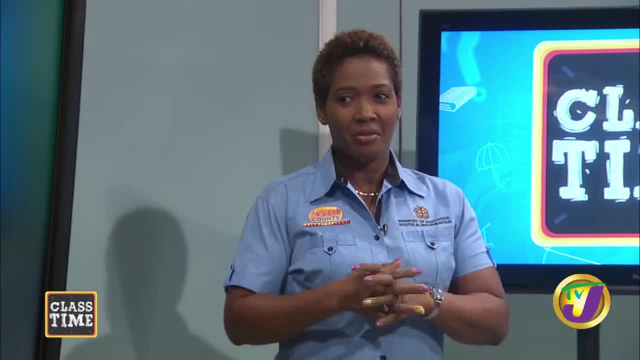 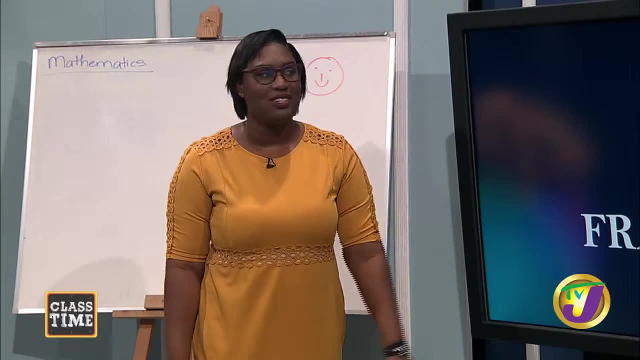 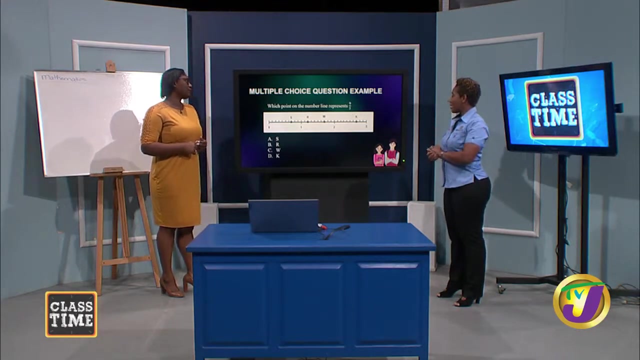 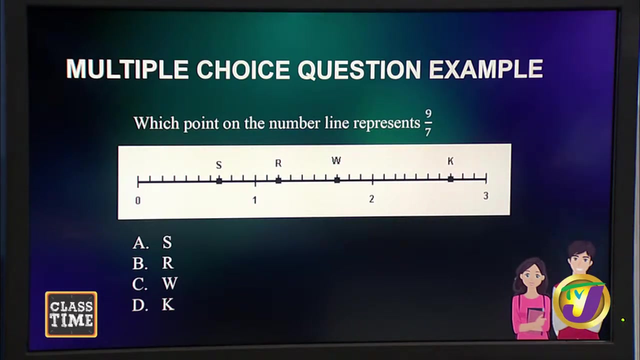 students, fractions, oh yeah, fractions, students, everybody knows. okay, all right. so, adults, children, babies, everybody. so everybody has a problem with fractions. so let's get into fractions some more, all right. so which point on the number line represents nine sevenths? nine sevenths, all right. so, right there, that's an improper fraction. therefore, we are talking about 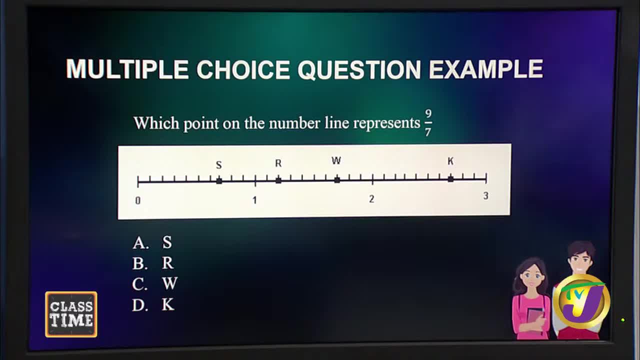 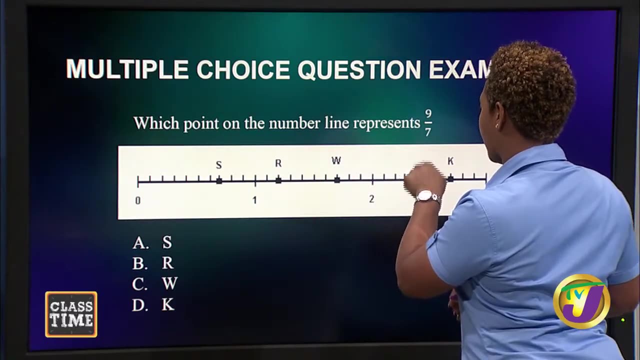 one and something. all right, so that's one. how many sevens can i get from nine? one and two is left, so i'm going to have to literally count up how much parts. one, two, three, four, five, six, seven, eight, nine, ten look like that, divided in ten, why you want to give me that. all right, two sevenths so. 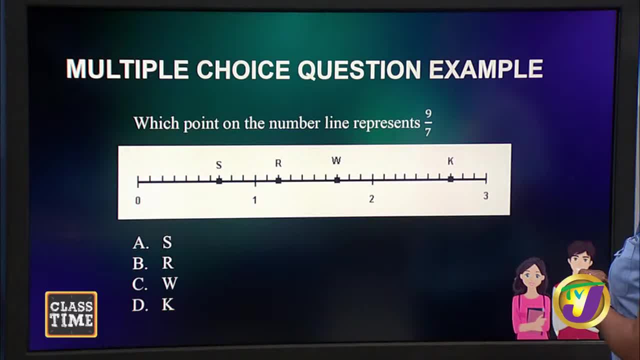 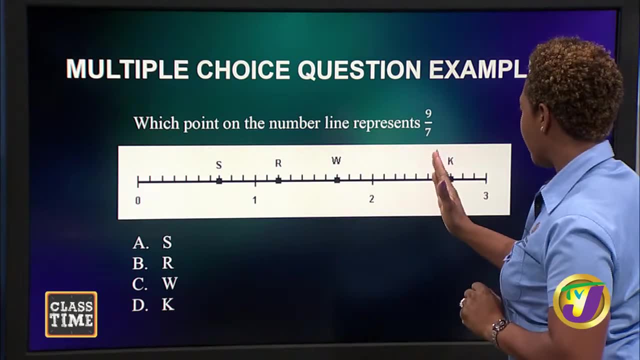 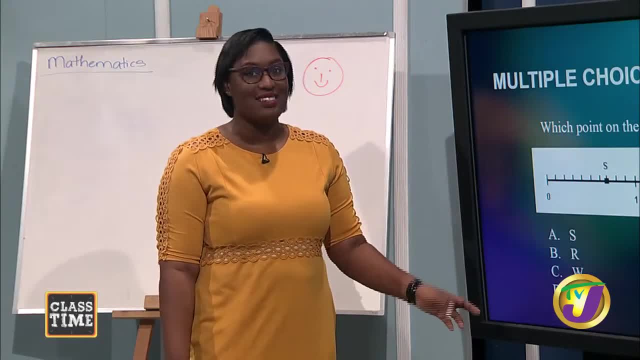 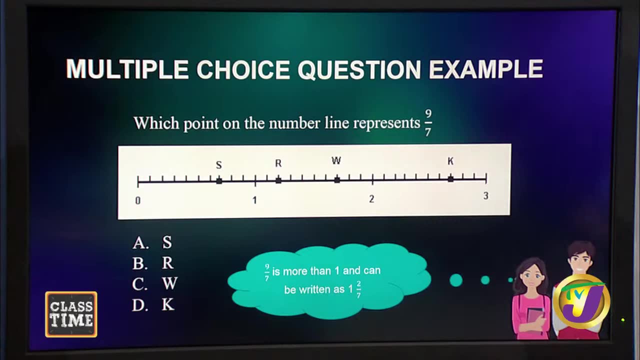 okay, it's unconfident, though. yeah, all right. okay, i've got this all right. so again, you converted and let's see. all right, oh, our friends are talking to us, so jenny and jack also want to get in on the mix and they're saying that you're correct. so it is one and two. sevenths got this right, so we know. 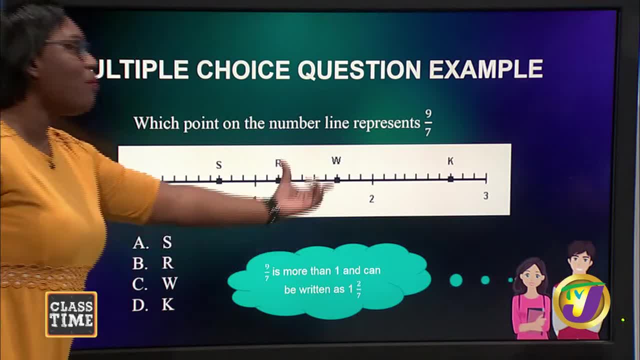 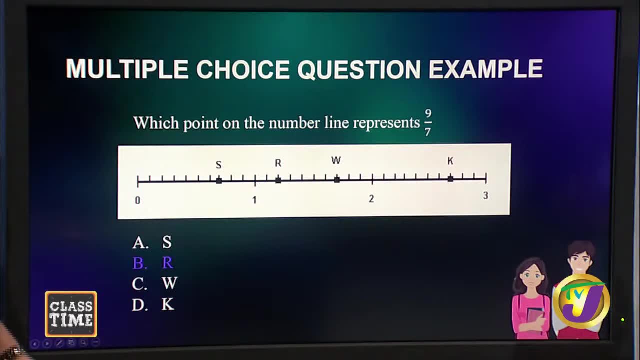 that we are not looking in the first partition, but we're somewhere in the second partition. that's good. good, all right. them don't talk. yes, yes, okay, and they have said that you are indeed correct. the answer is r. no, don't be daunted by the fact that you're seeing a number line. 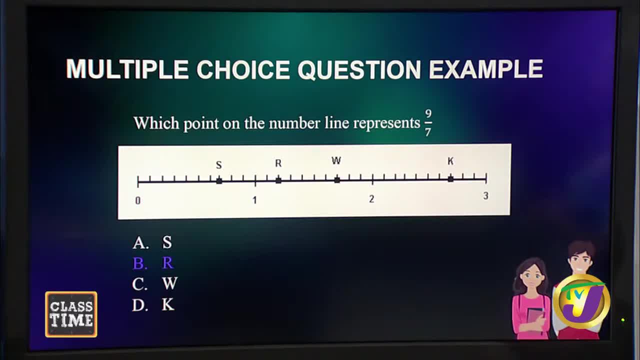 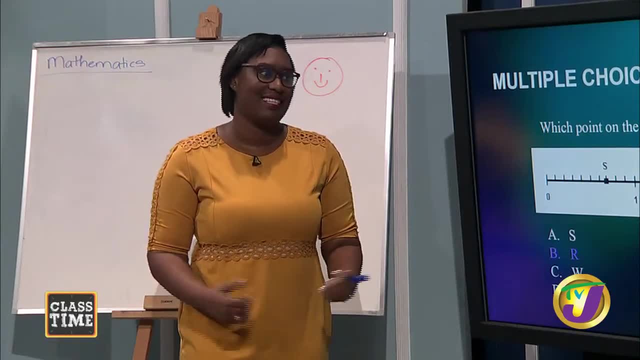 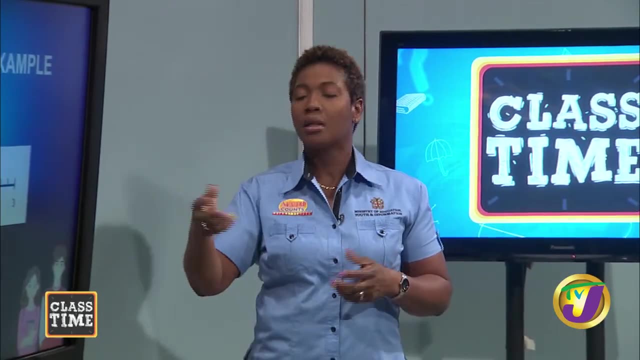 that not only has numbers but letters. oh yeah, so you might see this on the exam. lord of mercies, what they come with, no, why them come with this, relax. but it's important to benchmark, because when we converted the nine sevens to what, what is it again a mixed number. yes, one and two sevenths. 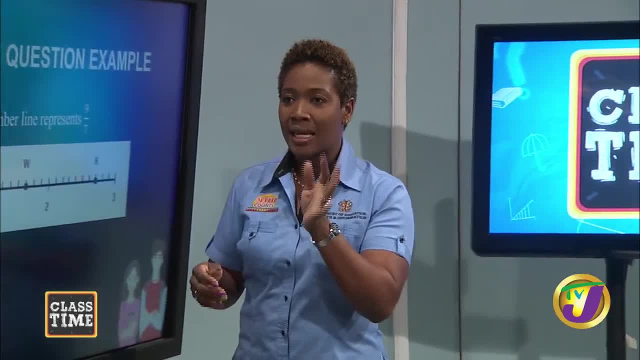 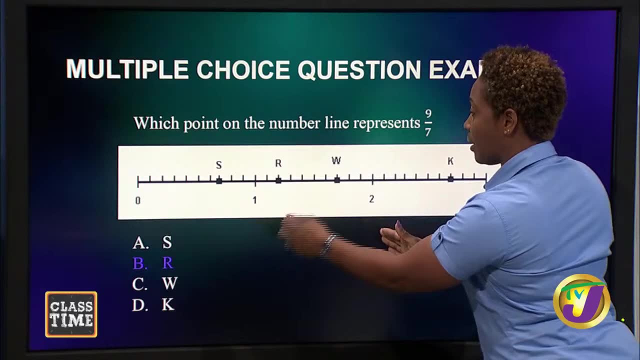 you have to be able to understand that two sevens isn't halfway, so it's less than half. so right away, you can look at the two options you have within this section. and this is more. w is more than half right, it's more than half so. 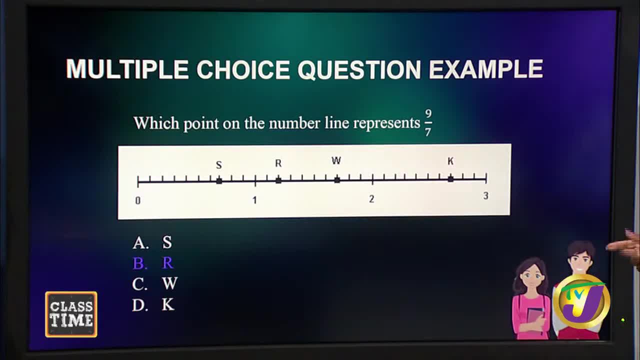 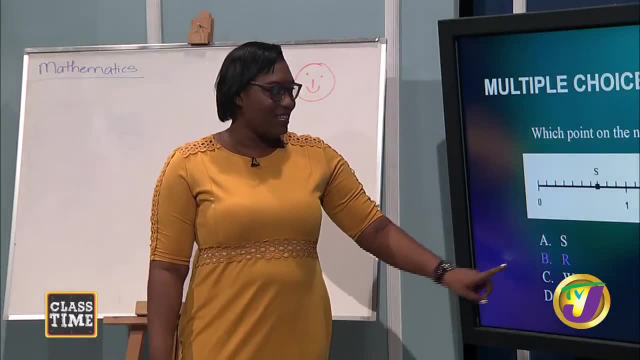 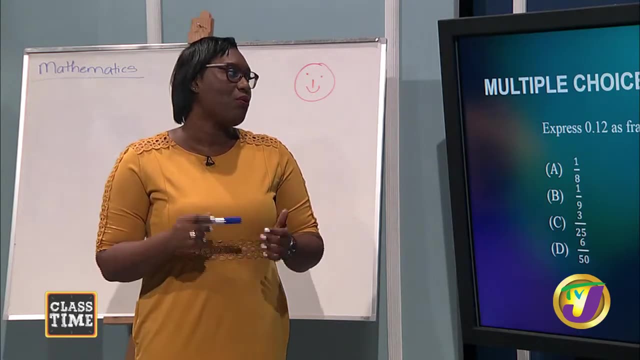 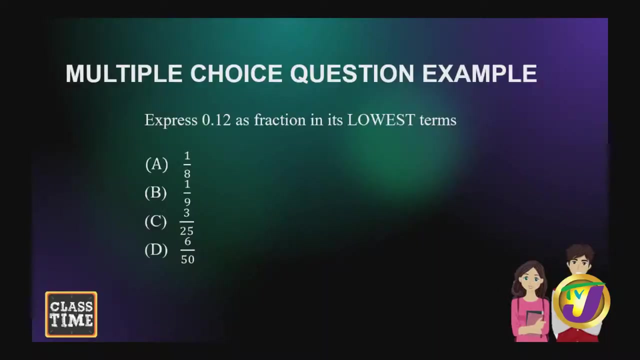 so w is closer to two most right. so we know that, you know, because that's two, yeah, man, all right, good, good, next question next. you, you just get so excited about the fractions, okay, so now we're going to take a look for one way to start x chapter one. one x zero, one x two. you see that. 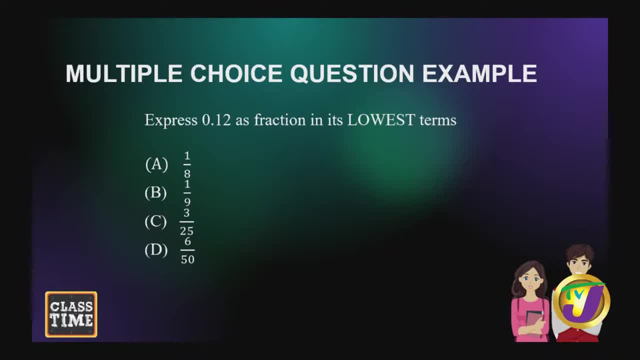 we have in this. this is a fact. two is female and we have a female and a female in the last class. so if we take one of them and we have um one and one as well as one as one, so here we have over one and two. so am i with you guys? yes, my name is. am i the only one who can express? zero point one, two as a fraction in its lowest terms. zero point one, two as a fraction in its lowest terms. what we mean- i see a decimal on the screen- are we? am i the only one who is a fraction? come out of this. but, guys, we know a few things. we know that another way of looking at zero point one, two is saying twelve hundreds. that's right, twelve hundreds. 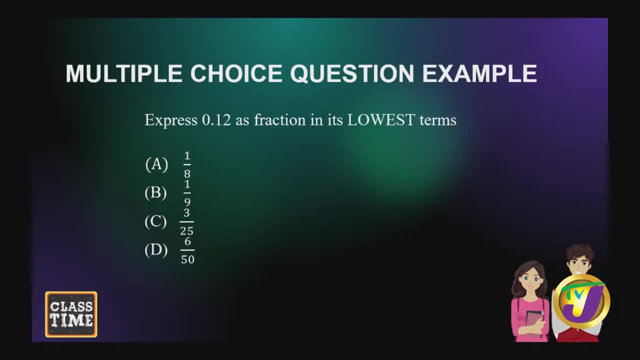 It's a big fraction. Eh, don't it. But we can write it, don't it? Of course we can. So that's the same as saying 12 divide 100, don't it? Yeah, 1,200,. so 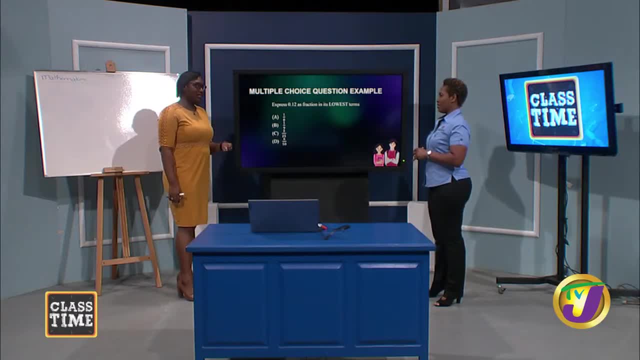 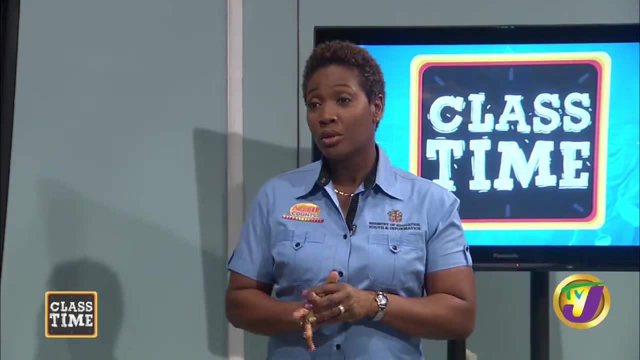 You can't simplify that though, Maybe. maybe because 12 and 100, they must have some common factors. Yes, they do. They have 4,, they have 2,. yes, Those are enough factors, though. all right. 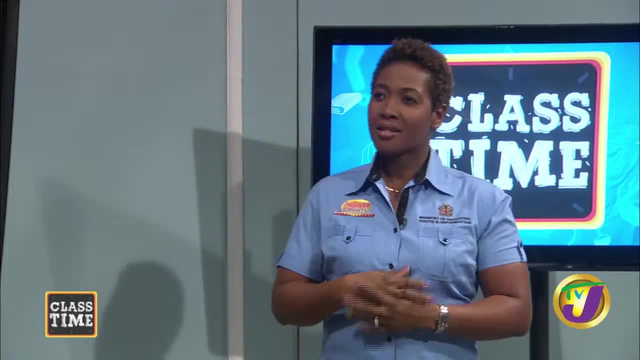 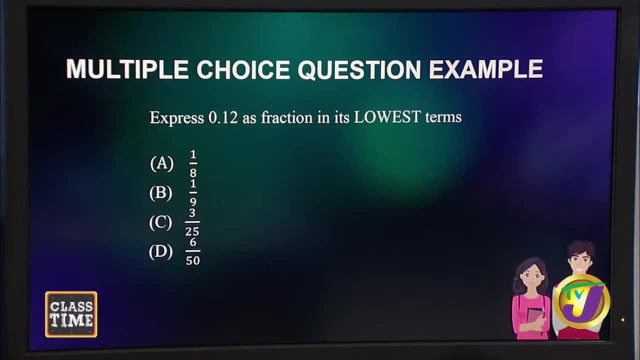 All right, we can use a 4.. So in this case, this is not. you just brought up a very important point. In this case, we need to look for the highest common factor, So we need the largest number that's common to both numbers. 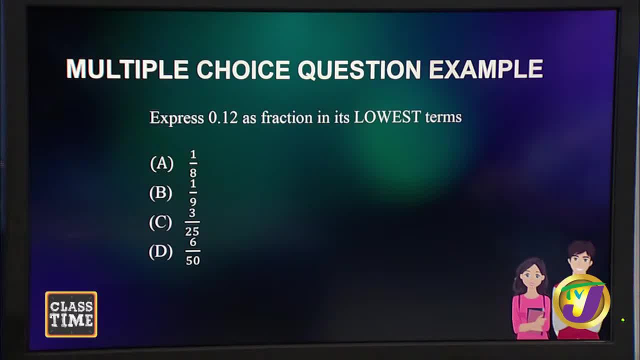 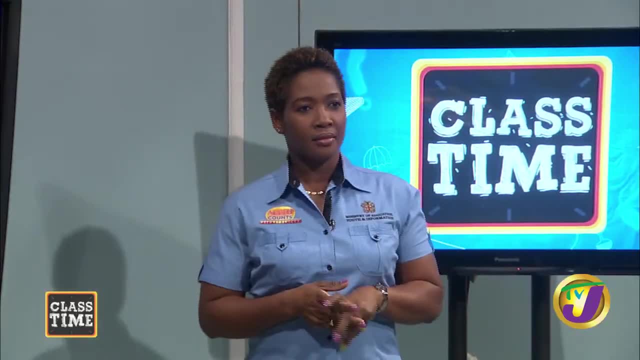 that when we divide them, we have no remainder, Because I know you don't ask me, no, you don't tell me, but you hear the word factors and a lot of you are scratching your brain. Factors, where that come from again, and I get confused. 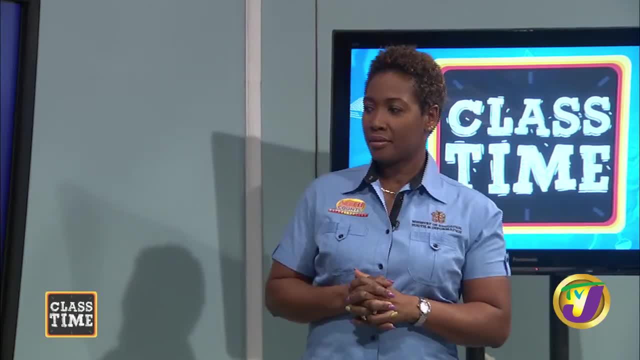 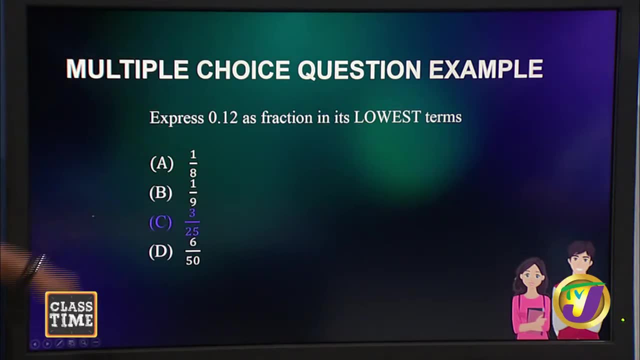 You can divide it in the number, man, and nothing is left, All right, So I keep on forgetting about Jenny and Jack. They're talking to us, all right, And so they're verifying that. indeed, our answer is C. 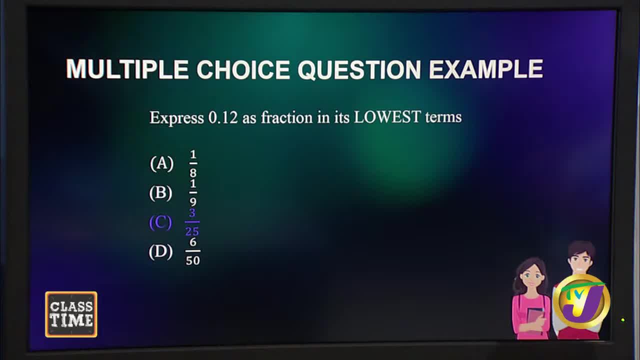 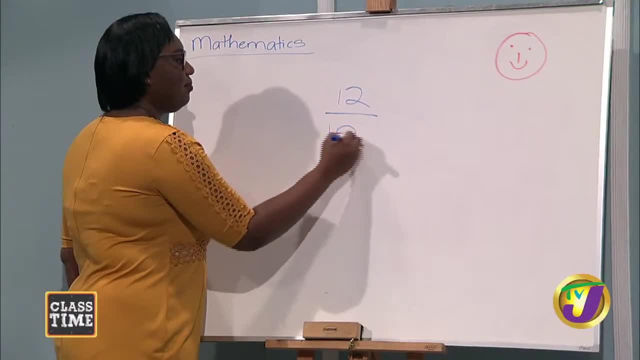 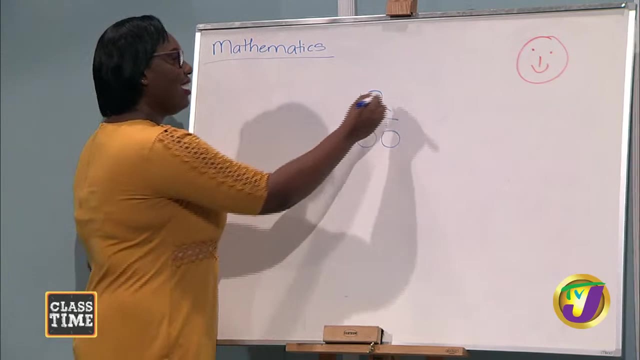 So let's show them how we got it to C though, So 1,200, with the largest factor being 4.. Look at that 1,200.. Look at the right picture on the board Right. so 4 divided into 12 goes 3 times. 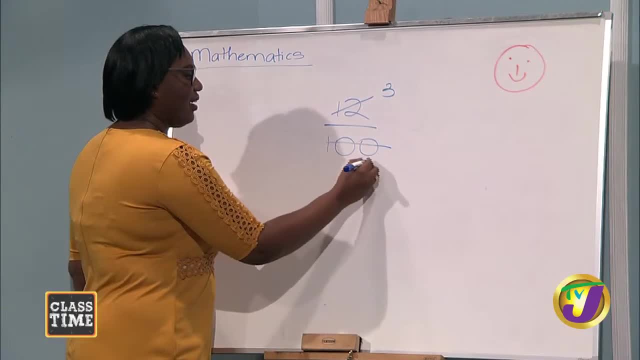 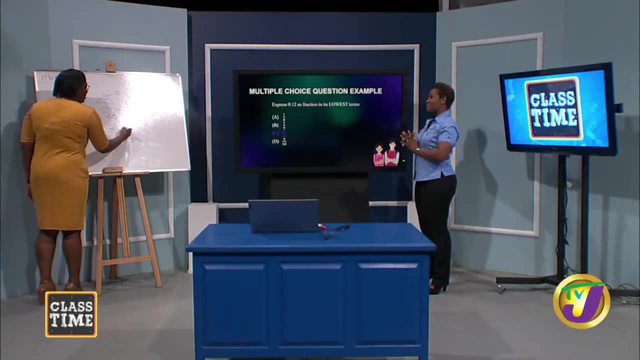 And then 4 into 100 goes 25 times. So look at that: Simplifying that fraction gives us 3, twenty-fifths. So again, let me just write it out. There's another way, because you know, Miss just said 4.. 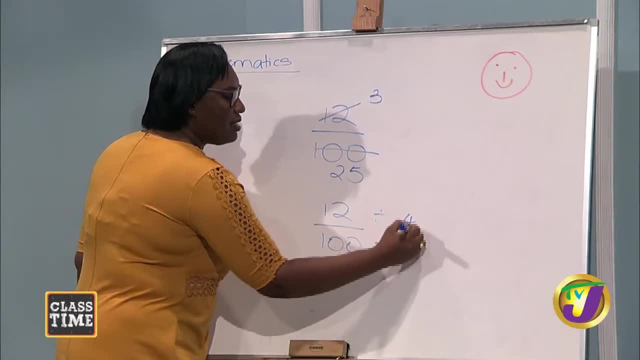 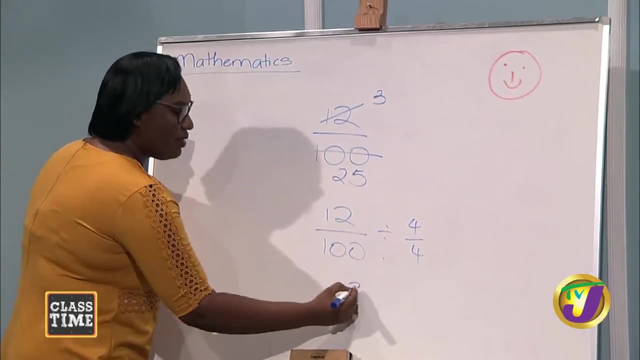 So it means that we're dividing both numerator and denominator by 4, right? So we're dividing both numerator and denominator by 4, so we're left with 3 twenty-fifths, 3 twenty-fifths. Yeah, yeah, there we go. 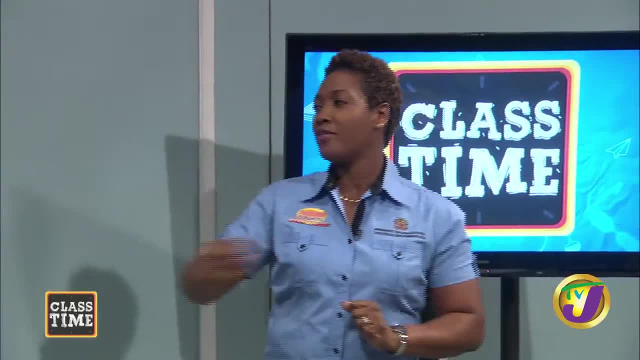 Okay, All right. So 1,200 is equivalent to 3, twenty-fifths, and it's in its lowest term. Oh, thank you. And then again, guys, you can always check to make sure that your division is correct. 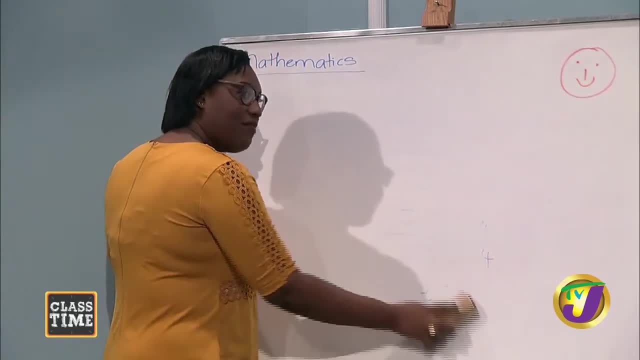 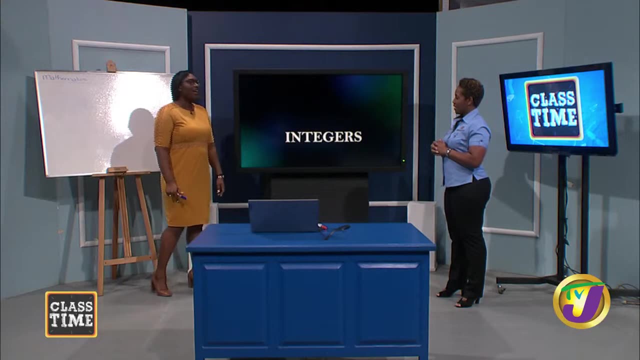 because sometimes you're dividing 2 and 25, because you know 5 and 4, sometimes you divide it, you get 20.. Check that, It's true. it's true. Check it, All right. So integers. 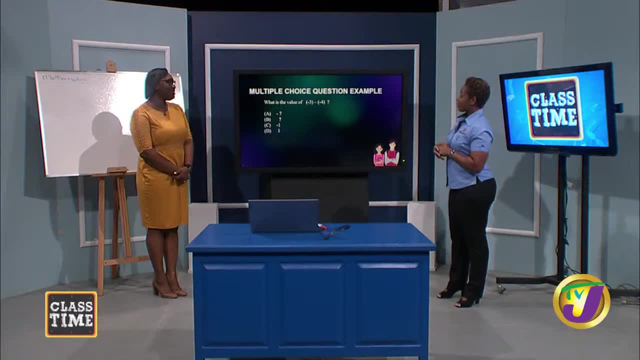 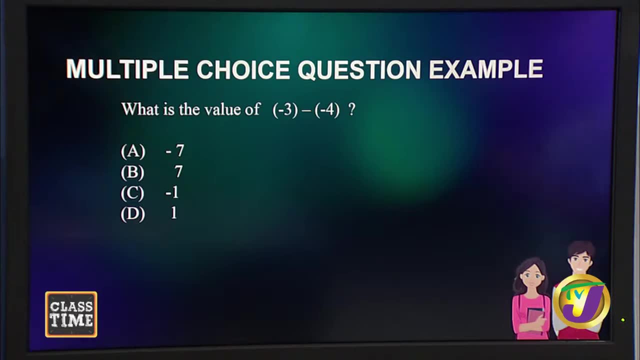 Okay, Fun times. Ooh, fun fun times. That looks great. Okay, This is another scary section for students. Oh, yes, When it comes down to integers, negative and positive numbers, Directed numbers, really and truly Really. 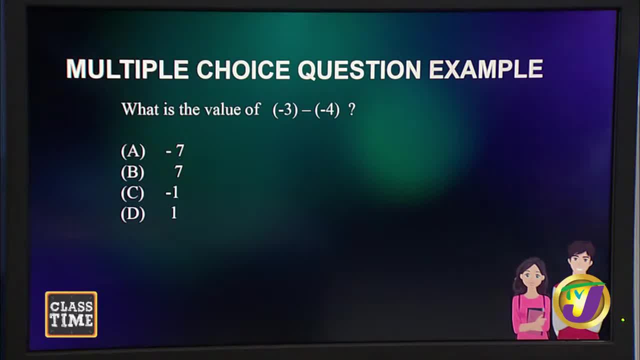 Really Don't want to look at it. All right, So what is the value of negative 3 subtract negative 4?? All right, Let's find the value. All right. So we have negative 3 subtracting negative 4.. 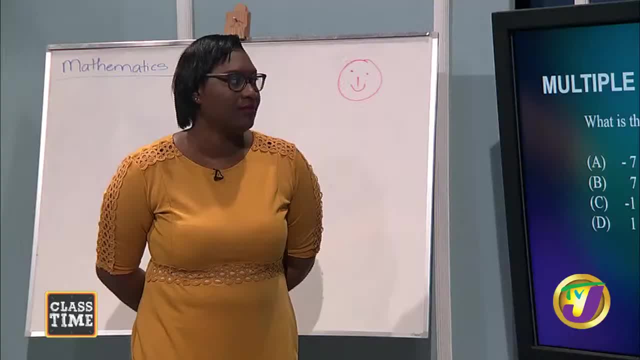 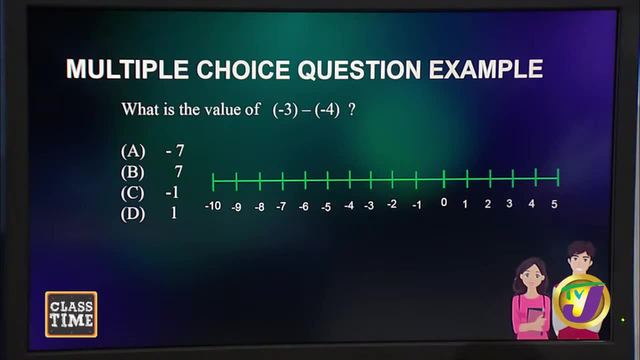 So that means we don't have nothing positive there? No, All right, We can put this on a number line, All right. So here we have our number line and let's locate. So we're starting at Negative 3.. 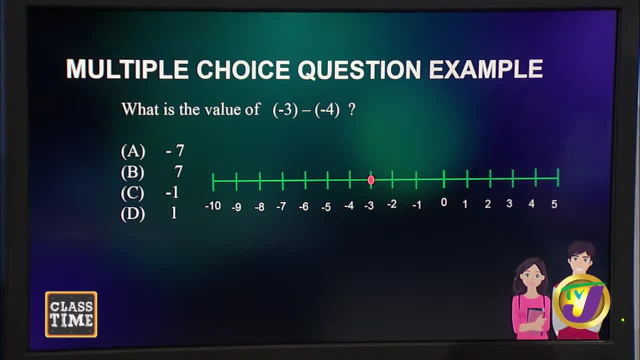 All right, Right, And I am subtracting negative. 4.. Mm-hmm, All right, So that means I am moving to the. what is this Left? Okay, Okay, Mm-hmm, Okay, Mm-hmm. 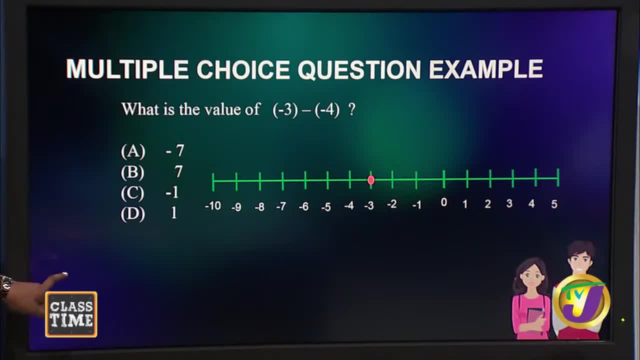 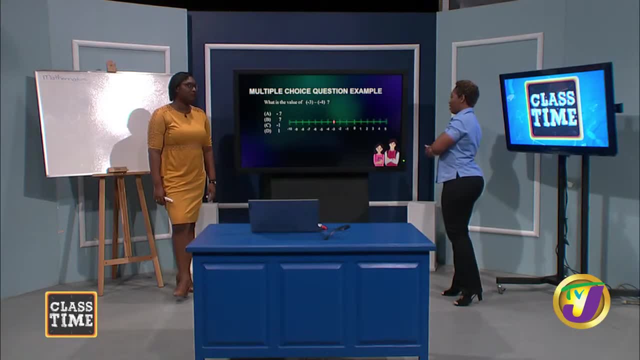 But because it's opposite of the opposite, we're actually going to be moving to the right. Awesome, Because I'm subtracting negative Mm-hmm, All right, So let's see what that looks like. So I'm actually moving 4 units to my left. 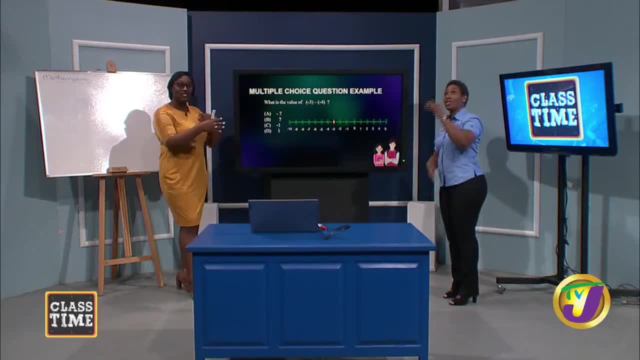 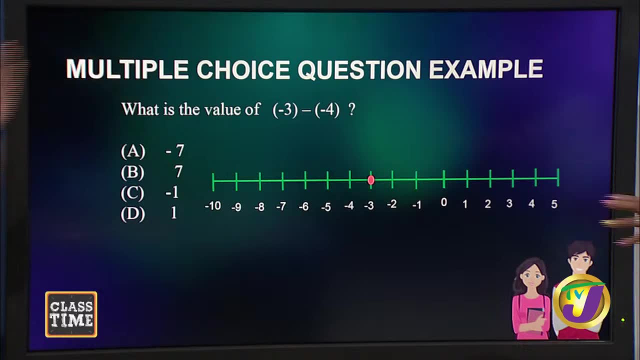 Well, my left, my left, your right, It depends on how you turn guys, That is relative, Let's just face it. so we stay on the same side, Okay, All right. So moving to the right guys, There you go. 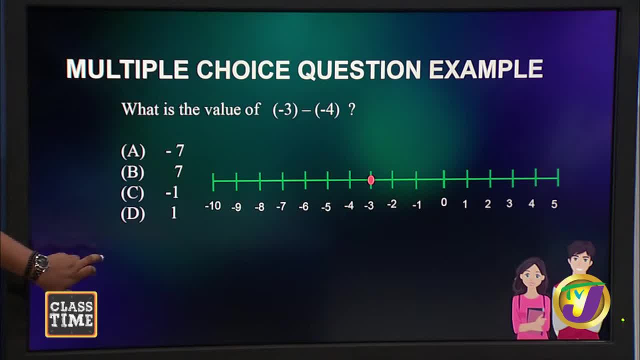 To the right, to the right. Moving to the right, Beyonce said to the left, We're going to the right, That's right. So we're moving to the right: 4 units and our result is going to be 1.. 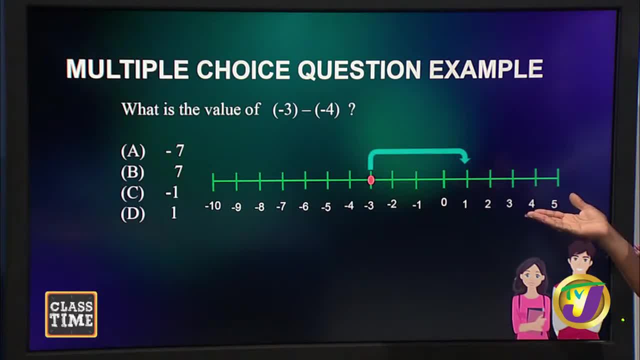 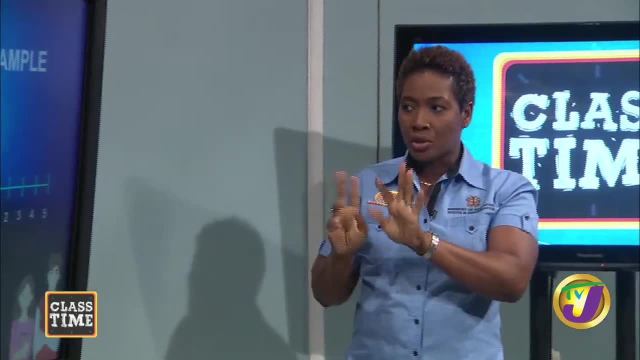 So what happened here is that the negative changed the direction in which we're going, Mm-hmm, So it became negative 3 plus 4.. Yes, Okay, In essence, So those two negatives when they meet, they change the direction. 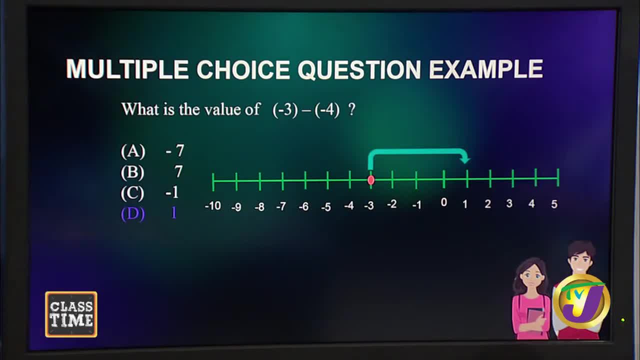 Yes, Gotcha, So we're at 1, right, Okay, Now. okay, we've been doing a lot of talking. I hope you guys at home trying the questions, Mm-hmm, I hope so you know. 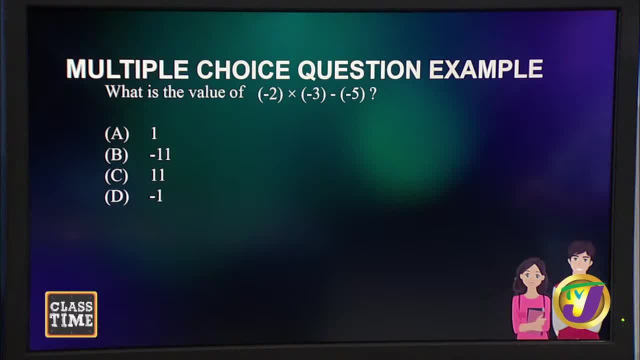 All right. So what is the value of negative 2 multiplied by, really by negative 3, subtract negative 5?? Okay, Well, right away, I know that It's some direction changing. right, You're the negative 5.. 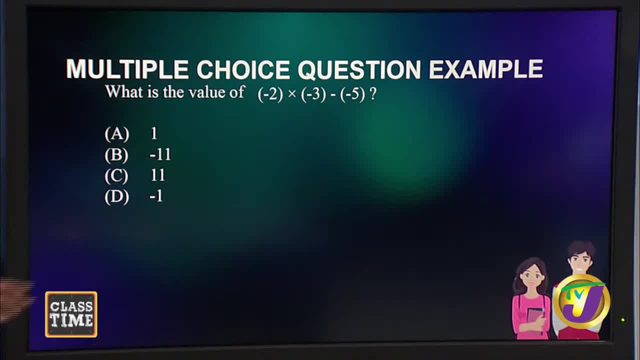 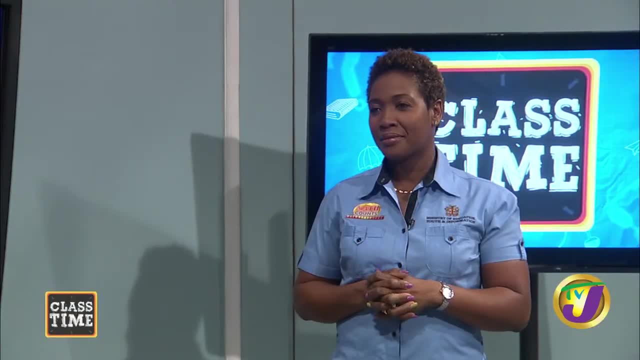 All right, No So um, This is exciting, This is not exciting. I'm excited, You're not excited, You guys are excited. I'm sure they're not excited to see all those negatives on the board. Is you want to feel that way? 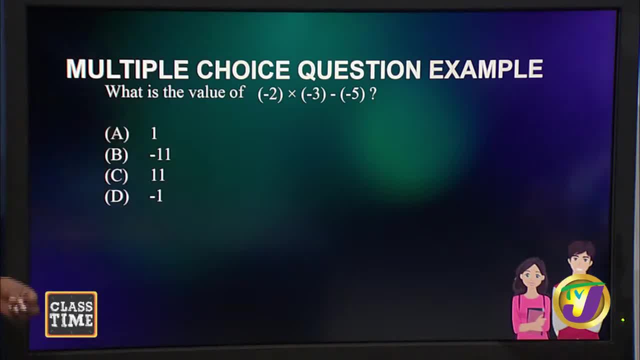 Yes, sir, Go Okay. So what does this actually mean to us? This means we have two groups of opposite negative 3, basically, Oh yeah, That's right, Yeah, So here's what we're going to do. 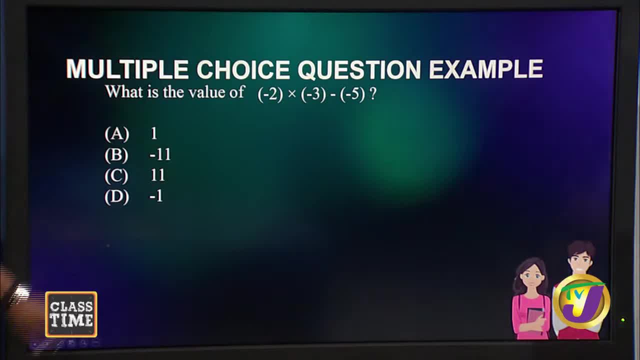 TV: magic, Magic, magic. We're going to bring in. we're going to bring in some algebra tiles. If you've never seen it before, this is what. this is what they look like, All right, So we're doing the representation of exactly what we have here. 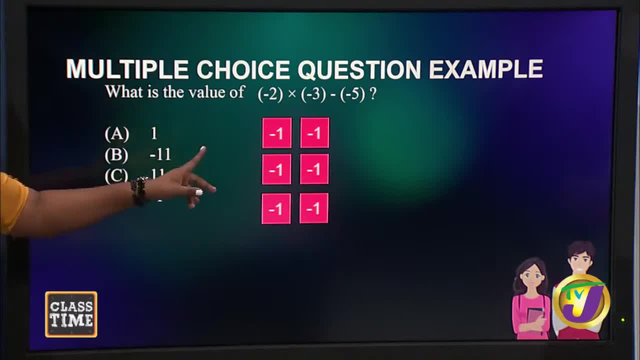 So we have to. let's start off with what we have first, Two groups of negative three. But again, because the sign is there, we know that we're going to take the opposite of these two groups of negative three. which magic, all right, TV magic, TV magic. 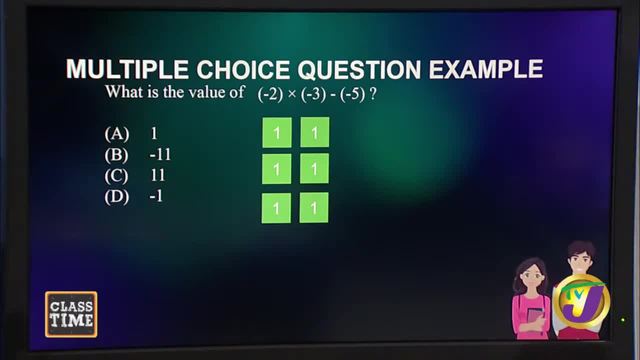 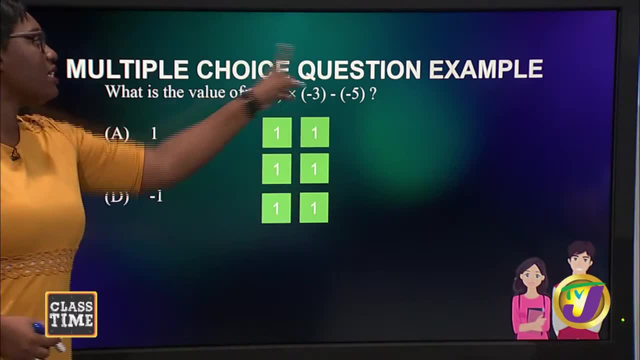 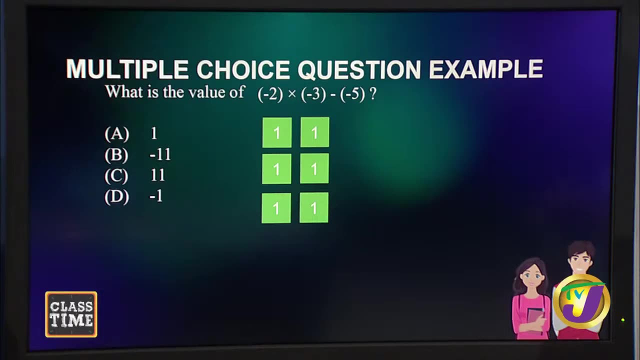 Yes, Which means we have two groups of positive, positive three, which is two groups of positive. three is the same as saying six. So we know that the result of multiplying negative to multiply negative three gives us positive six. Okay, Okay, More magic. 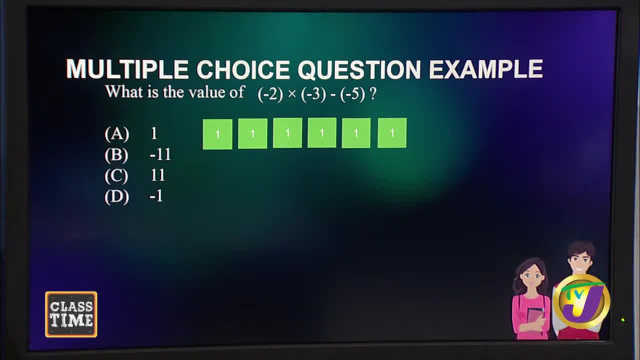 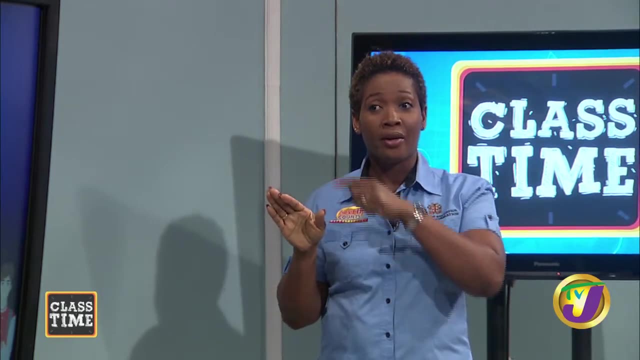 Okay, So we have the positive six. Our equation does not stop there. So now we're going to subtract negative negative five, And you just told me that that negative in front of my negative five is going to change the direction. So that means now I'm going to add five. 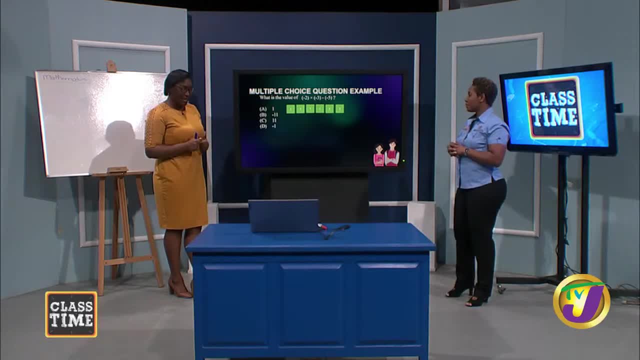 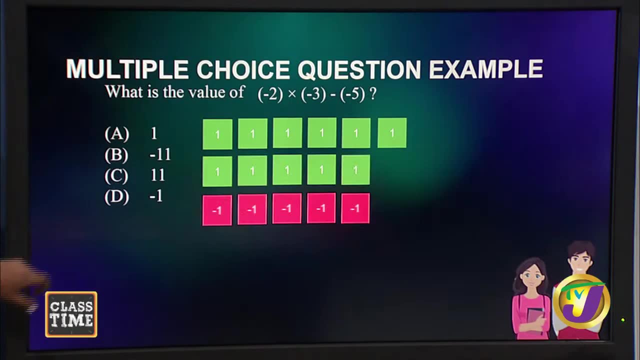 Okay, Yes, So true, true, true. But in the land of algebra tiles which we're in, we need to. as you can see here, we don't have any negative five, so we're going to introduce some zero pairs. 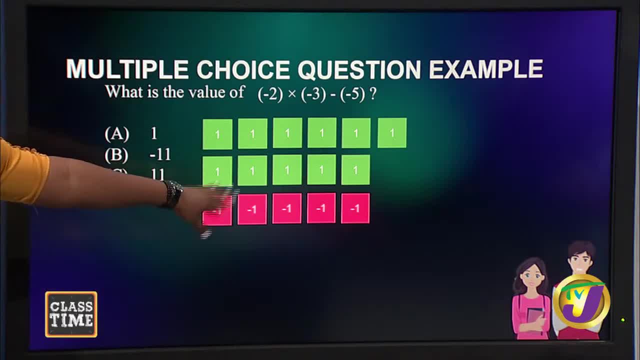 So we have five groups of zero pairs, Right. So now I can subtract my negative five. Okay, Right. So, as you rightfully said, the direction changed, And so it's simply that I'm adding five to the six, that I've got the result that I've. 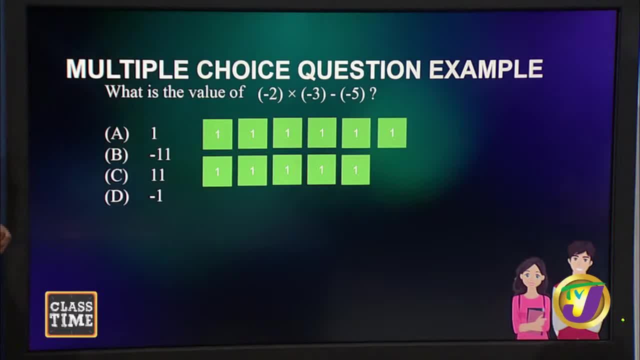 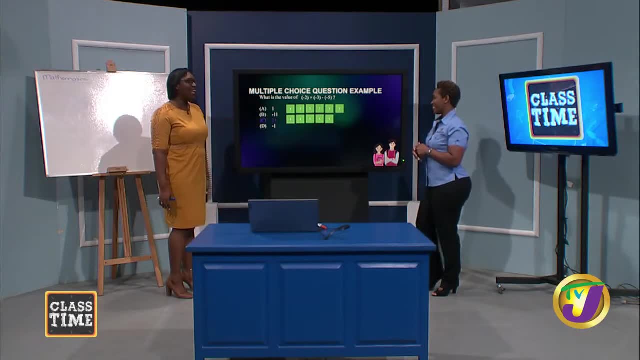 gotten. So in total, let's count it up- We have six plus five. I'm going to count it up. It's eleven. All right, It's eleven. Yeah, it's eleven. See, nice, And yeah, it's eleven. 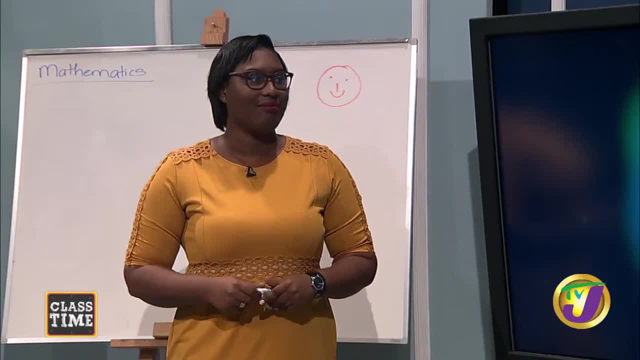 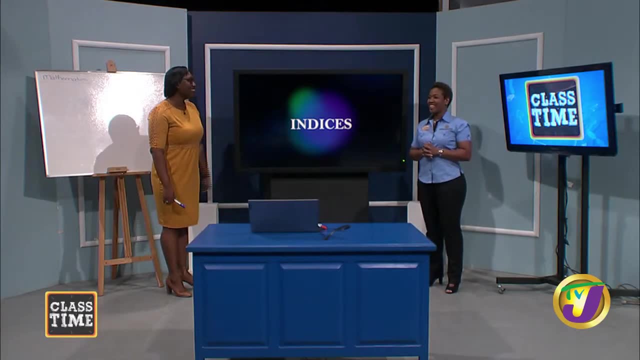 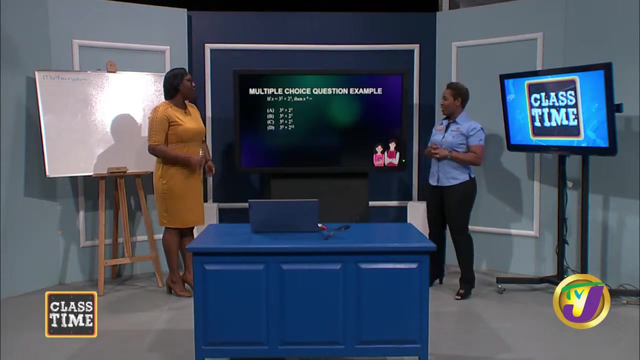 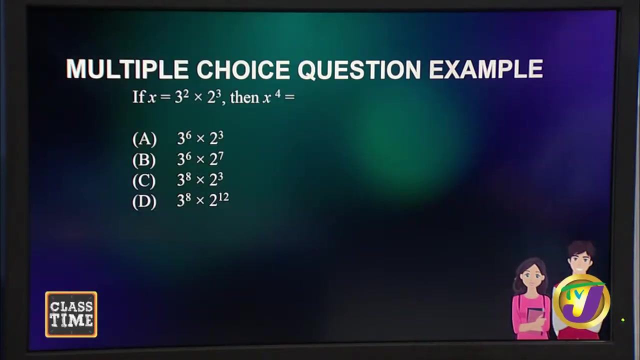 Okay, All right. Indices. hooray, If we're going too fast, you know, slow us down. I'm joking, This is like awesome. Okay, let's do. indices All right. So indices, All right. So the first question is: X equal three raised to the second, power multiplied. 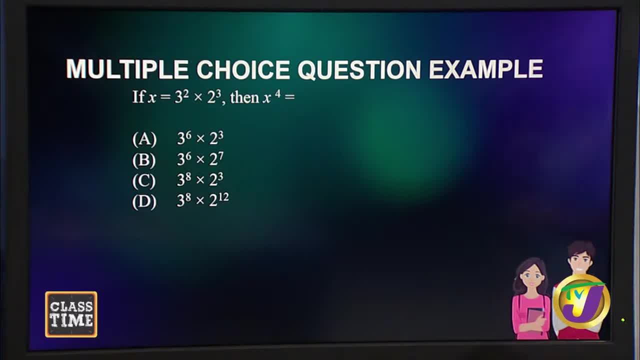 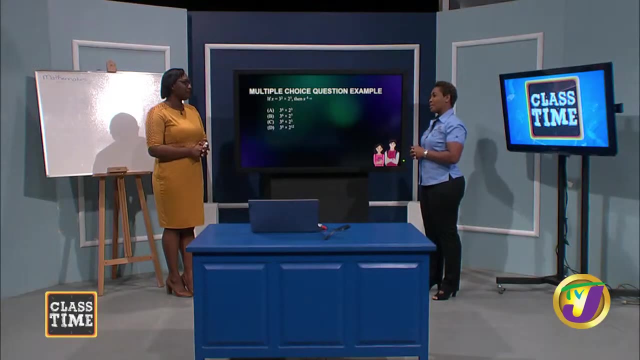 What did I just say? X equal. Did I say X equal? Okay, X equal three squared multiplied by two cubed. Then X to the fourth, power equal. Oh, Maybe you know we skipped over zero pairs a little bit fast. 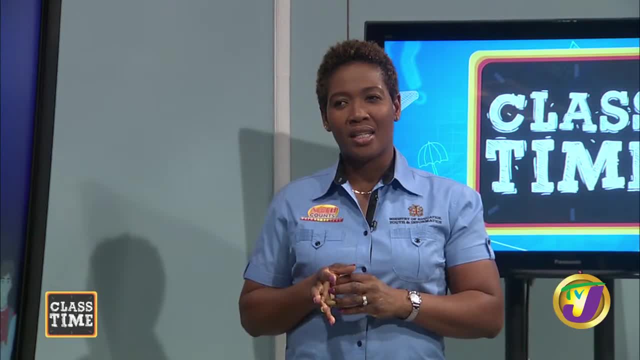 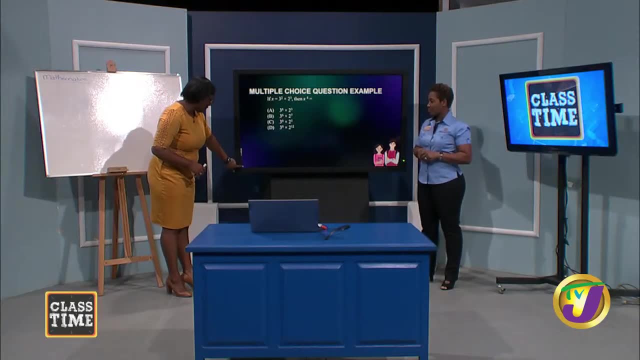 You think you think they got it out there. I think we need to explain it a little bit more so that we don't lose anyone. Let's go back to that slide just a little before we go into indices, because you know, 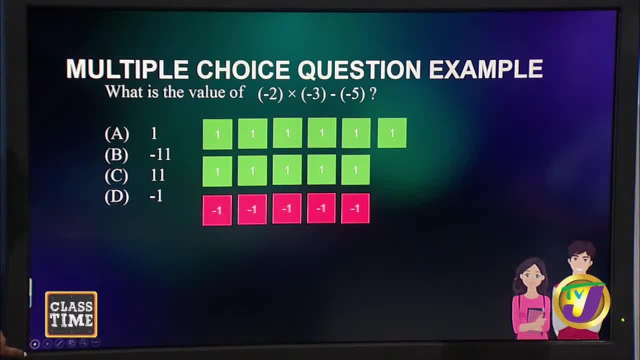 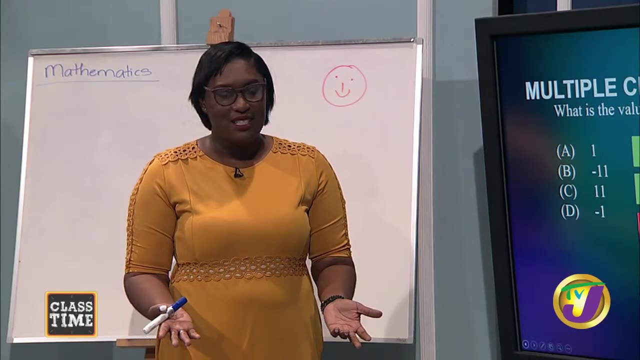 All right, So our zero pairs? Okay. So what does our zero pair tells us? What does that term mean? Zero pairs? It means, when we combine them, we get zero. Well, in essence yes, because you know, we have one subtract one. 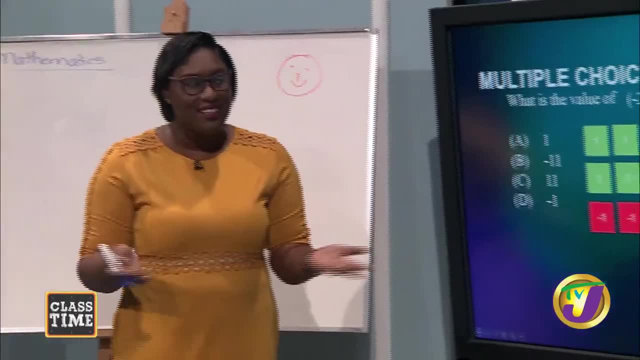 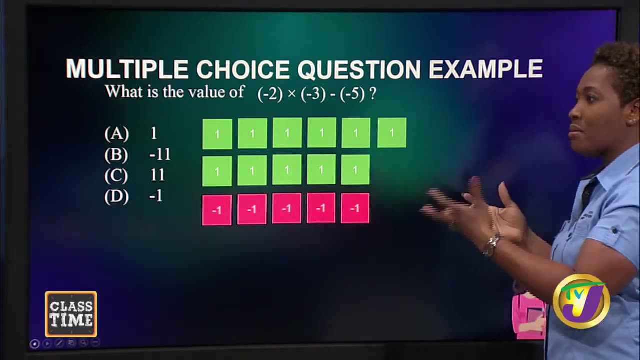 We get zero, which is really a zero pair. So if you have so, we have positive one here and we have negative one here- If we were to combine them, what it means is each of them will end up with really zero. You're saying one subtract, one zero. 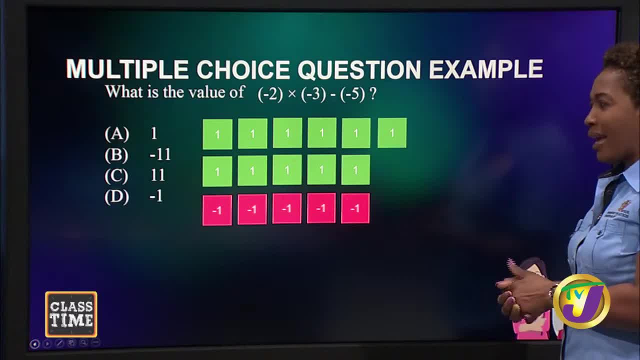 Now we know zero is an identity element, you know? Oh, yeah, Okay. So can I have any other zero pairs? So negative five and five is a zero pair. Negative seven and seven: zero pair. So once you have both the positive and the negative number, the same value. 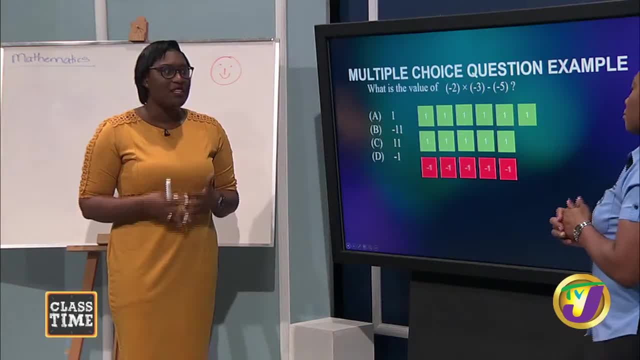 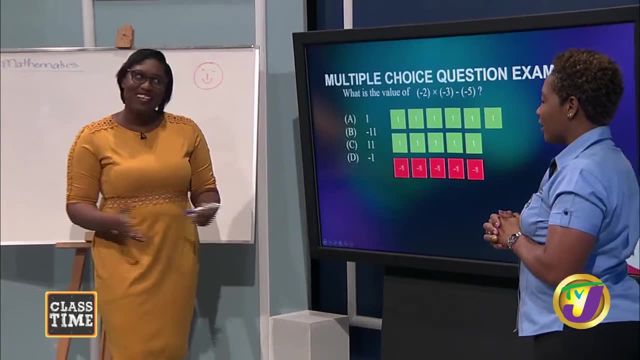 they form zero pairs and they exist all around. You know, sometimes we need to draw So they're always in. It's not like, okay, we're going to pick it up out of a pocket and they're always around. Zero is always around, you know. 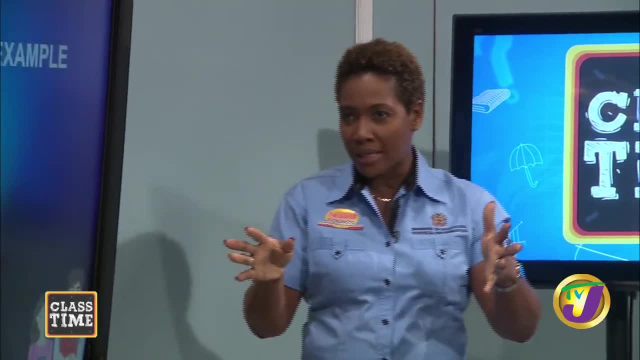 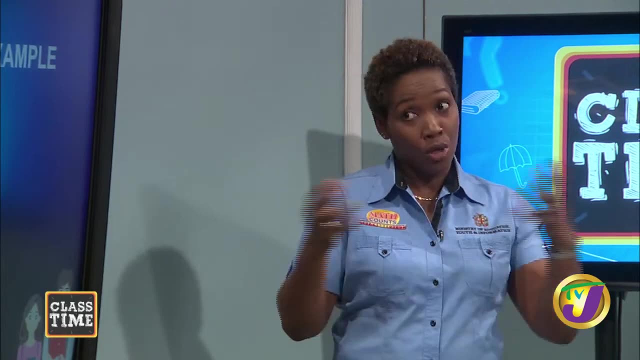 Okay, Right. So once you're looking at a number, whatever it is, and we have both the negative value of it and the positive value, they form a zero pair. Yes, Okay, So it could be 200.. It could be, Yes, Yes. 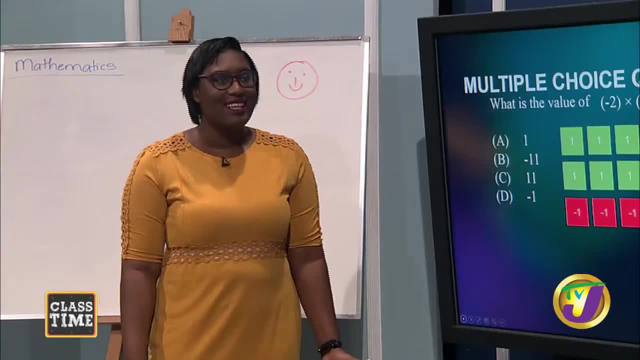 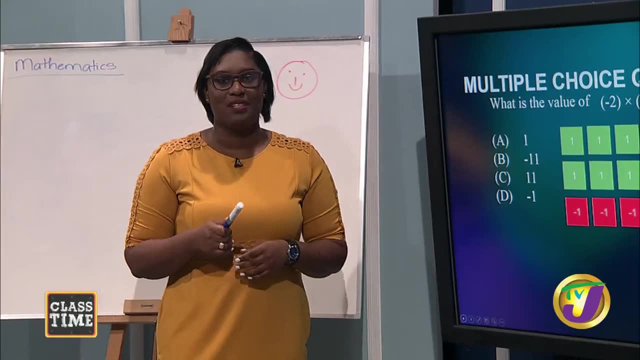 So 200 and negative 200, zero pairs. Yeah, man, Yeah, of course. So again, they're always around guys, They're always around Everybody get it. Yeah, man, We talk about TV magic, but it really wasn't really so much magic. 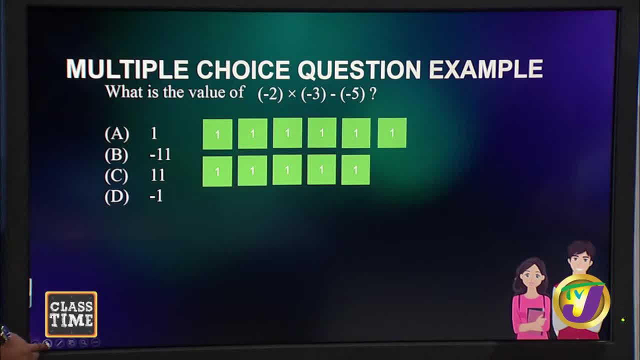 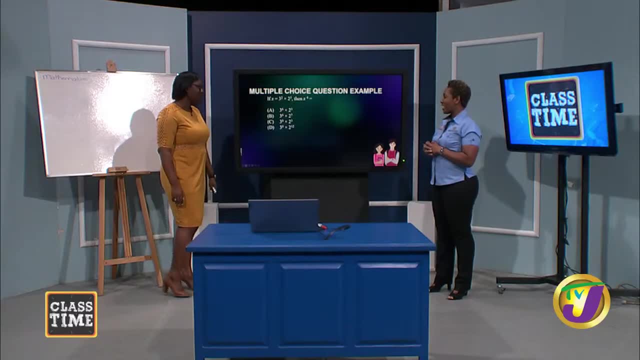 It was math magic, Right, Okay, Okay, Okay, All right, All right. So we're back at indices. Lovely topic again: Exciting times. Okay, maybe not dance. I don't know why you're dancing for this topic. 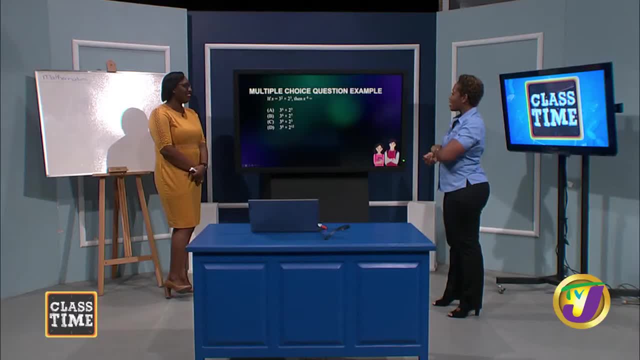 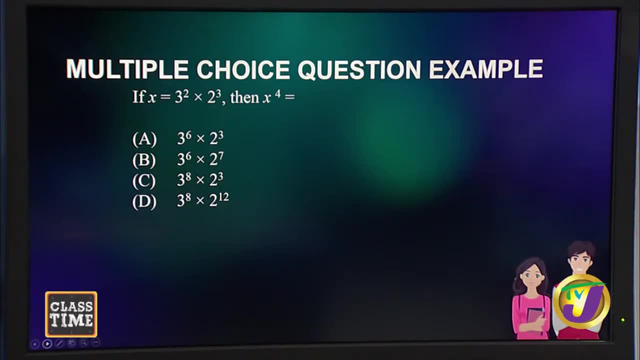 I know these kids out there are like: really All right, So X. So we have a problem. We have a math sentence there where X, if X is equal to three squared multiplied by two cubed, then X to the fourth power is, I don't know. 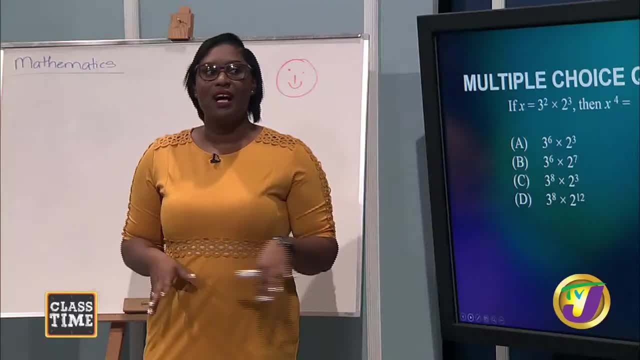 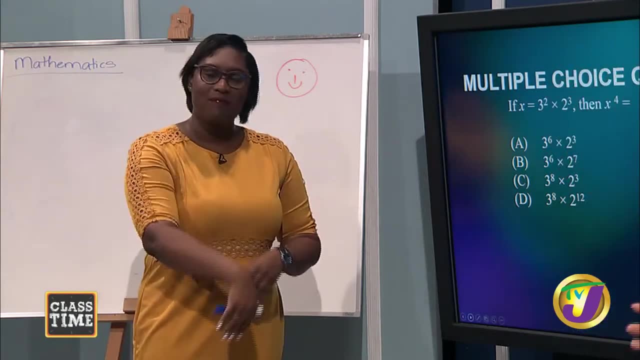 Okay, So indices. Now let's go back into our memory box and let's just remember some of the laws of indices. you know those laws of indices that you did throw away. Come back for them Right. So now it is okay. 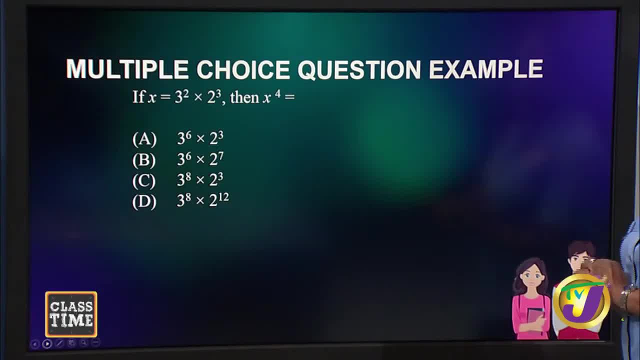 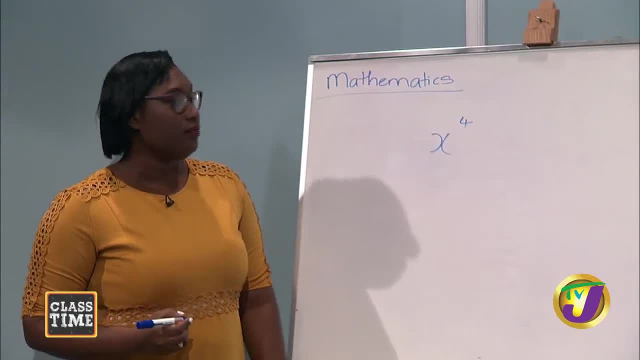 I'm going back to the board. I like when you go to the board, Oh gosh. And so you know, we want to find out the value of X to the fourth power. Now we have a value for X. 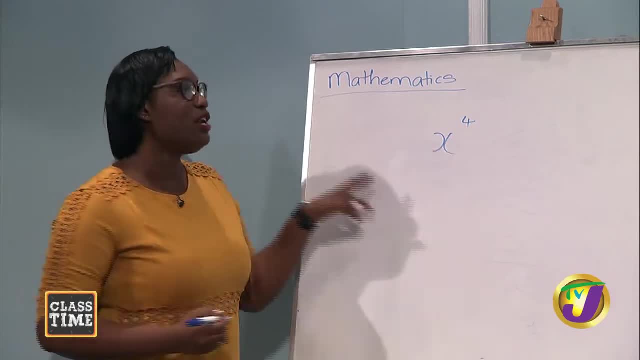 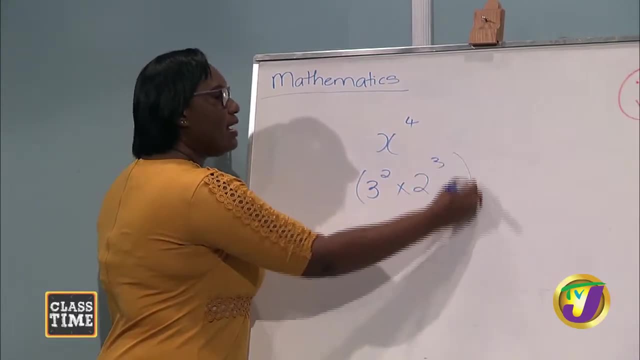 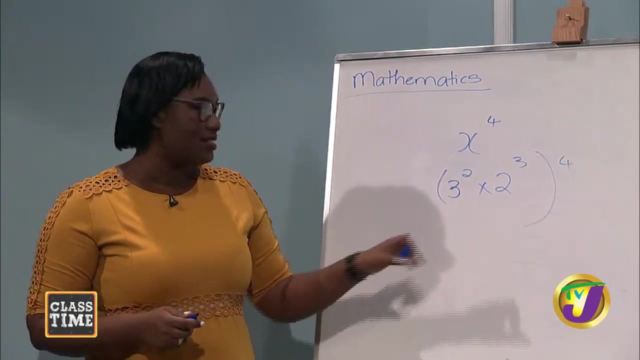 So now we know the value for X, So we have to substitute. We know that X is actually Three squared multiplied by two cubed, And this is all raised to the fourth power. Look at that, All right. Okay, So we're back to talking about laws of indices. 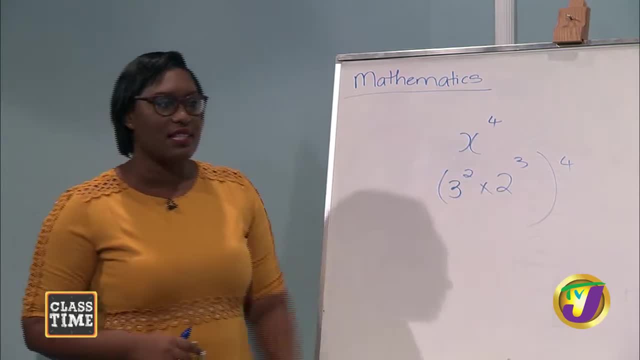 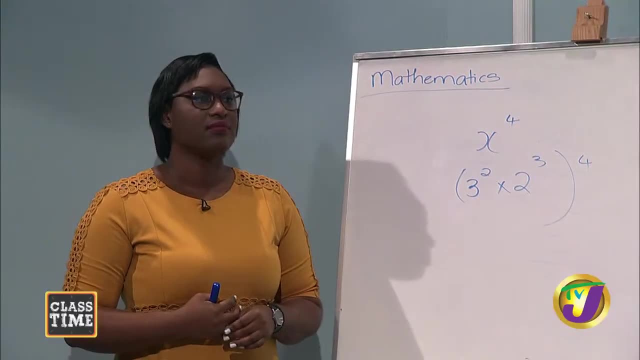 Now what happens, What we call? which one of the laws do you think we need to draw for here? Well, when a base is raised to a power and then to another power, Oh, so it's a power to power one. 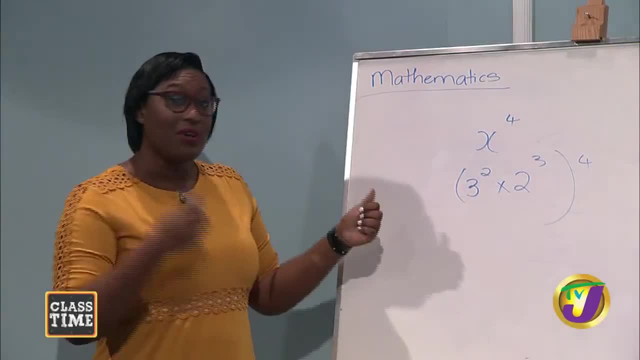 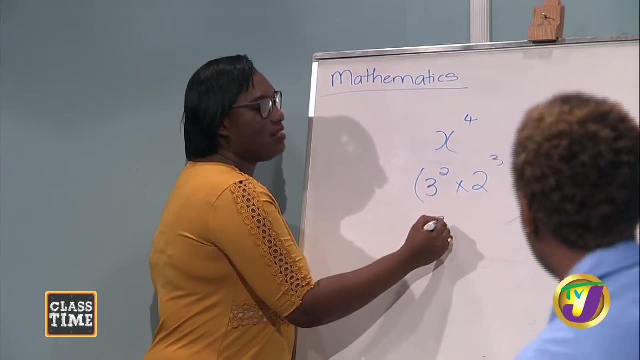 Yes, Okay, All right. So let's see What happens. So we could even further break this down to say: whoopsie, you know, three squared, Okay, Maybe my writing is not so- Three squared all to the fourth power. 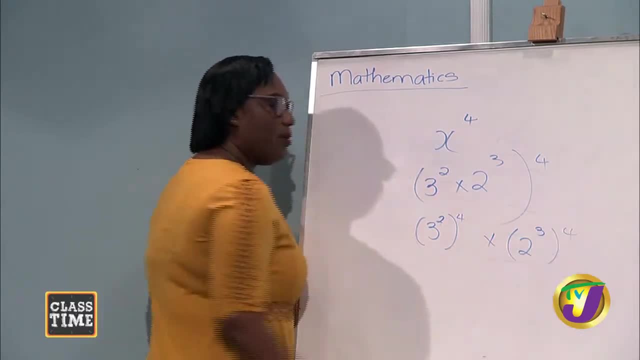 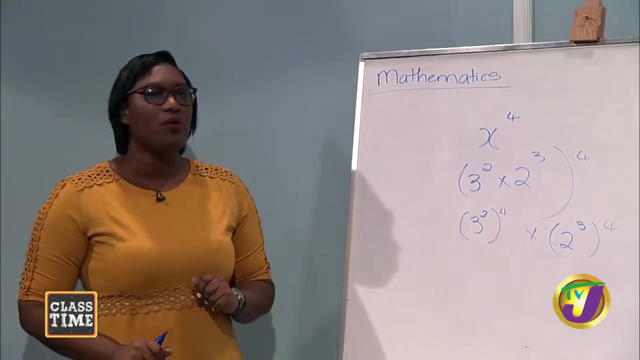 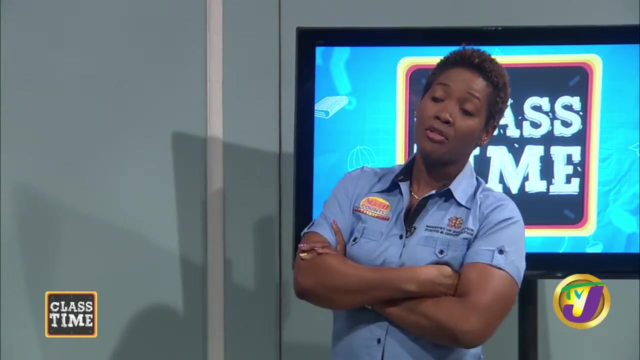 Multiply two, cubed, all to the fourth power, Right, Right. So I'm hoping that this is a lot clearer for you. So now you can see power to power. Now what happens here? All right, So basically you're saying: what is that? 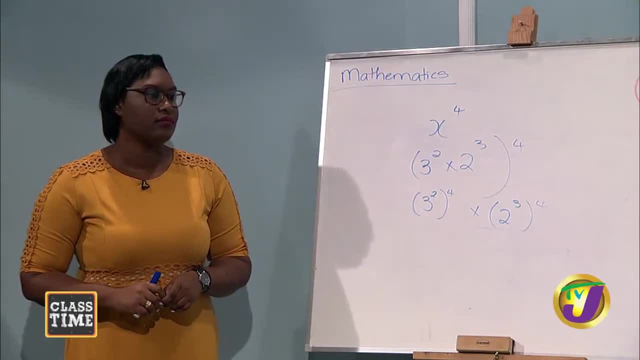 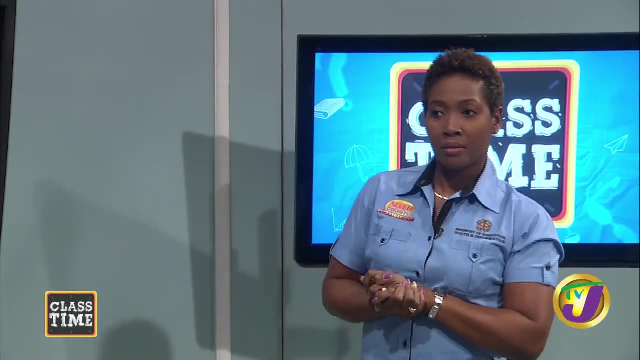 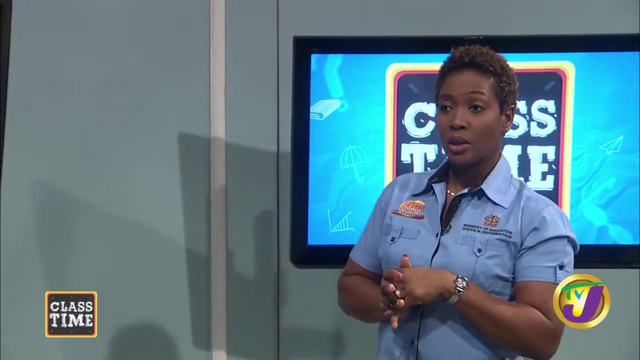 Three squared Multiply by itself four times. I could have written it all, but that takes forever, Right. So I really So I don't want to do that, because I know a shorter way. So I am going to look at three squared. 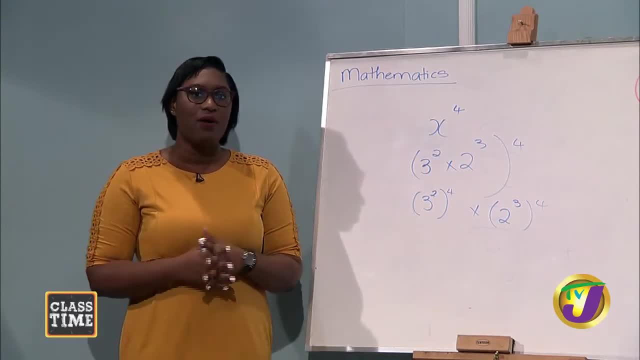 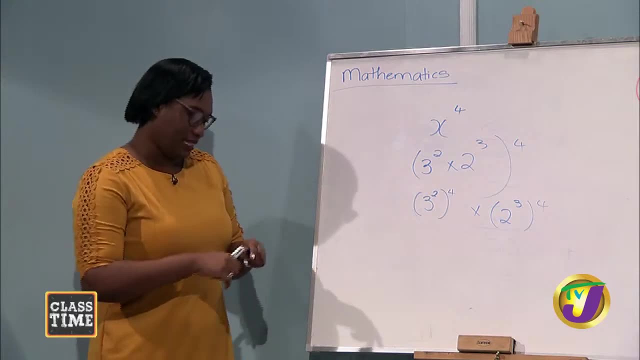 multiplied by four. Yes, So again we're going back to the power law, And we know that when we have a power raised to another power, you know we simply multiply these powers, Right? So the result here is going to be three. 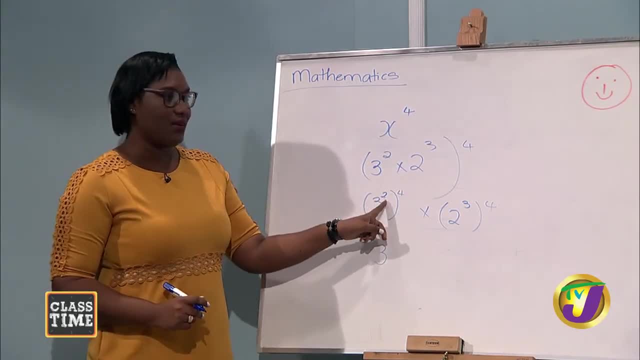 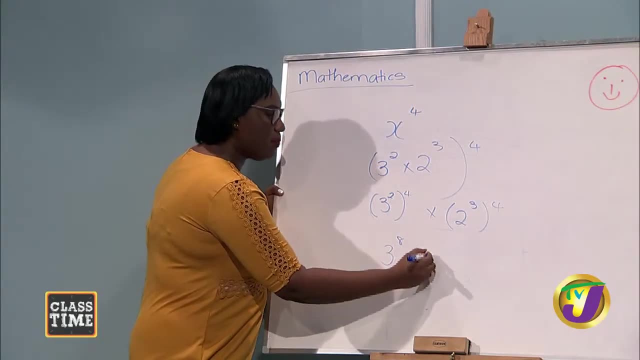 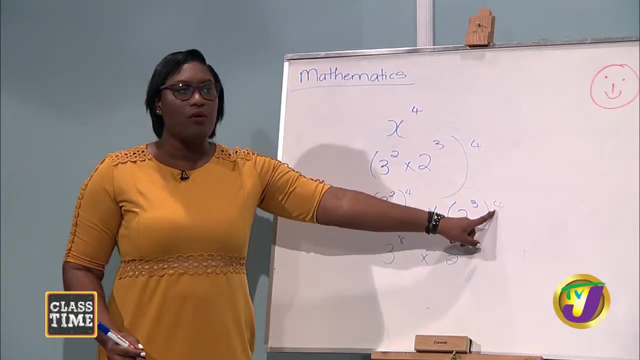 So squared, Okay, Square, human, three squared multiplied by four, So it's two times four, which will give us it eight. multiply Again, we write back our base. So we're writing back our base, which is two, And we're now multiplying our powers. 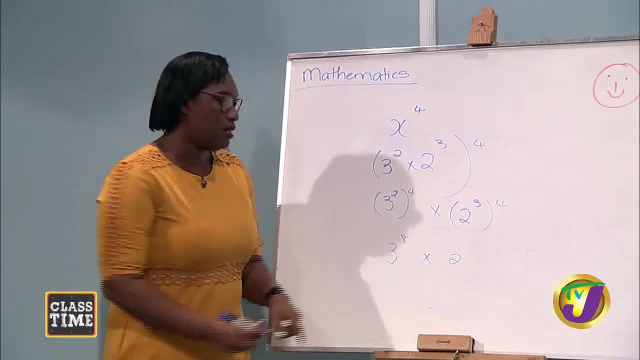 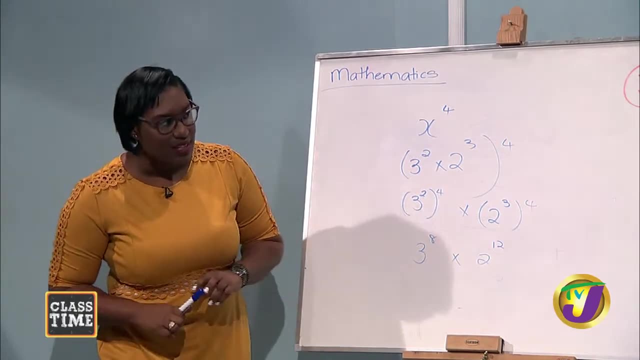 So it's going to be three multiply four, which gives us twelve. twelve So the product is Twelve. So we've done this. Let us assess our question. Let's go back to the question again. Can be a no, sir? 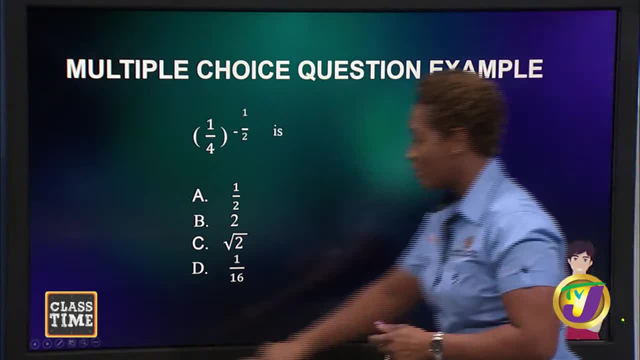 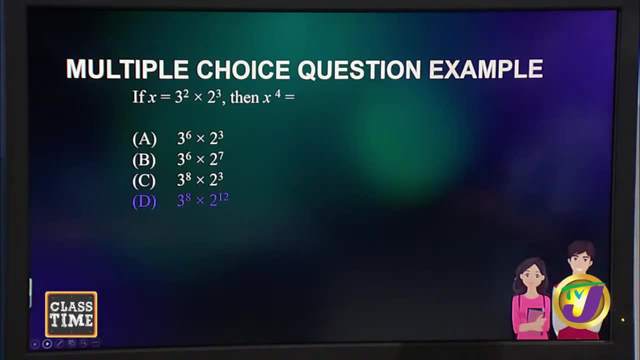 It looks like C, It does. No, it doesn't. I keep on So pressing this thing. So it's. it's actually D. So our answer is actually D, It's three. three to the eighth power, multiply two to the 12th power. 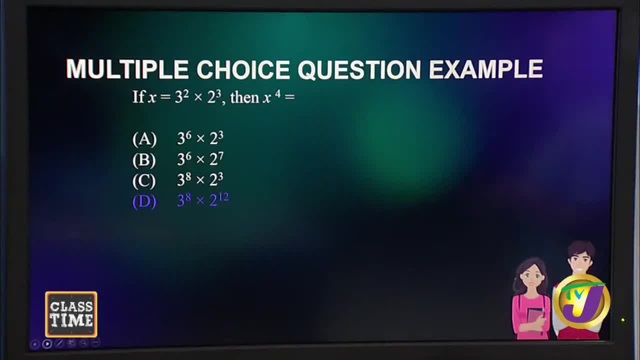 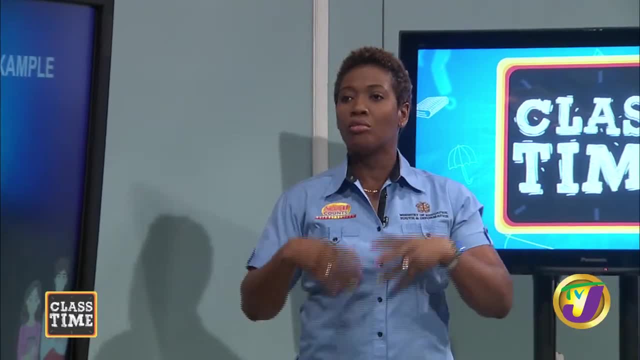 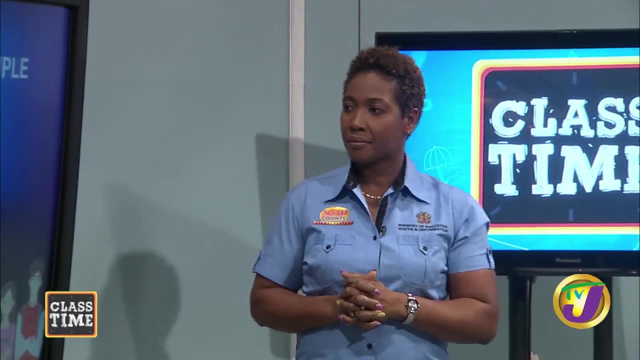 And we saw how we we did that a while ago. We use the power Of indices. So the power law states: when a base is raised to a power and raised to another power, you multiply the powers to give you the solution. Yes, OK, All right. 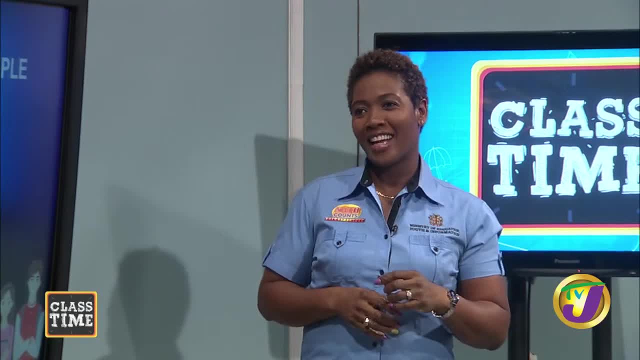 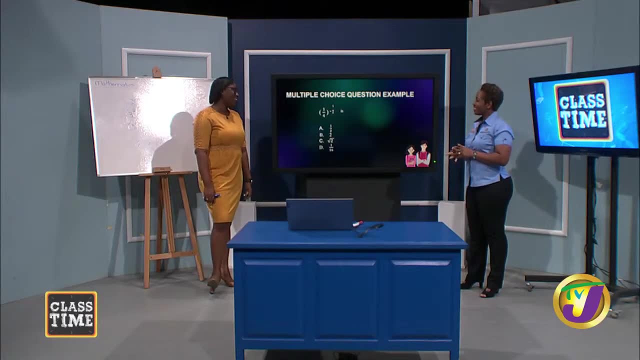 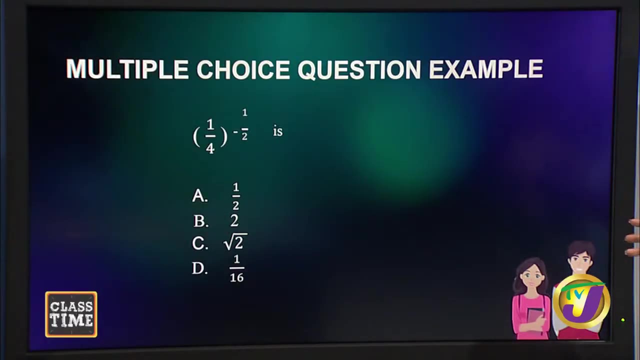 I hope they got that one. This one is a little scary again to show them. No, OK, All right. So this one looks a little bit scary. No, we know that we're dealing with indices again, But this time You're putting indices and fraction. 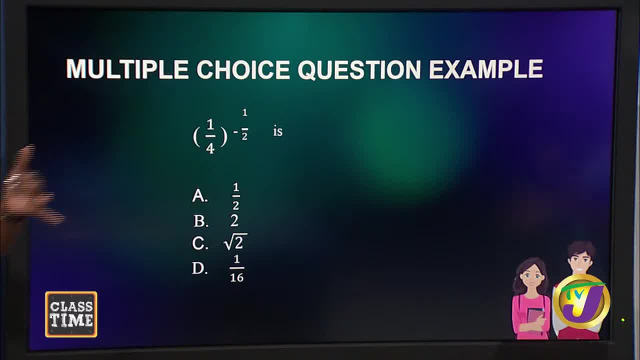 So who does this? My base is a fraction, My index is a fraction, And not only is it a fraction, it is a negative. OK, it is a negative power. So it's a negative power in my fraction, But again, relax. 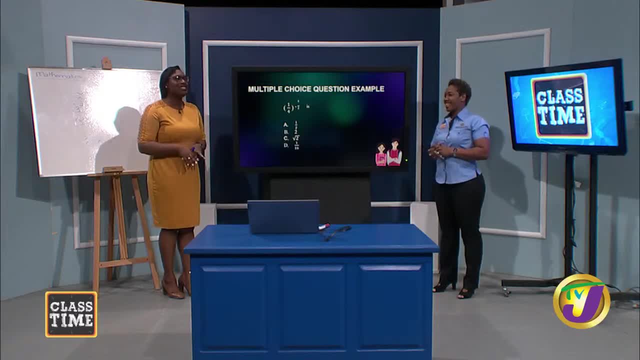 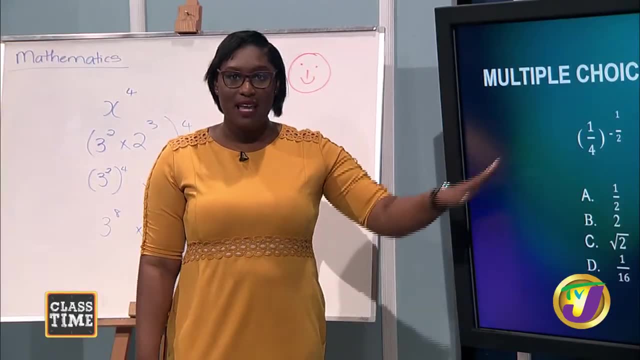 So, guys, relax, We've got this. Relax, You're going to do well though, Yeah, man. So here's what I'm going to ask for you guys: to Take a second Look at this question, Relax at home and do it. 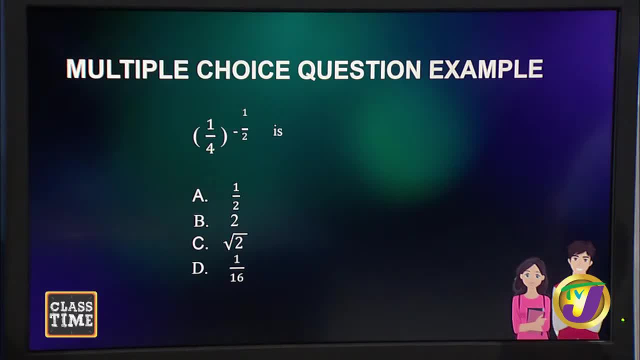 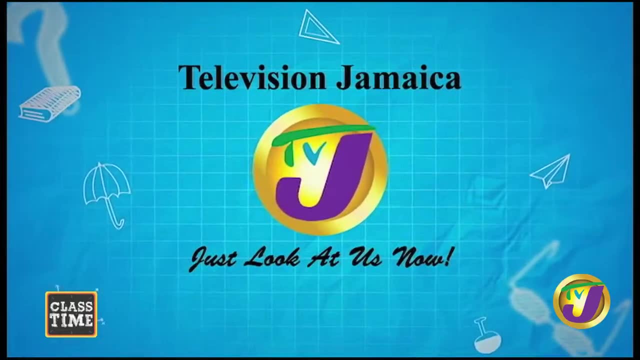 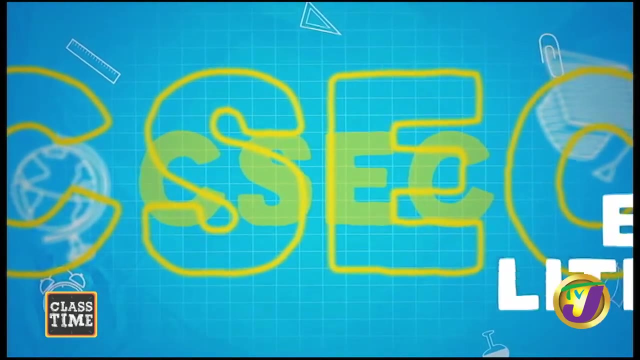 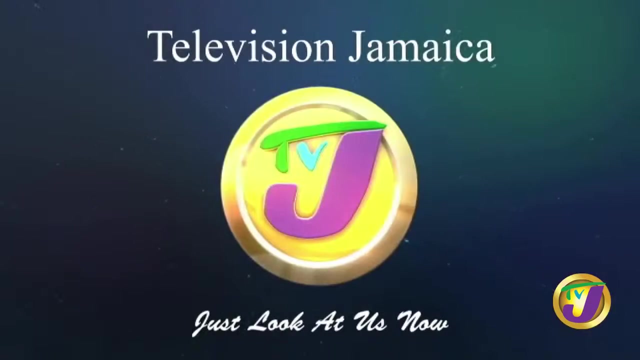 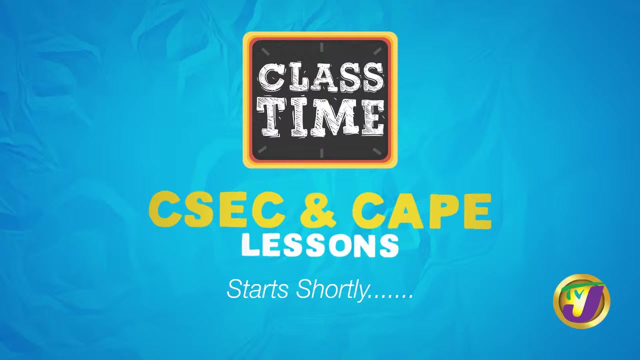 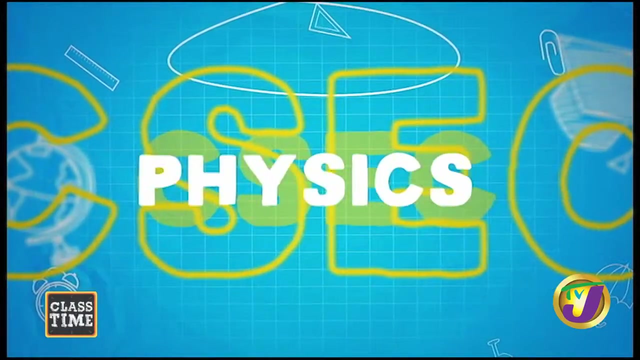 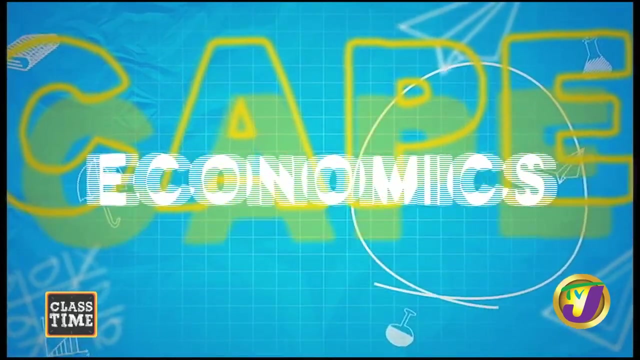 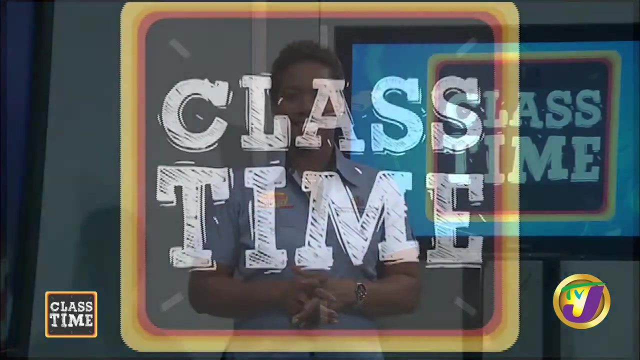 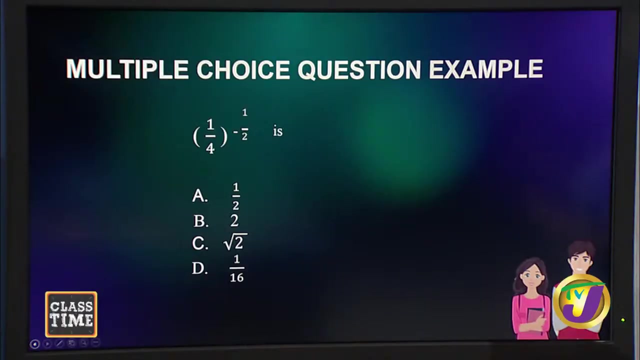 So we're going to pause here and we will wrap things up after the break, All right, So come come back guys. I know you are at home looking at this question And I know you're probably working it out. Don't take Britney. 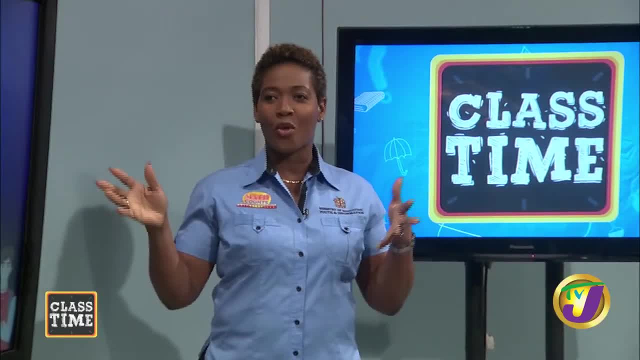 You mean, we're telling them to work it out before we come back. right, Let's just work with you so that you can check what you did at home. All right, So we're still relaxing. So this part is the check part. 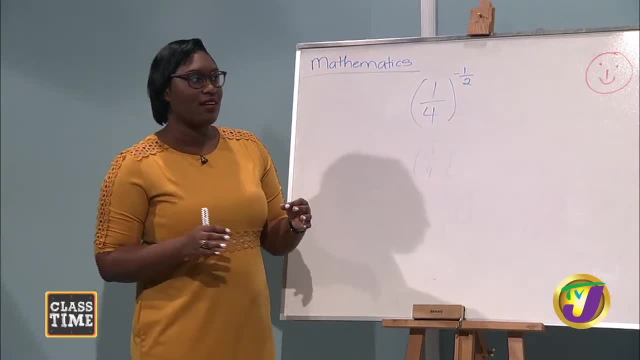 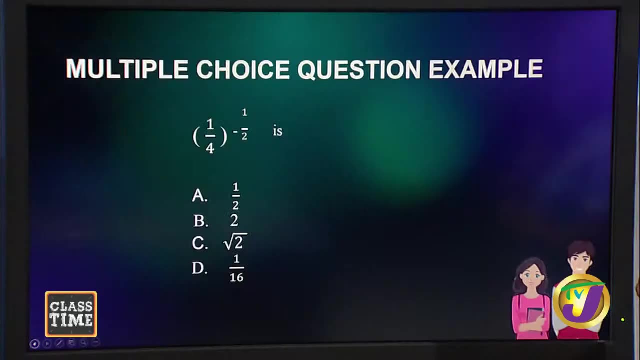 OK, Yes, All right. So what does this mean? That's all about things. So a whole lot, A lot of laws are at work here. on a negative one, We have the law, the negative law, of a negative index. We also have the law of to a fraction, a fractional power. 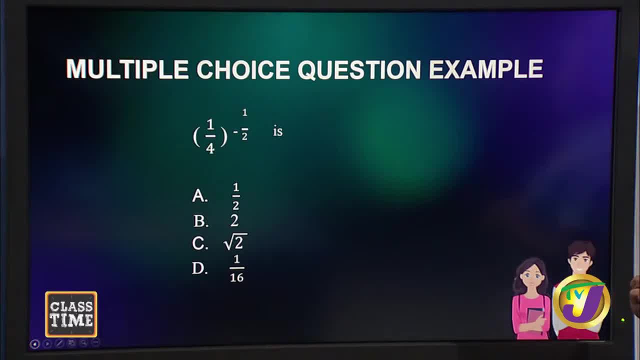 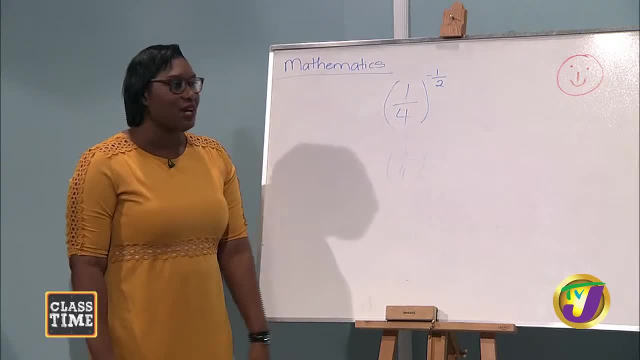 So there are several laws, So there are two laws at play here, Right? So here's what we're going to do: Break it down. Thank you, because all right. So first let's start off with the negative law. So what does that actually mean? 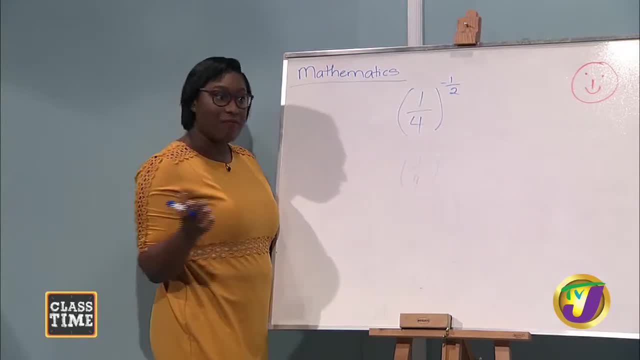 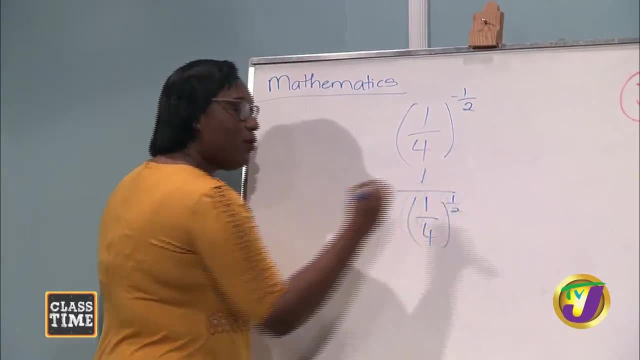 So I can now rewrite a quarter raised to the negative half power, as one divide one quarter, all raised to the half power. OK, so you got rid of that negative. Yes, So the negative. Well, it's not really gotten rid of. 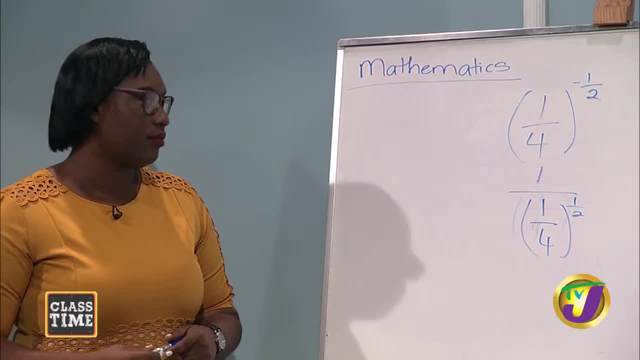 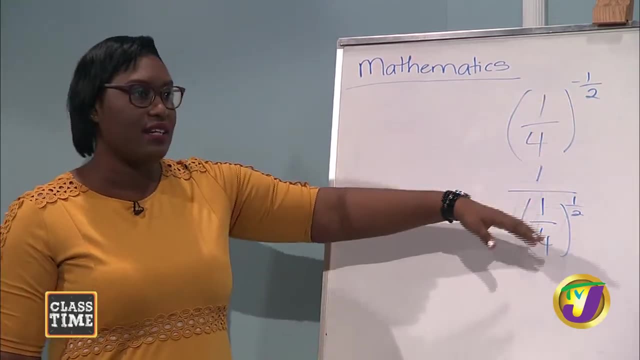 No, you're rewritten the power without the negative Yes As a positive Yes, because the law of indices states that when I have a negative power, I'm actually dividing one by the denominator Yes, Right, Right, All right. So here I've done something. 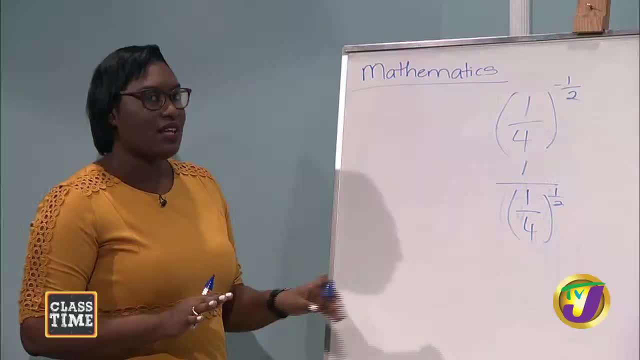 Or, to make it positive, you put it in the denominator's place. Yes, Got you All right. Guys, are you a little bit scared? OK, let's rewrite it. Let's rewrite it in a form that is more user friendly. 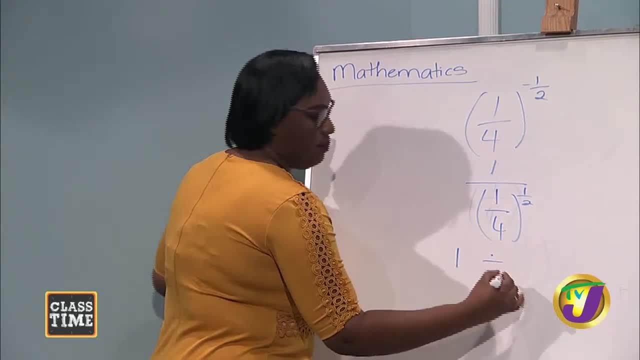 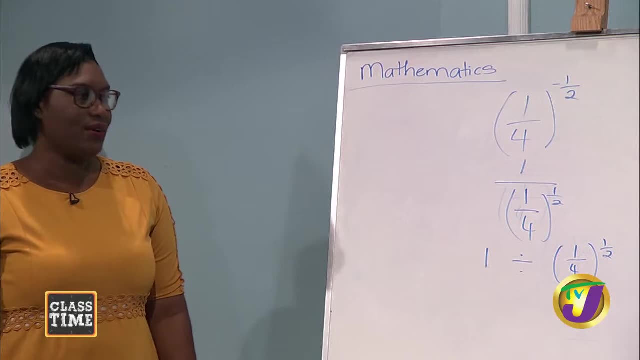 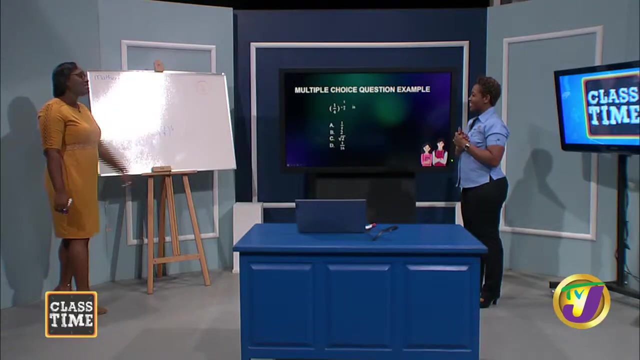 How about that? So it's one divide by a quarter, raised to the half power. There you go Right, OK, we got this. No, but go on, OK, All right. So let's deal with one divide by a quarter. 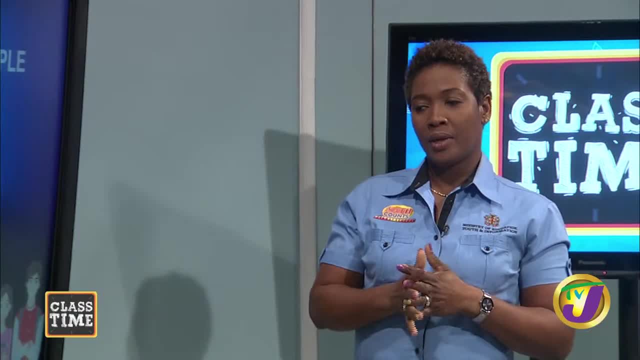 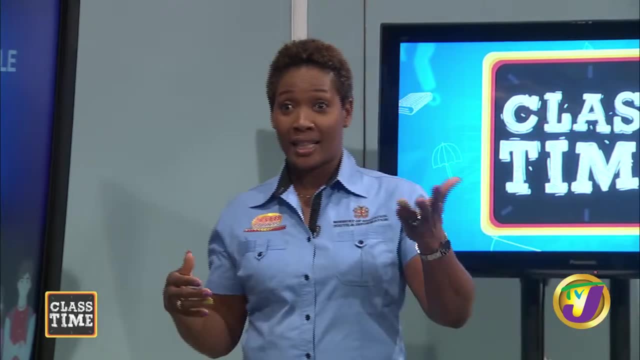 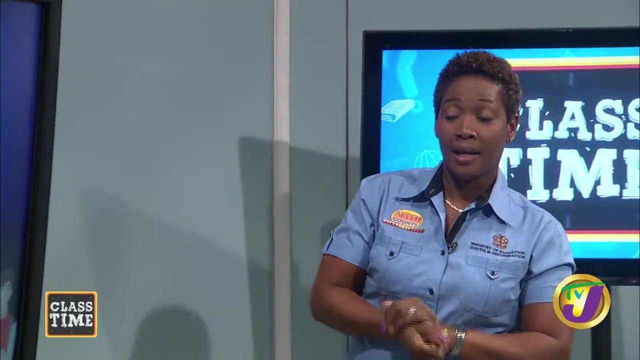 Yes, All right, So you think we can do that. We don't have to go to the powers? Yeah, we have to go to that powers first, because you did tell them the law of indices and we do the exponent first. Yes, So let us do that raise. 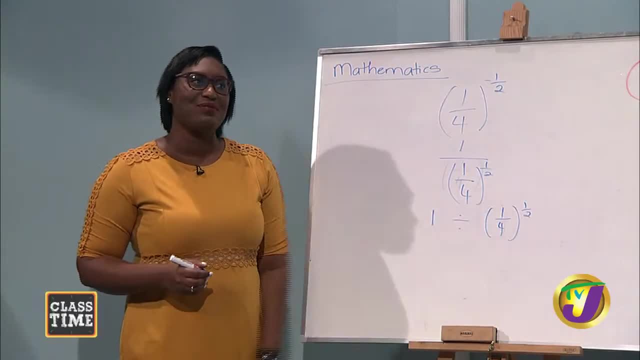 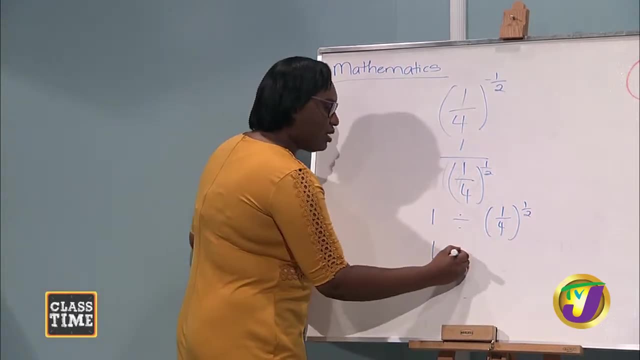 Let's find the square root of that. All right, So we know that when something is raised to the half power, it's the same as finding the square root of that number. So it's actually one, And we're going to find the square root of this, which will give me 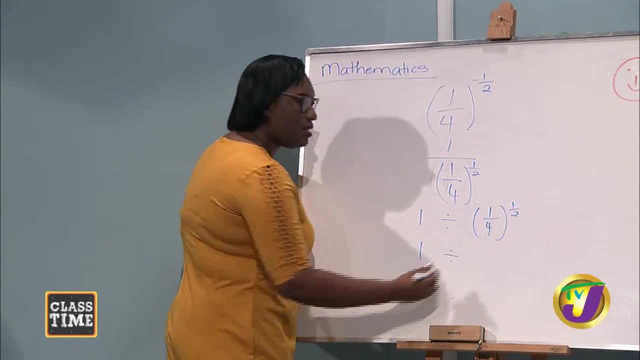 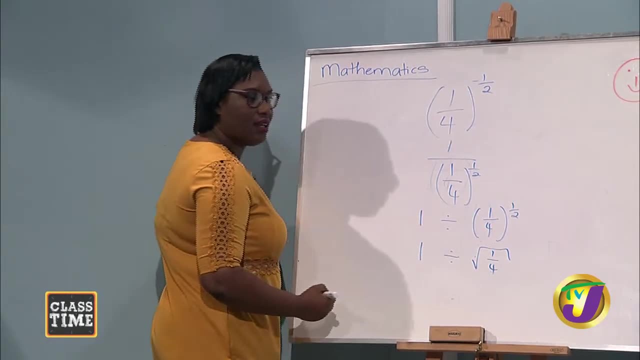 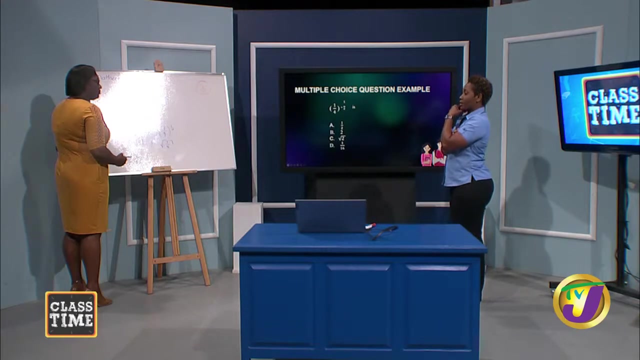 Couldn't just put that outside. What, What, OK, So the one it's actually going to be the square root, OK, Or let's, if we were to do, to do, to do, Mm. hmm, Take that off, OK, please. 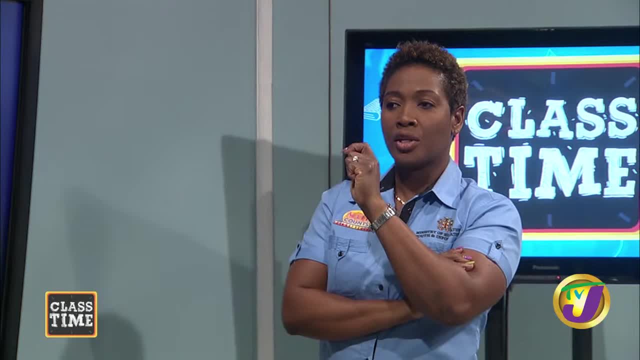 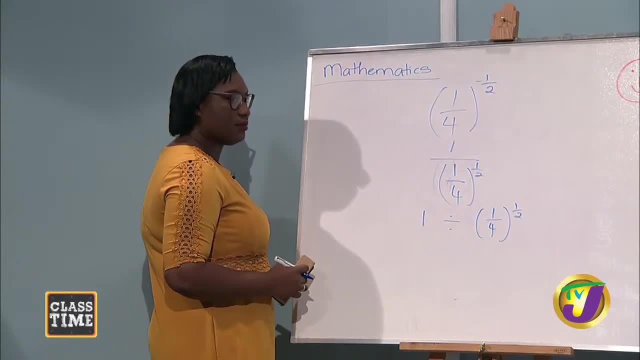 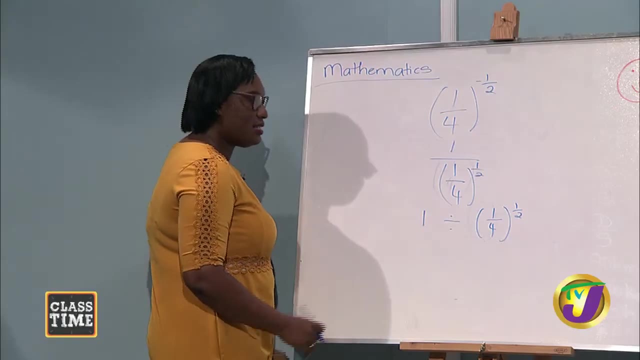 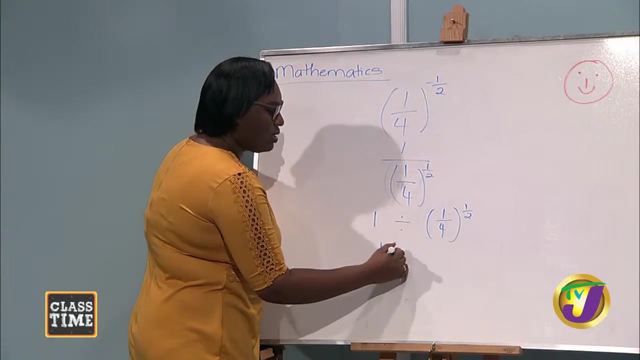 We just removed that. We just rewrote the thing in terms of a positive index. All right, All right. So this is the same as saying So one divide by a quarter. a quarter is the same as saying one divide by four. 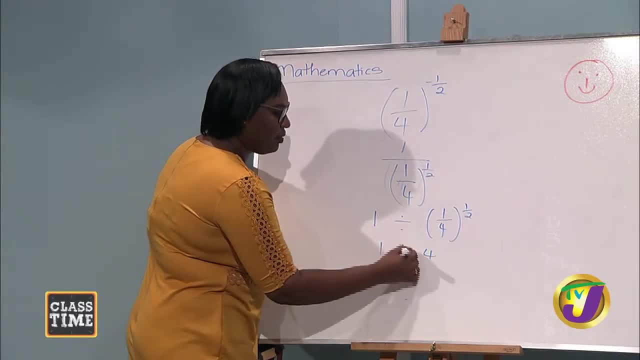 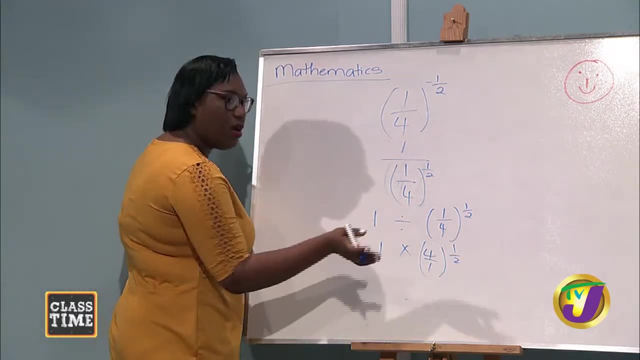 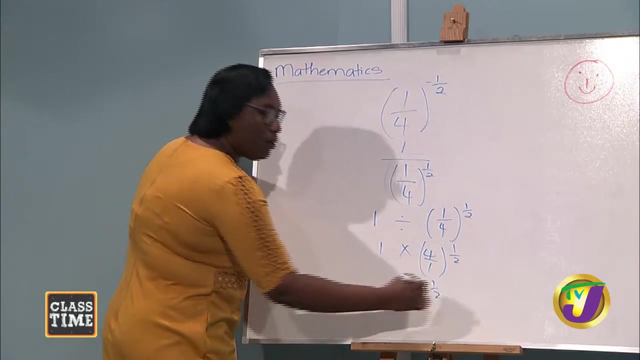 one multiplied by four, sorry, one multiplied by four over one, raised to half, Right, Which is the same as saying one multiplied by anything. I'm going to get back that result. So that is going to To be four to the half power, Right. 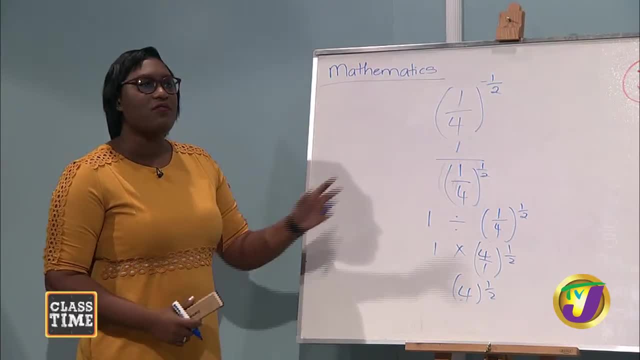 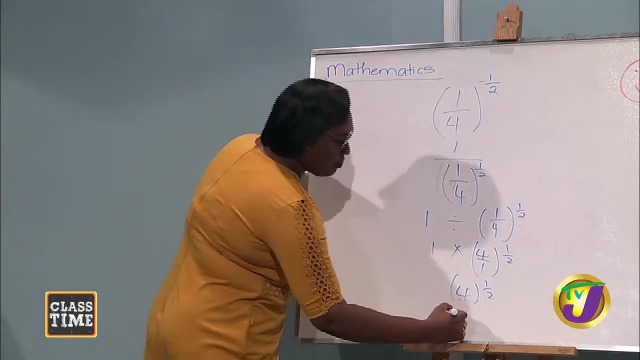 So any, any number raised to a fractional power And in this case, because the fractional power is a half, we're not going to find the square root of this number, So we're going to find the square root of four, which is: the square root of four is: 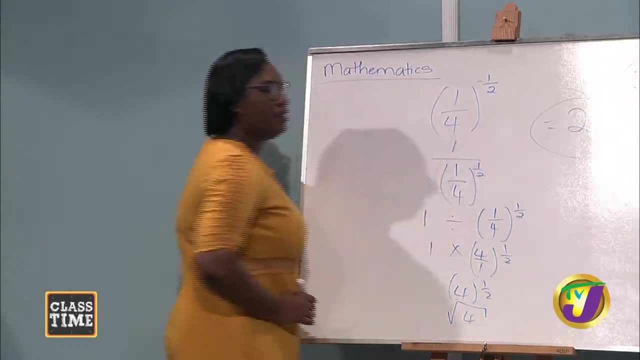 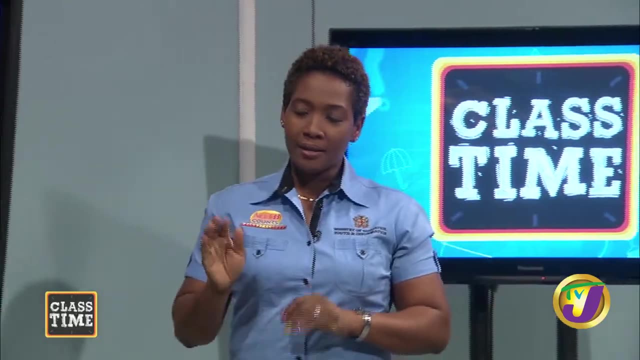 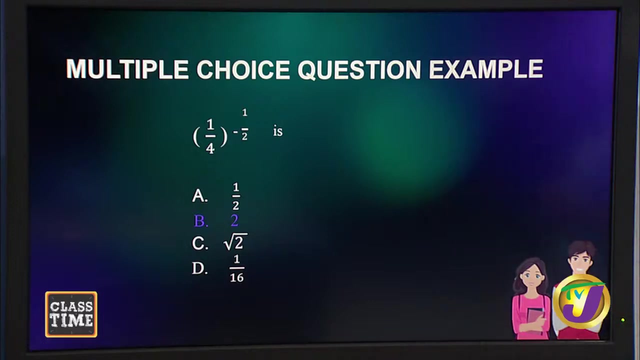 two, all the way up here. two: All right, We're right, I'm wrong. teacher Boy, It's a little stickler. Let's see what Jenny says. All right, Jenny says I am right. Jenny says that I am good. 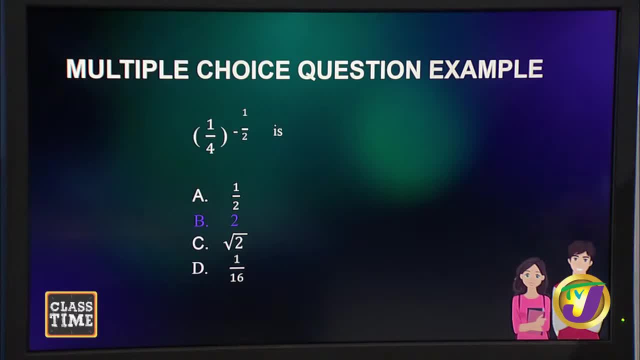 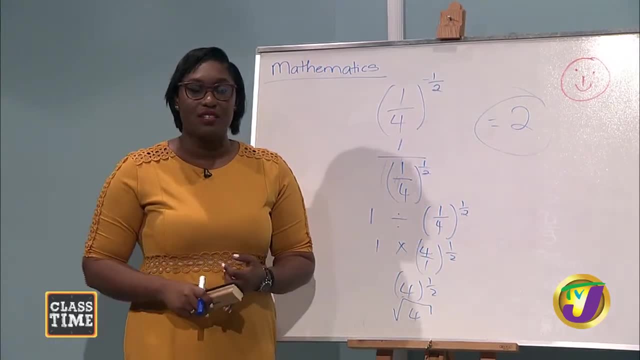 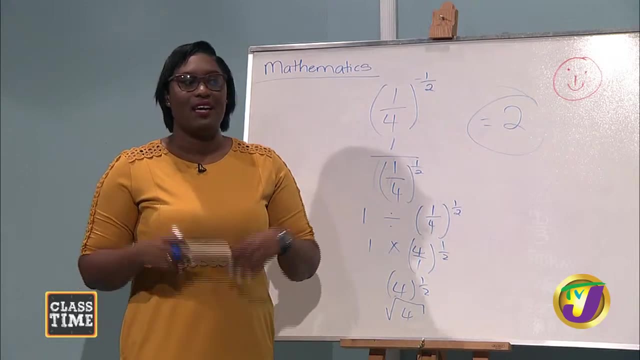 Jenny says that too. it is right. I know this one may kind of throw a loop again, because we're not only dealing with negative power but we're also dealing with fractional power And, as you can see here, mistake can make. So please and please and please, please, check and always relax. 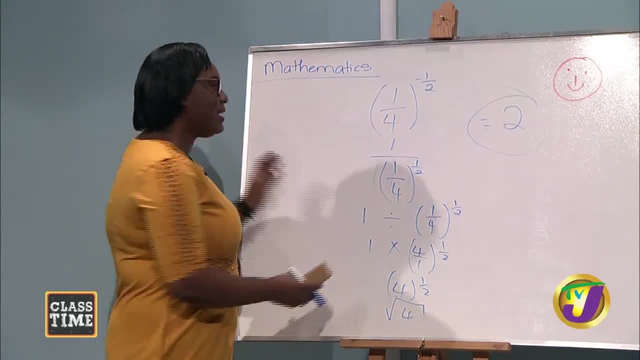 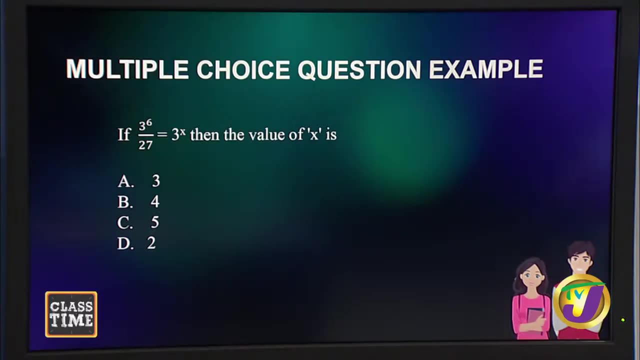 Right. So let's go to another one. Exciting time still. So we're still excited. So if three to the six power, divided by twenty seven, equals three to the X power, then the value of X is all right. All right, So now we have an index equation. 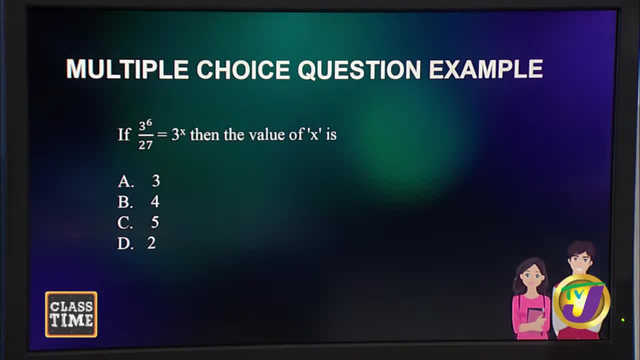 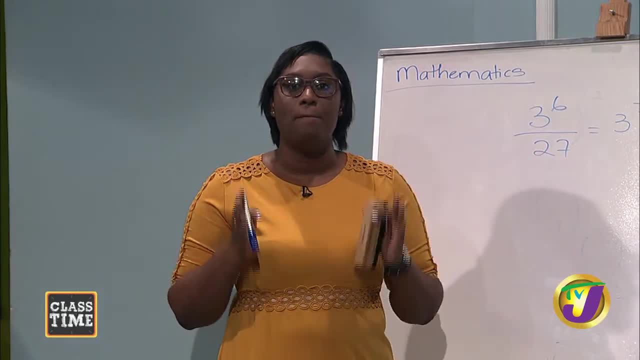 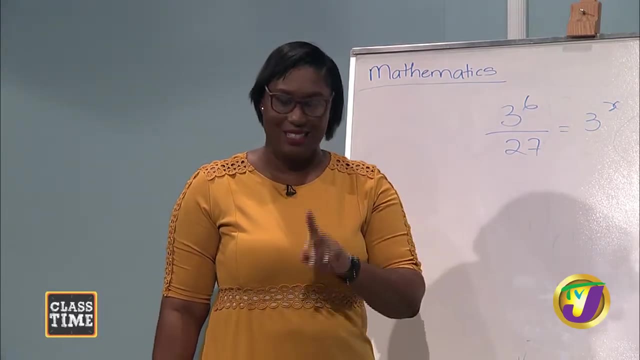 Right, And one of the things that we know about indices is that we always have to have. if we're doing any sort of equation, we have to have everything written to the same base. So it's very important, if possible. So let us go ahead and assess our equation. 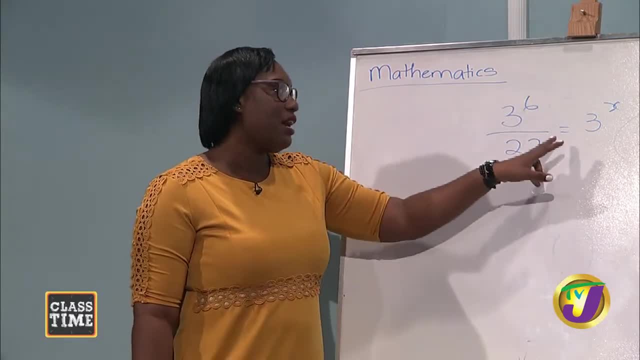 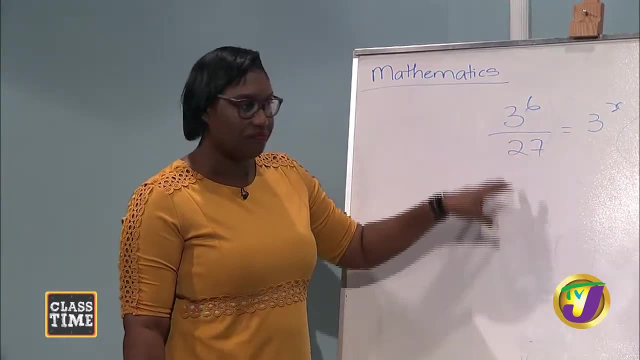 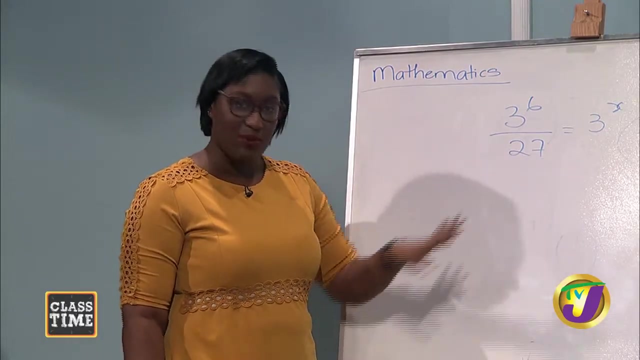 So now we have three to the six power divide. twenty seven is equal to three to something power. So so now we know that we can convert twenty seven, Right, Because three is a factor of twenty seven. Yes, So we can convert twenty seven to something. 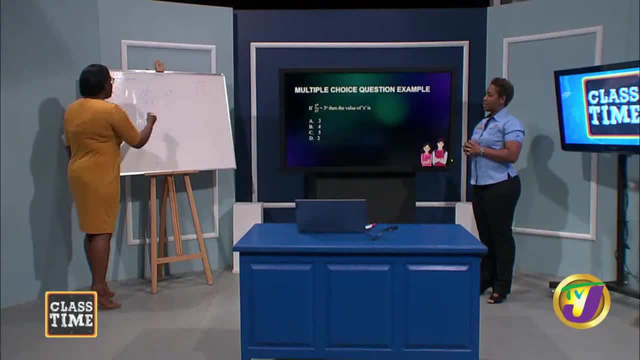 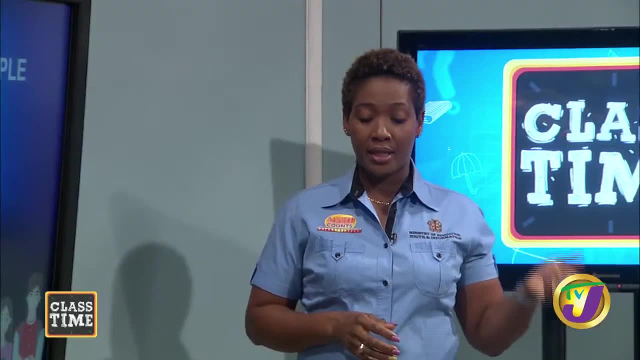 To represent. to represent three to the power of something, So it's going to be three to the six power divide. OK, twenty seven, You have three times three is nine times nine is twenty seven. So that makes three to the third power is equal to three to the X. 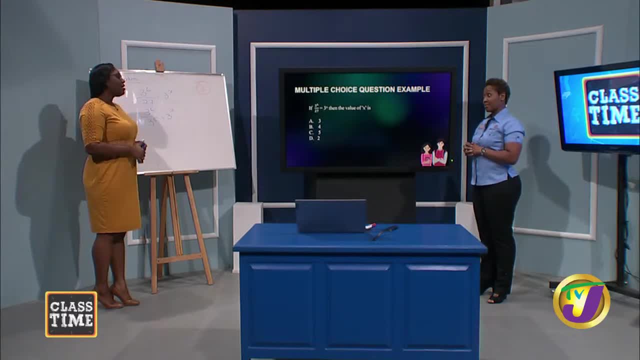 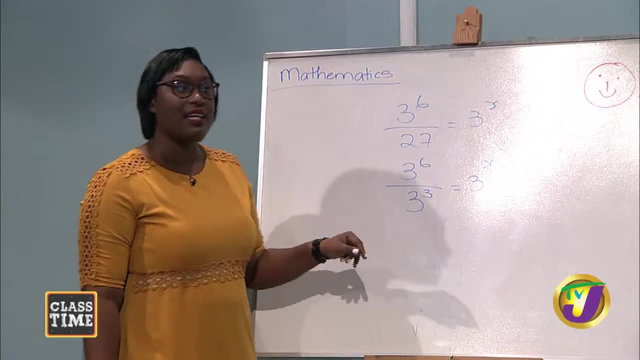 No, you're applying another law. Laws come back in and we excited again looking at the law of law of indices and specifically, we're looking at what happens when we divide two indexes. So here it is that we're dividing two indexes, right? 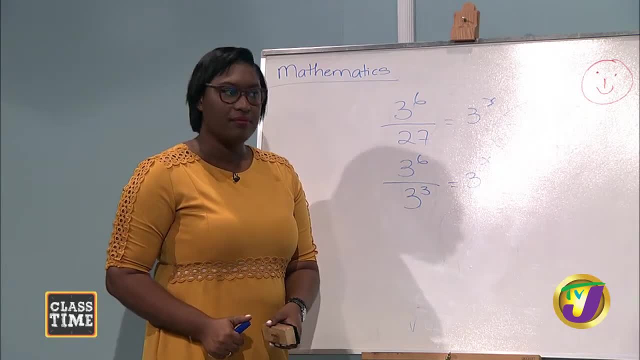 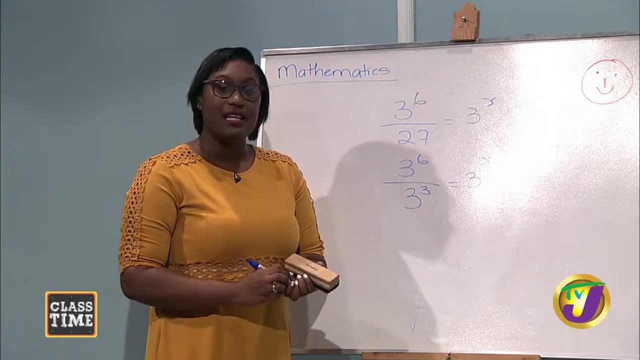 Well, the two numbers that has the same base raise the powers. OK, Yes, So what happens with the index? We simply subtract our index, right? So the last thing that we know, subtract our index. So it's going to be- I can rewrite it several ways- right guys? 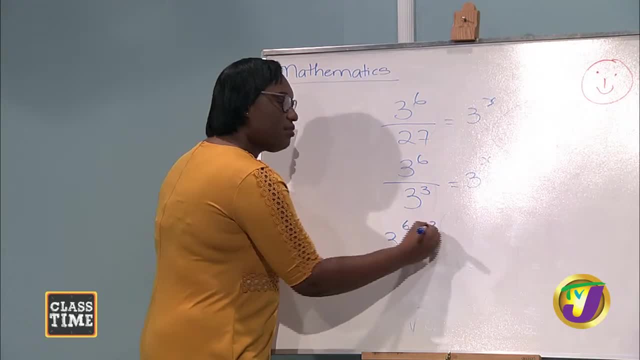 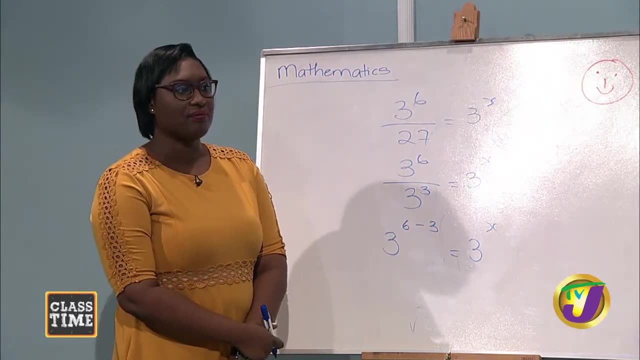 So I can rewrite it as three to the six power Subtract three is equal to three X. Now, just to remind them, we're not guessing this thing. If we were to write out three, raise to the six, power expanded form and then write: 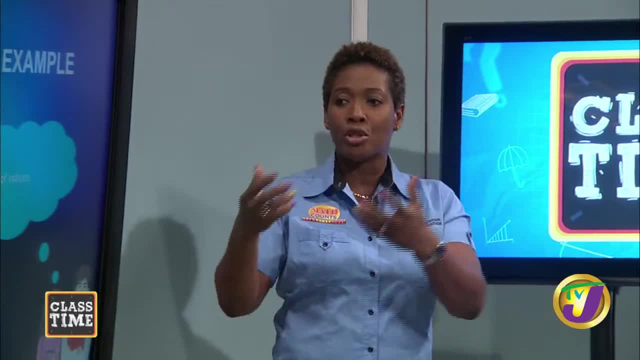 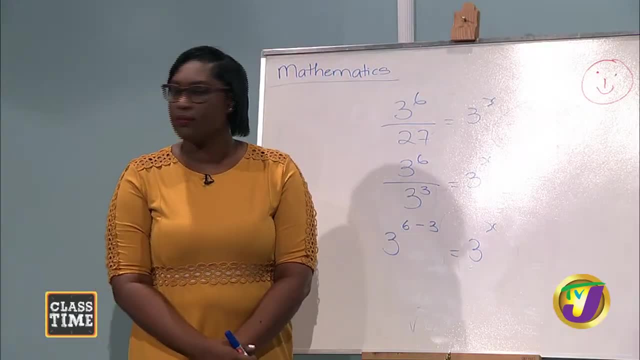 out three raise to the third power expanded form, you'd have realized that the result would have given you the very same thing as three raise to the six power subtract three. So it is just that this is the shorter, the shorter way to do this. 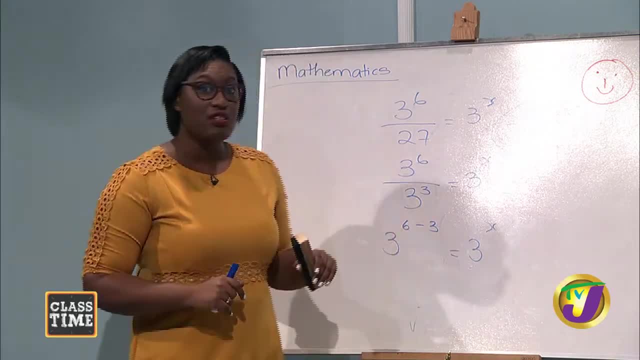 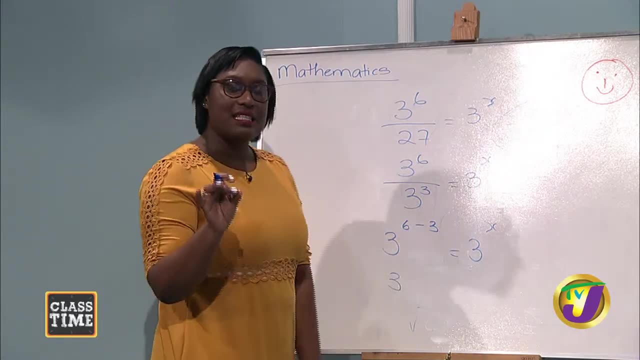 All right, So this is the shorter way of doing it. Yes, that is true. So my result here is going to be: I'm just simply subtracting my indexes, And so it's going to be three. six Subtract three is three.